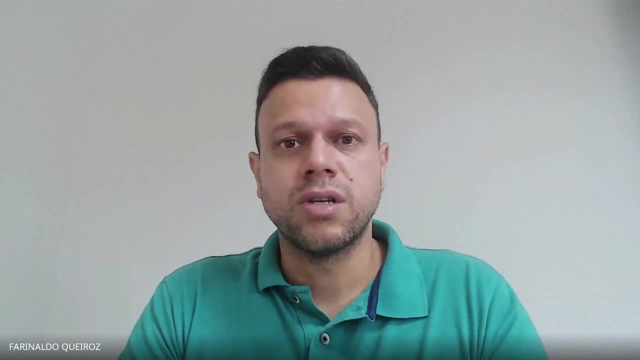 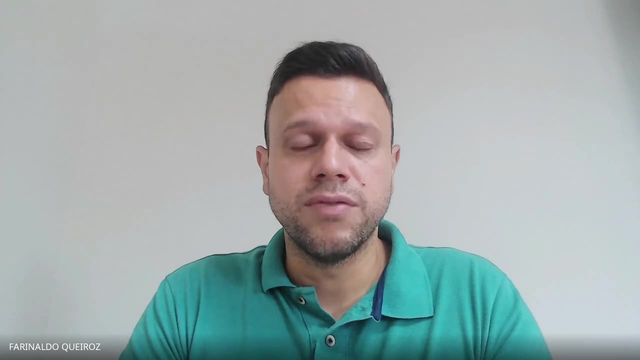 first time, that's a series of lectures concerning dark matter for advanced students, which is being organized by the International Institute of Physics and the physics department here in Natal, Brazil. So welcome, and let's start with the eighth lecture. In the previous lecture, we discussed: 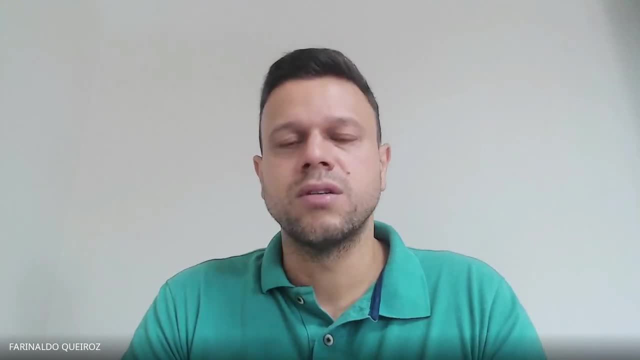 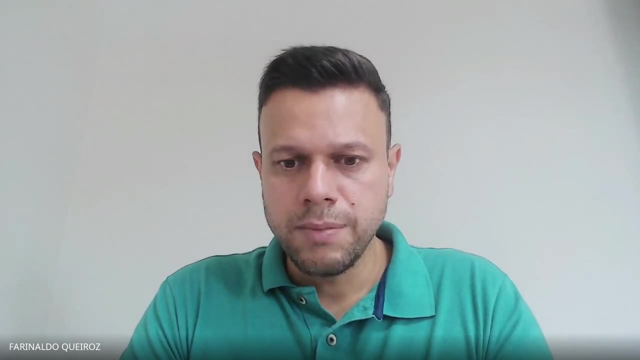 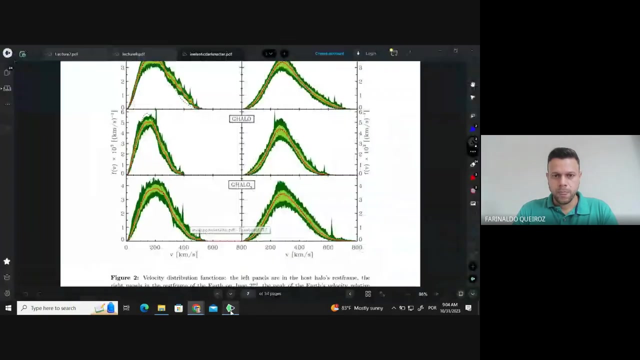 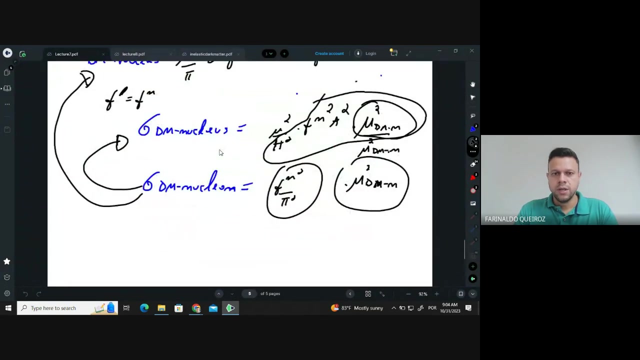 direct detection. and now we're gonna finish discussing direct detection, then move on to indirect dark matter detection. So let me share my slides. So we were here in the last lecture, So just to recap, what we've seen was that we did the, we deduced. 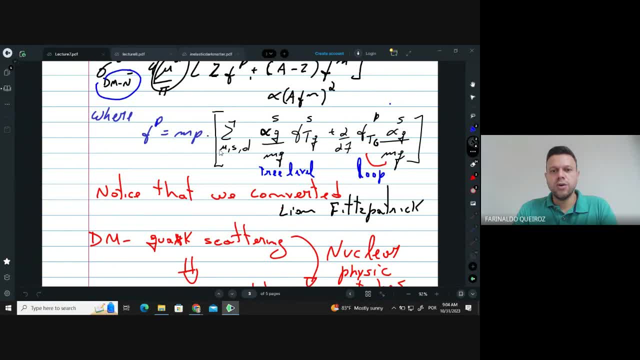 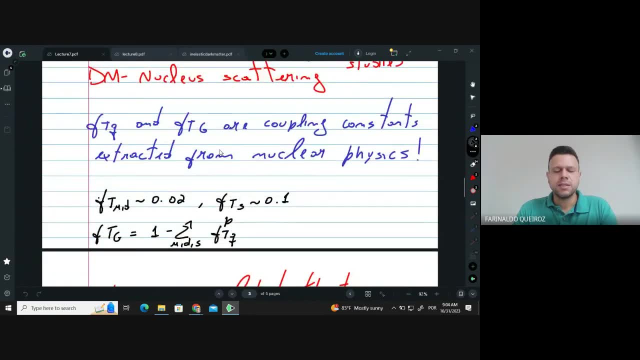 the dark matter nucleus scattering and showed that how you can connect the dark matter nucleus scattering to the dark matter nucleon scattering. It's simply, it's just by a simple relation with the reduced mass, one for the nucleus, one for the nucleon or proton or neutron. and you have to as 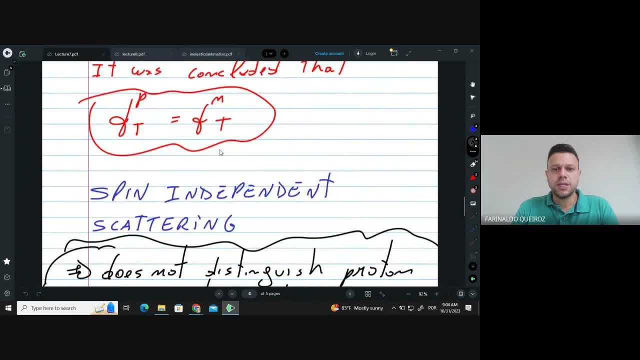 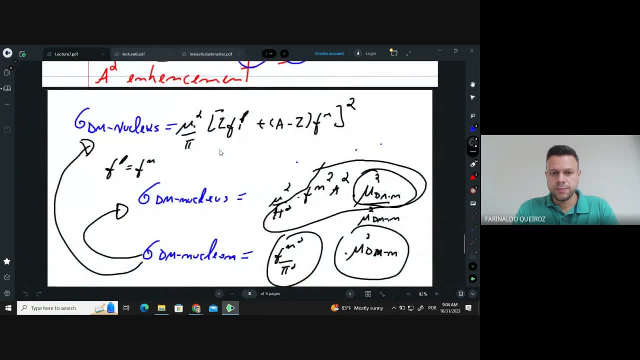 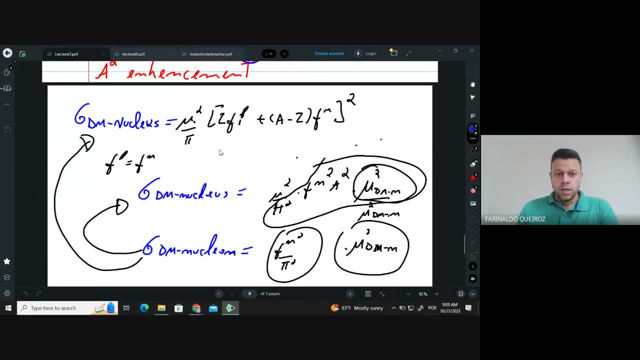 collaborations, experimental collaborations, do they assume that the coupling with protons and neutrons are the same. Once you do that, so let me just go back here, so you have this formula right there. so the dark matter nucleus scattering depends on the how dark matter couples to protons and how dark matter couples to 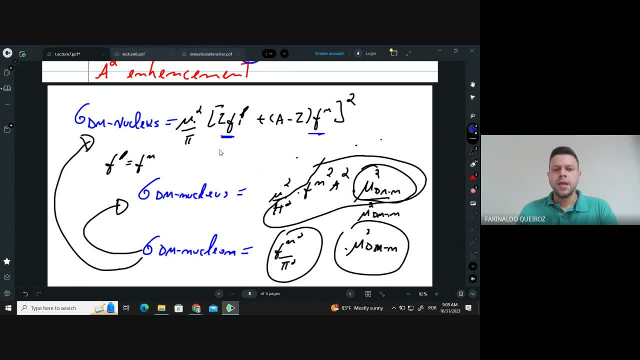 neutrons for spin independent scattering, and this reduced mass is reduced mass between the dark matter and the nucleus. so mu here is the product of the dark matter coupling. So this is the dark matter. chi mass times the mass of the nucleus divided by the sum of those masses. This mu here is the dark. 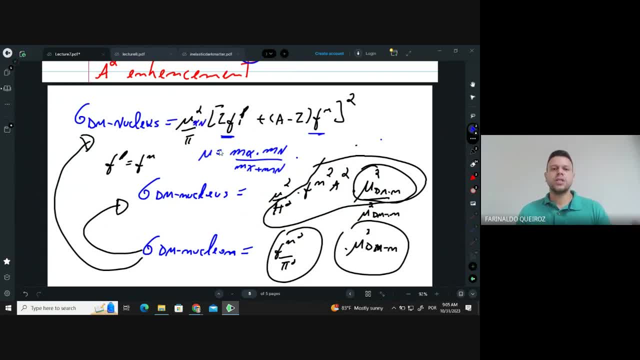 matter chi nucleus, and it wants to. what the experiments report is not the constraint on the dark matter nucleus scattering, but rather the constraint on the dark matter nucleon scattering. So what they do? they assume that fp is equal fn. so dark matter couples to protons and neutrons are the same. 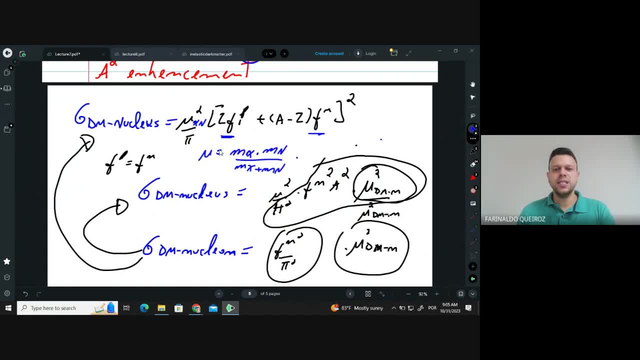 way in this case, then the z dependence goes away and you have just a fn squared, a squared dependence on the that governs the dark matter, nucleon nucleus scattering. and when from this one you convert to a dark matter, let me erase here to a dark matter nucleon scattering cross-section by 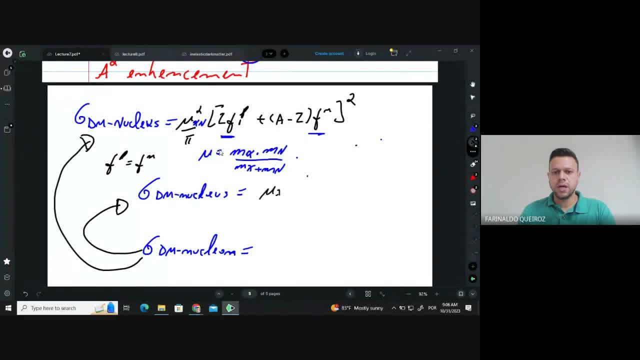 simply you have this one, so you get mu chi n over pi squared, and then you'll get an fn squared, a squared. so that's what you get for dark matter- nucleus scattering cross-section, and then for a nucleon is simply mu chi n, nucleon, pi fn squared, and then you integrate out the a squared dependence. so 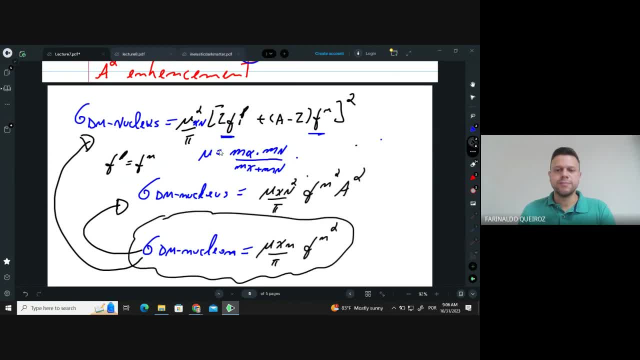 that's what the dark matter- nucleon scattering cross-section looks like. So this thing is just particle physics, as you can see. so it's just how dark matter couples to up and down quarks, and then eventually you translate that to dark matter nucleon scattering. 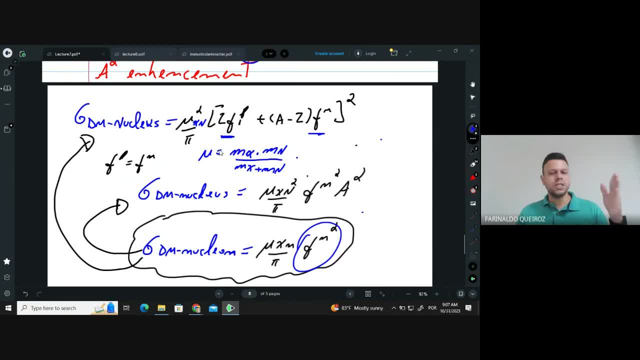 okay, so there are two conversions that need to take place. one is from quarks to nucleons, from nucleons to nucleus. okay, but luckily our nuclear physicist friends have done this for us, and the only thing we need to do is to plug in the numbers one by one. 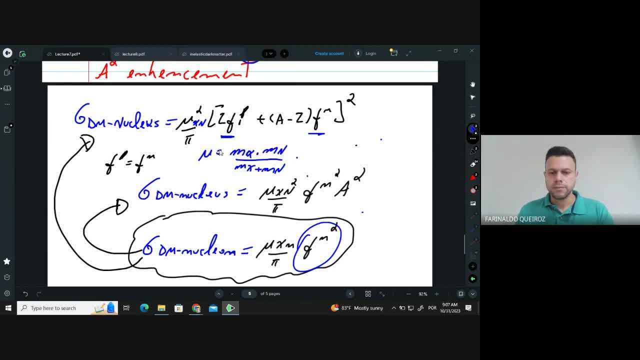 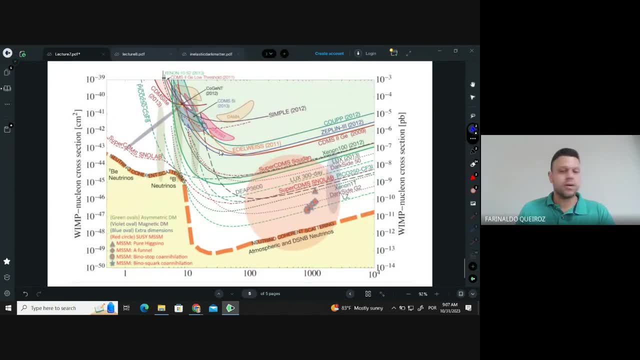 So we plug in the numbers once we know our model. Okay, and now I want to show this one, this figure, which is the common figure, where you're going to see at conferences where direct detection experiments they report there are new results- no results so far. and this figure. I'm going to try to explain some key things, so you've learned already. 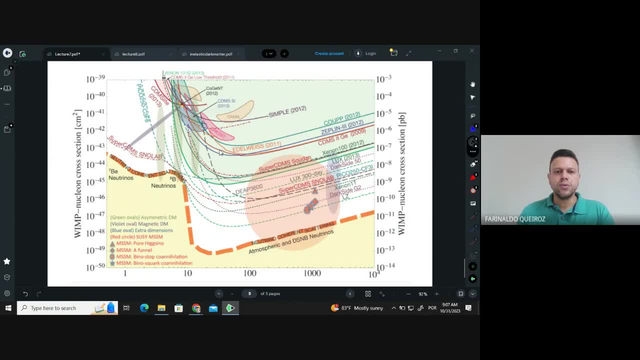 from last lecture That the. that the the reason why those curves have this shape. so they go up, they rise up for low dark matter masses and then they have a deep, a dip, and then rises again linearly with the mass, with one over mass. okay, so this has to do with the energy threshold, this has to do with the kinetic. 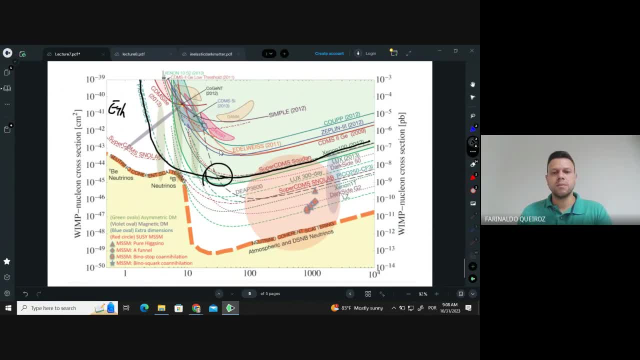 arguments: okay, reduced mass of dark matter between the dark matter particle and the nucleus. and this has to do with the one over m chi behavior, which is related to the number density- remember, rho is n n times m, but the scattering rate depends on the number density. therefore, 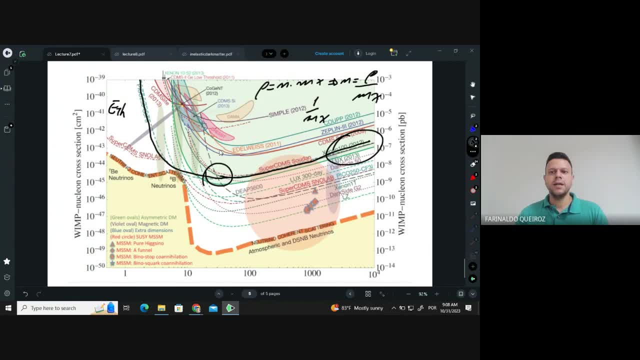 the number density is rho over m chi. so as i increase the dark matter mass, the number n chi decreases linearly, one over x m chi. then the scattering rate decreases. and as the the scattering rate decreases, my constraining power discreetly weakens at the same rate. 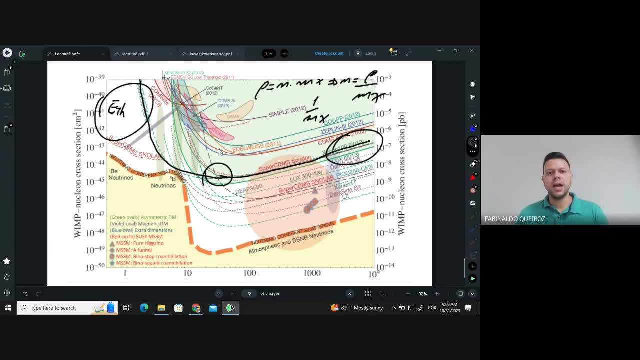 So I have three features: threshold, kinematic arguments and kinematics and the number density. So one has to do with astro, One has to do with just relativity. I would say Kinematics, Kinematics, Kinematics. 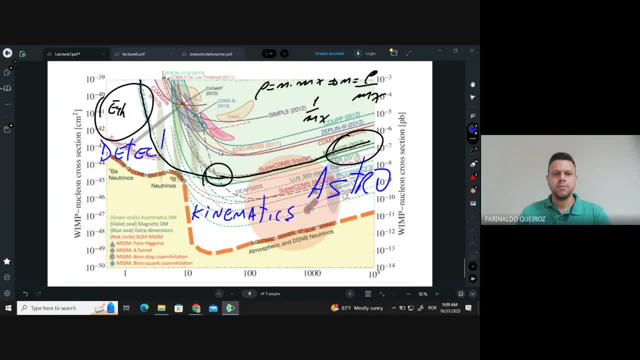 And this has to do with detector. And then you see that all the direct detection experiments have the same feature. Their limits have the same feature for all of them. They have different ways, different limits, obviously, But they have the same shape. 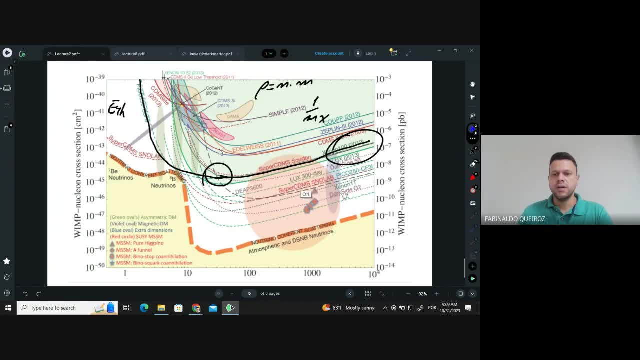 And the reason for this, as I'm going to cover now, is for this reason, Hold on. So, as you know, the rate dr de is proportional to the scattering rate and also goes one over the mass dark matter mass. 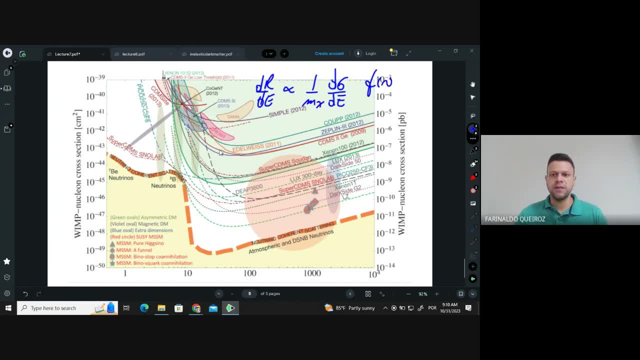 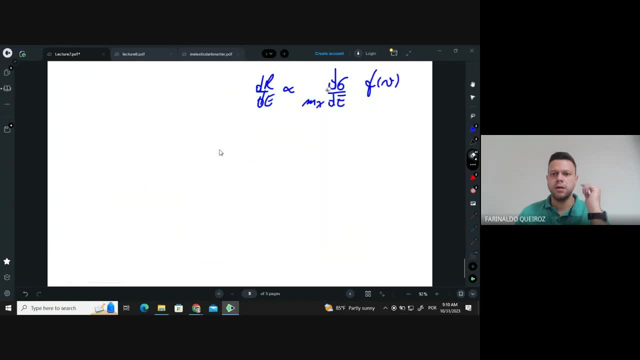 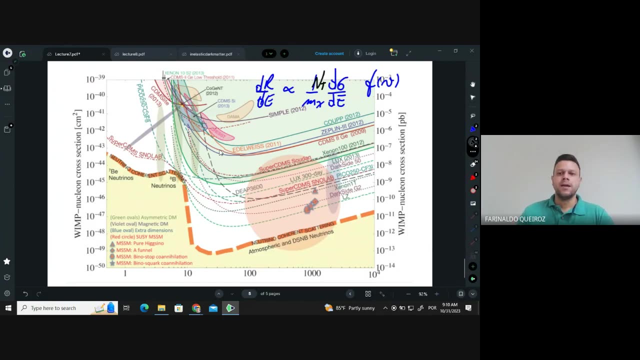 And also you have some form factors in the velocity distribution act of v. OK, But we also had a number here in the numerator which was the number- Oh no, Sorry- And the number of targets And the number of targets. 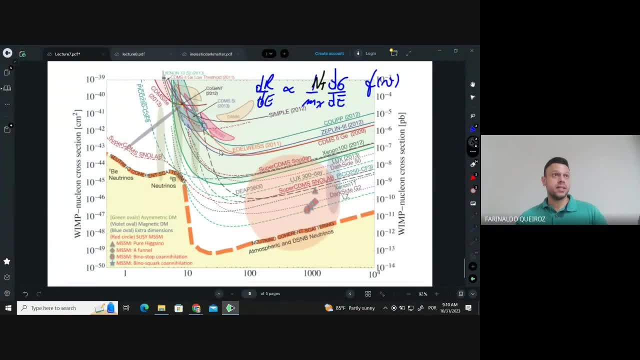 Which is related to the exposure, the volume of my detector. So as I increase the volume of my detector, my constraint becomes stronger at the same rate as I increase the volume of my detector. It's linearly dependent. So as I increase the scale up the volume of my detector. 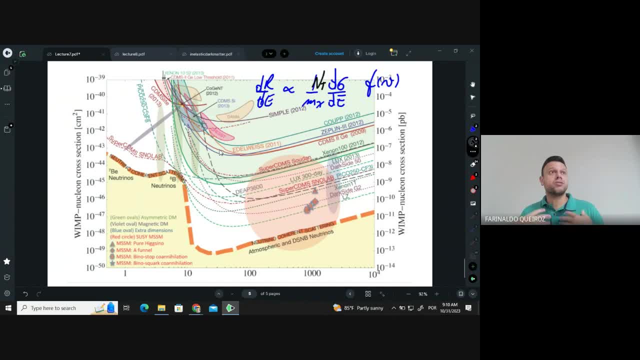 the number of targets, I increase my constraint in power. OK, Therefore, these detectors, they need to go bigger, Grow bigger and bigger and bigger, Because as they grow bigger, much bigger, and then my limit or my sensitivity to that scattering grows linearly. 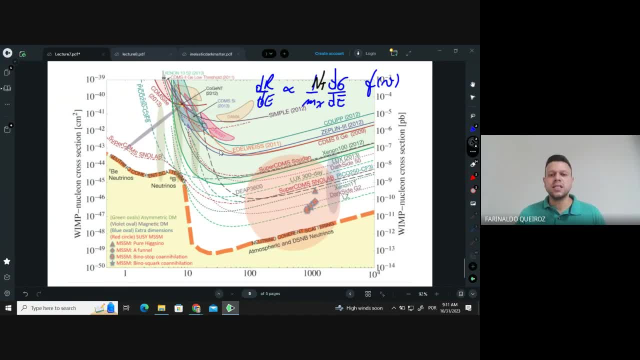 And then, for this reason only, you see that these detectors, which have limits, way down here, way down here, that's happening simply because they went from one fiducial volume to the other. OK, We're just increasing the fiducial volume of the detector. 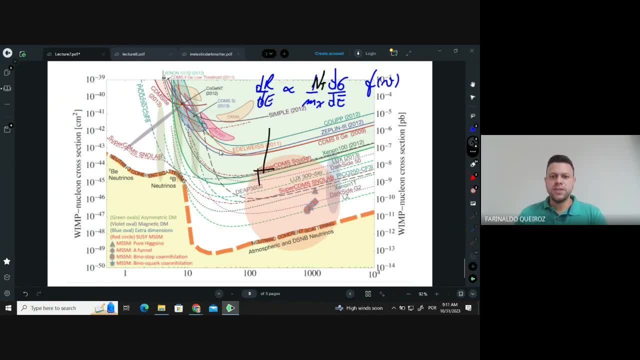 Fine, OK, So that's why you can move down by scaling up the fiducial volume And the reason why some detectors have a curve like this and then eventually they have a curve like this. So the reason why it moved down is because they increased the volume. 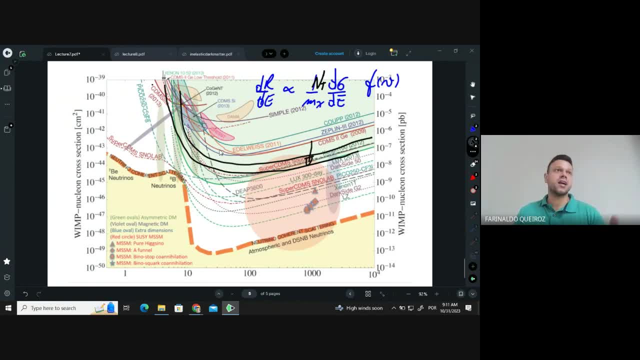 The reason why now they're covering up the volume- they're covering lighter, dark matter masses- is because they got a better way to reduce the energy threshold. As you reduce the energy threshold, you can cover smaller masses. Remember, Because this energy threshold dictates the smallest mass. 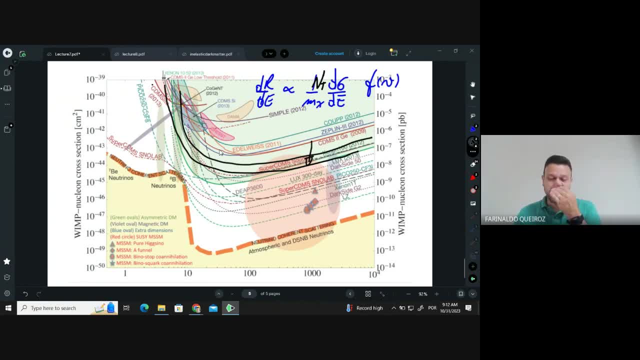 you can probe for a signal, you can probe with a given signal. OK, So that's the way you can move. You can move downwards or to the left, and then it has to do with the energy threshold and the volume, the fiducial volume, of your detector. 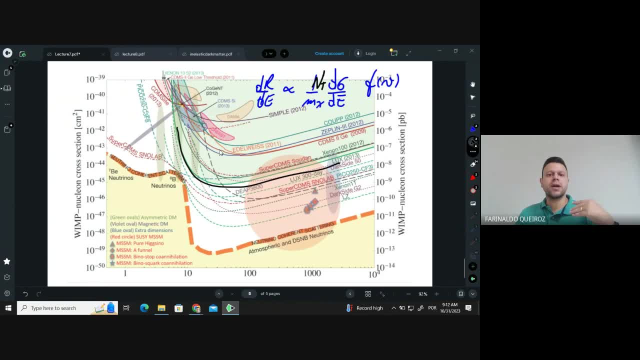 Obviously you can also scale down if you have a better handle on the background. OK, If I control more of my background, my constraining power becomes more effective. The more I know about my background, the better the constraint I can get on dark matter scattering. 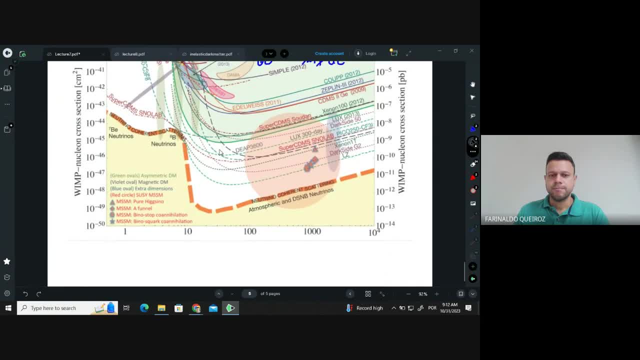 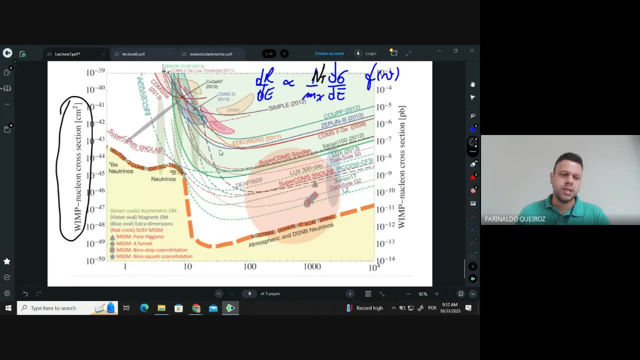 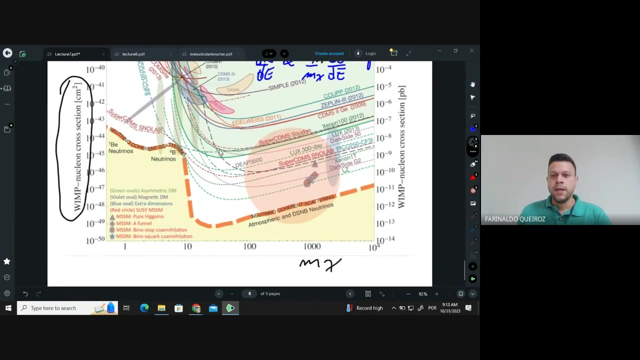 Make sense. OK, And as you see, As you see here, what I have in the x-axis- now let's discuss in more details- is the dark matter nucleon scattering cross-section. In the x-axis we have the dark matter mass. 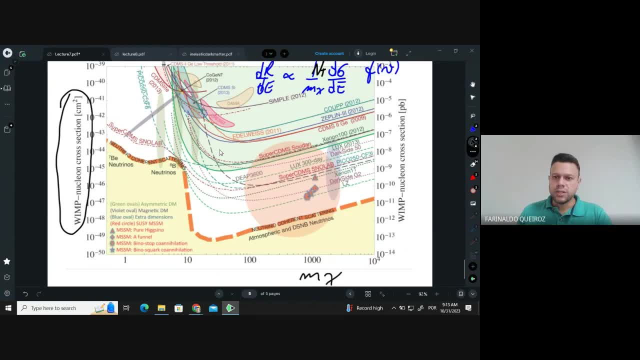 So you see, now we are probing. So this xenon and ton, which was the latest limit basically in LZ, this is the projected limit. OK, Xenon now is today's current, So this one right here around there. 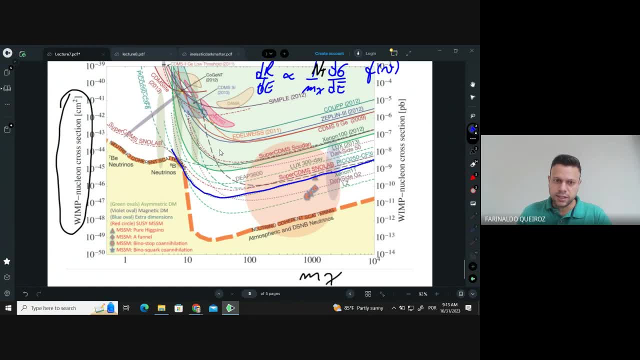 It did not go as good as they projected, but it's similar to this bond For cross-section around theta minus 46, which is roughly what they probed For dark matter masses between 10 GV and 100 GV. That's in GV units. 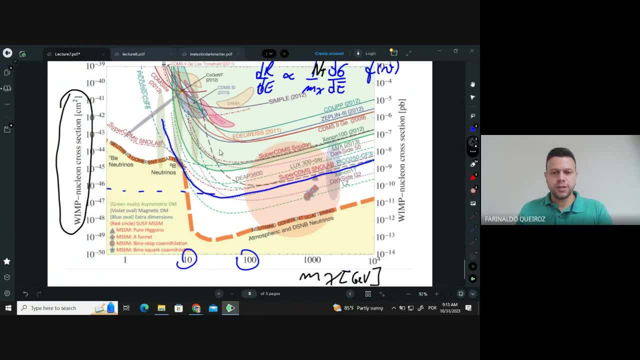 So they probed cross-section around theta minus 46 centimeter squared, Or theta minus 10 picobarons OK. So I want to point out some important things. So first one is that you see that there is a large portion of parameter space. 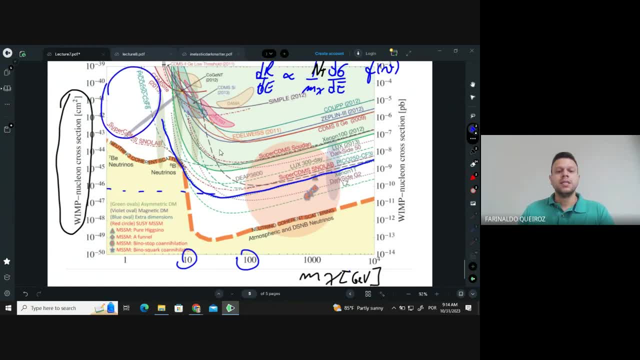 which is not covered towards light dark matter masses. This has to do with the energy threshold of those detectors, because dark matter particles became too light to produce a detectable signal And because of this new techniques are coming Now. they're rising now because they want to cover the whole parameter space. 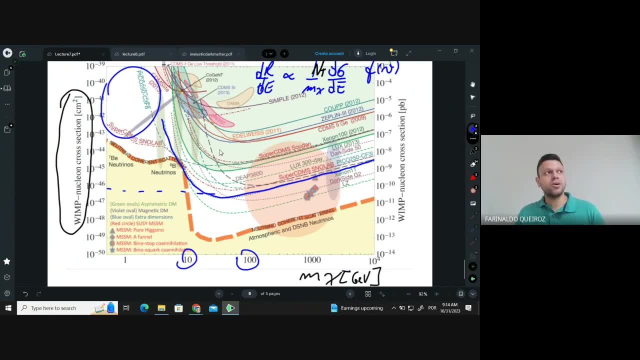 So how can we overcome the energy threshold of direct detection experiments and then cover light dark matter, particles, masses? How can I cover light dark matter The way they do it? there's many ways. One of them is using different targets which have lower energy threshold. 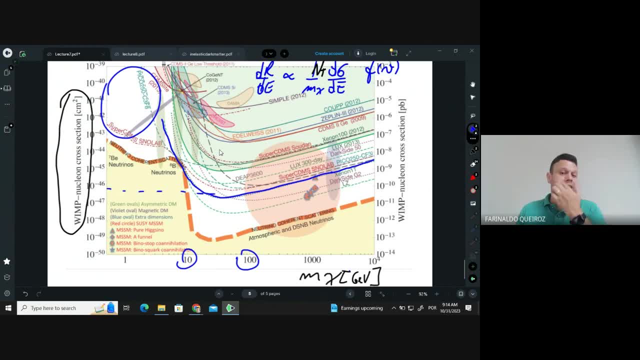 That's the easy part. The second one is: just remember that most of those detectors they require ionization, scintillation for instance, And having a second readout technique makes them harder, makes the threshold, those attacks increase, Because what happened is remember. 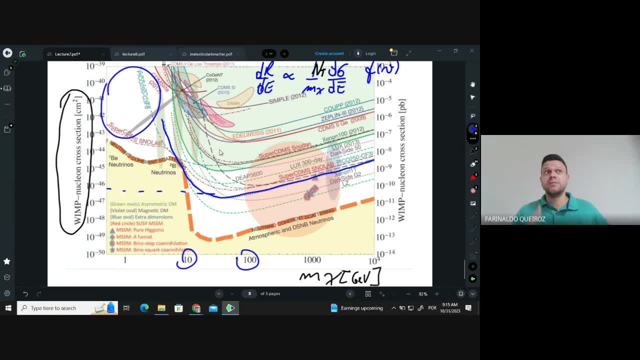 that the case of coagent we discussed with coagent had just ionization And the threshold of coagent was really small because they had just one readout techniques And it means this Ionization is very efficient to ionization refers to the amount of electrons. 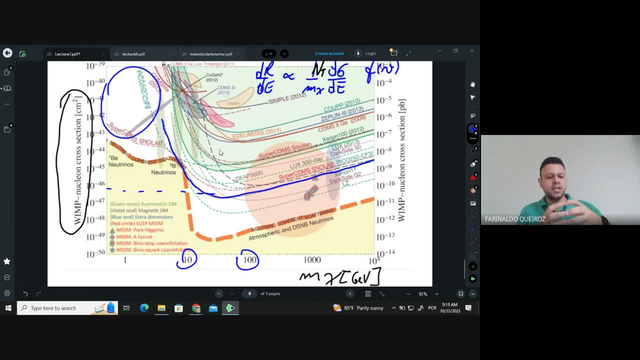 that I get. when something comes in, hits the nucleus and strips off some electrons. That's the ionization: You ionize the atom. This requires a very small energy threshold, because for most of the detectors we are talking about EV ionization energy. 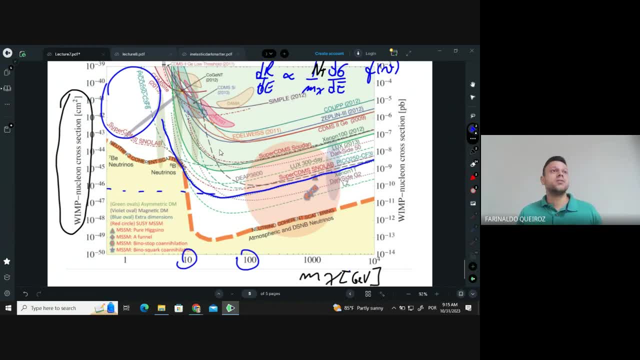 KeV ionization energy. So it's very small energies. So then I can I really lower the threshold if I rely just on ionization And some of those experience. what they did was they gave up on the idea of having a second readout. 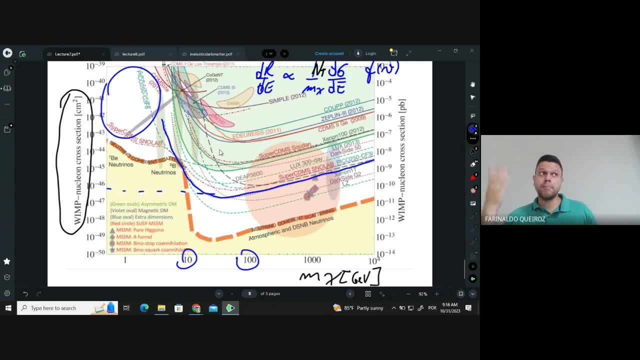 technique. Once you do that, you pay a price, which is you don't know so well the background, because you're paying a price. But with two readout techniques you have a better handle on the background, But you gave up on that. 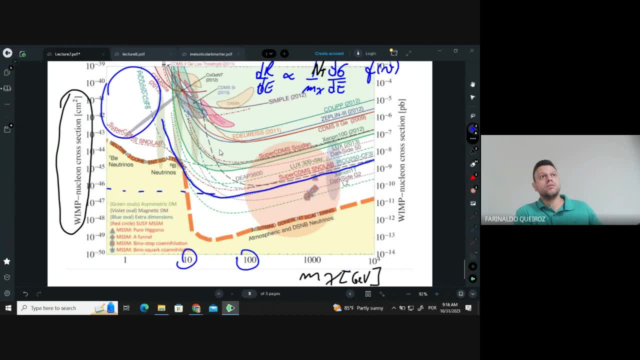 At the cost also to probe light and dark metaparticle masses. But then it's tricky now to distinguish signal from background because you don't have to read out techniques, Because remember of the xenon we had. The xenon was the time it takes for S1 and S2 signals to appear. 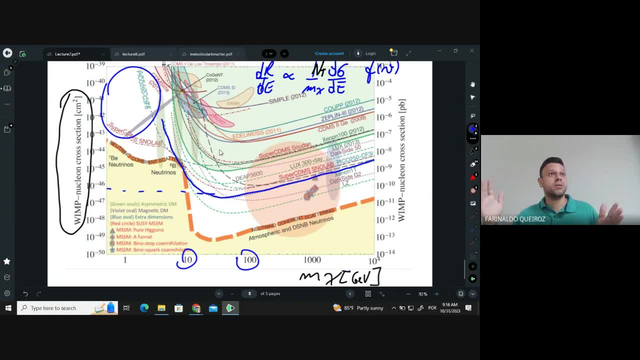 is one of the ways how they can distinguish signal from background, But there is not just S1 and S2. There's just one S1.. So now, how are you going to distinguish a signal from background if you have just S1?? 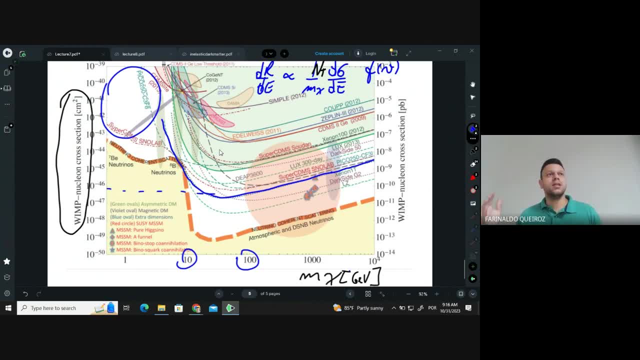 So they have to really know really well the background to say, look, I'll observe, Sorry, I'll expect this number of events from background. If I see something more, it's a signal They have to have a very good understanding of their background in order to claim any dark matter signal. 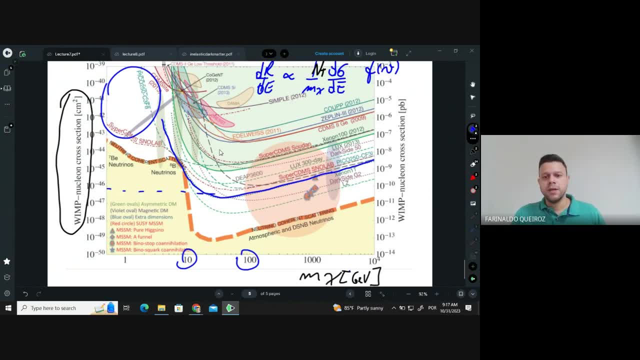 to observe the observation of any dark matter signal. So it's tricky in this sense, But some experiments have given up the second readout techniques to then be able to cover light dark metaparticle masses. And some other ways are to use different targets which 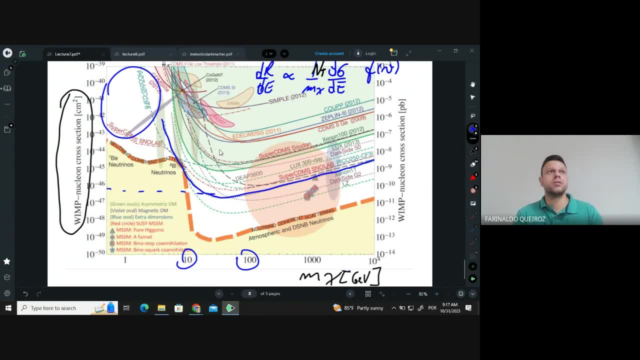 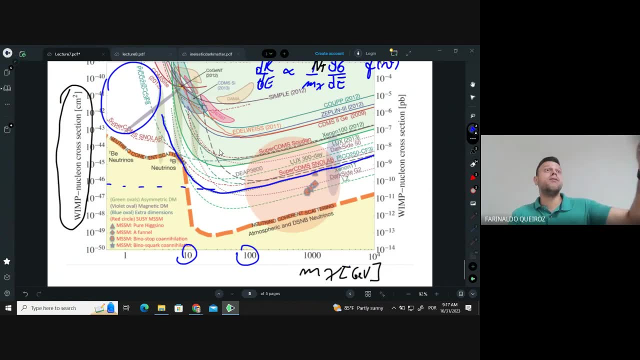 have. the material itself has a lower energy threshold and light targets, Because the lighter it goes, the less is the minimal velocity I need to produce a signal, Remember. So, for instance, everything is related to reduced mass. So as I increase, if I have a, this is visible. 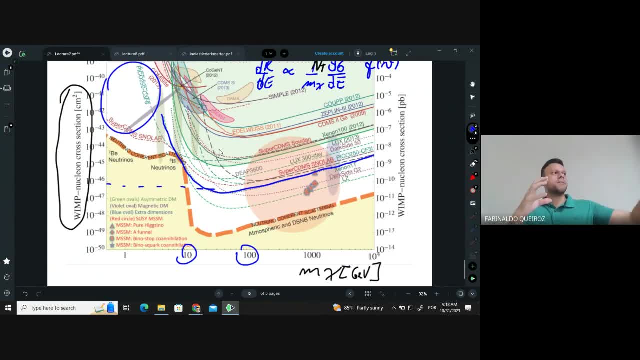 Let's say I have a ball really heavy. Comes a light dark matter particle hits the heavy ball. Well, the energy for me to see any vibration in this ball. it's tricky right, Because this is a heavy ball. 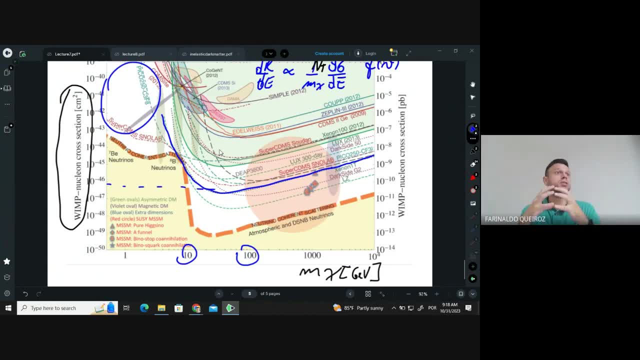 It's a heavy nucleus. The light, dark matter, comes in. it won't produce any visible signal, But it is, As this ball becomes, very small and light. if a light particle comes in, it will bounce this thing And I'm going to see it because it's bouncing. 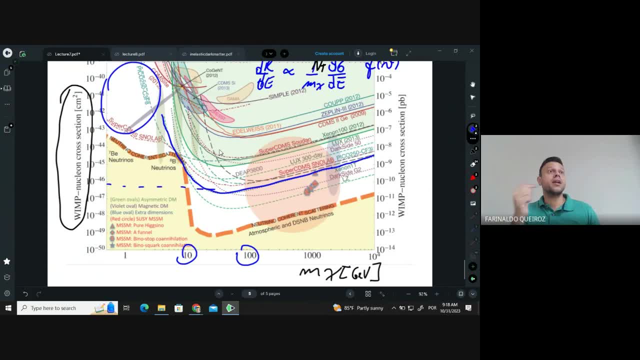 because it reduced the mass of the nucleus. So as I go to lighter targets, I'm becoming able, just from kinematics, of increasing the chances of observing a signal right. That makes total sense. Then, on top of that, if I use these balls or the materials, 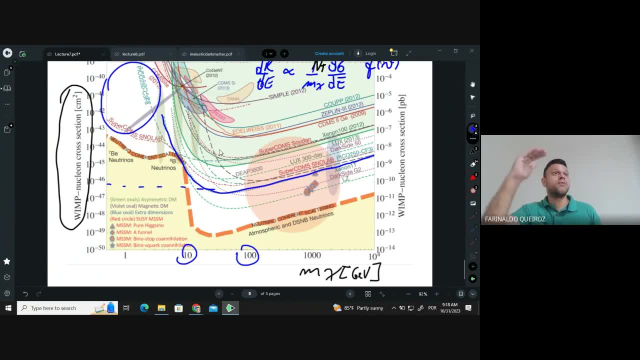 which have a low energy threshold, from going from the valence band to the conduction band or the ionization energy the energy requires to strip off an electron. then I can probe again: light dark matter particles. OK, The smaller the energy, it means the smaller the mass. 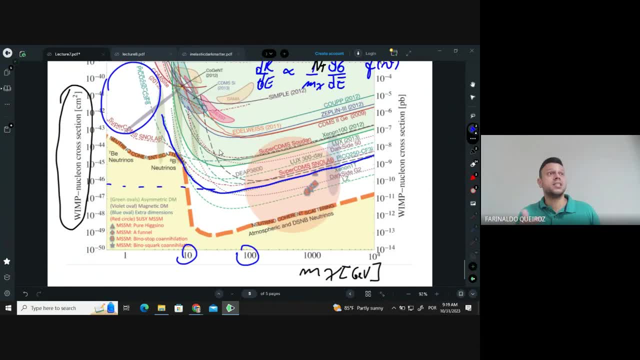 Because the dark matter mass, dark matter, energy it has is just kinetic energy, mass v squared. So the mass I already know is the same for all of them. It's a max or both mass. The only thing I can change is the mass. 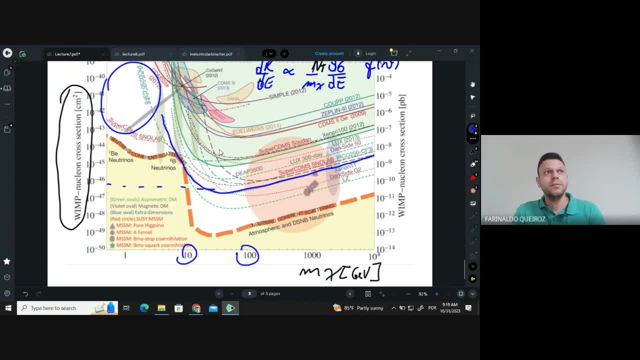 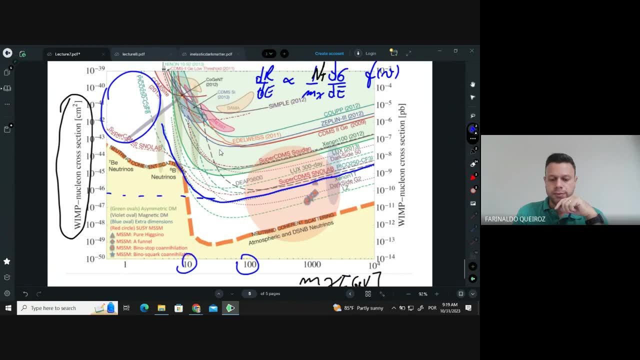 OK, OK, Fine. So another thing I want to discuss in this plot is the neutrino floor. So the neutrino floor refers to an irreducible background coming from neutrinos. So this part here, this corner right here, is solar neutrinos. 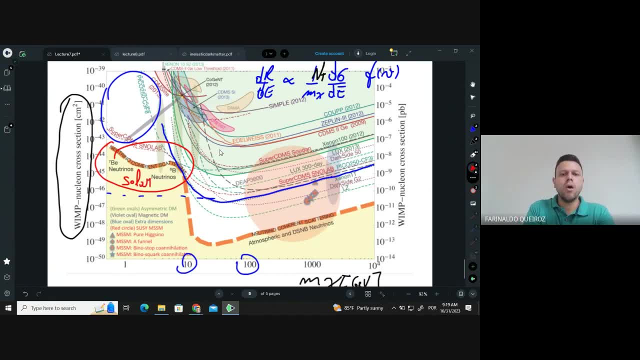 So these solar neutrinos have the same energy as the light. these solar neutrinos are well measured and they come either from beryllium or from bottom decays and they produce neutrinos. they always produce neutrinos. we detect them, but these neutrinos, 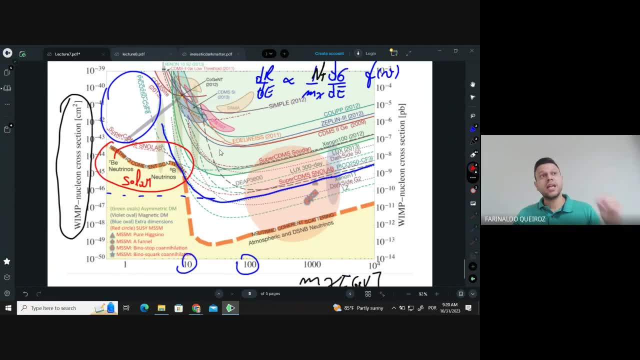 are coming to us all the time. however, that cross section is small. okay, it's more around 10 to minus 44 for this mass. so what are you saying this? this orange dashed curve is the following: what would be something i know? the flux of neutrinos coming. okay, i know the cross section, the standard model, physics. 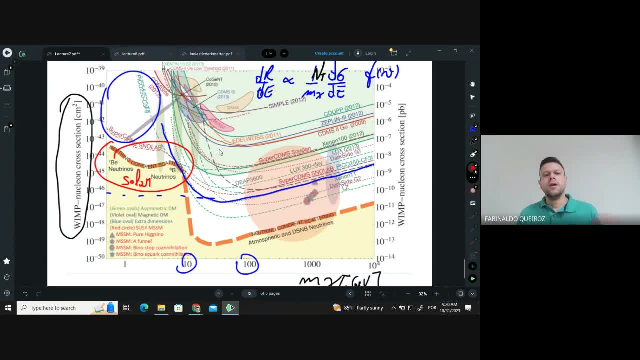 right, there's nothing new. it's not a model. okay, knowing that these neutrinos is coming, are coming towards us. they are passing through the earth because they are weakly interactive. massive particles- right, interacting massive particles, they're coming to us. the cross section i know is: 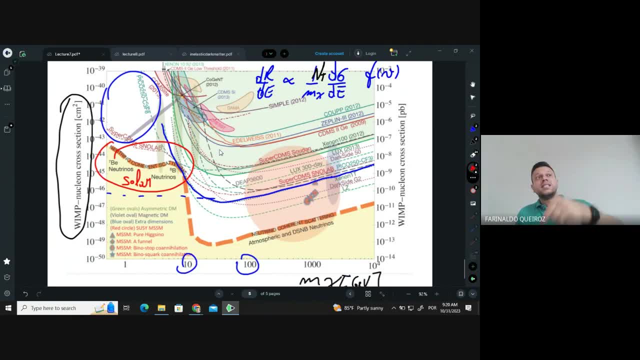 standard model physics. what is the signal they produce in my detector? uh, they produce this number of events. this number of events is small. well, if i'm trying to probe this region here in blue, then the number of neutrino signals they produce is small, because that cross section is small: 6 minus 44.. okay, because 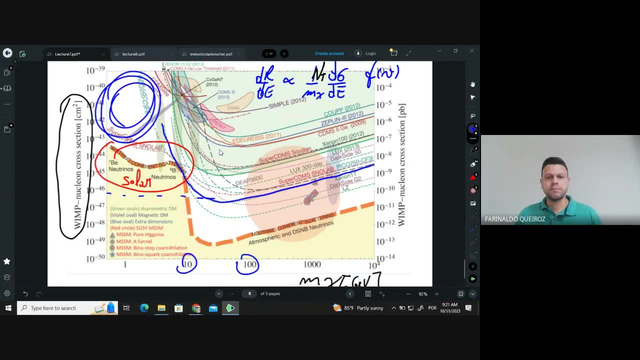 the number of neutrinos is smaller, the cross section is smaller, the amount of events they yield right. so i'm probably here. but as i push down the, the, the sensitivity of my detectors, as i'm going down, i'm- i wasn't here probing here, and then i'm probing there and then i'm. 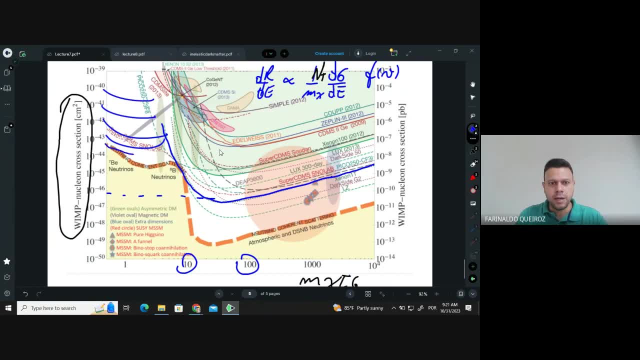 probing here, i'm probing here and then eventually i'm going to probe there. but now, as i not trying to see, a signal which is roughly producing a cross-section slimmer to neutrinos, now comes the question: how do i know if that signal was produced from a dark metal park? 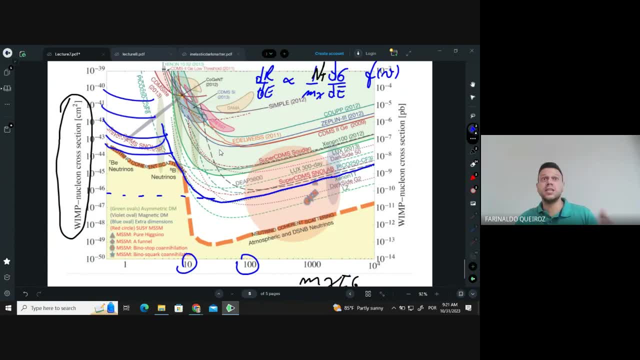 whether from a neutrino, because the signal is the same, is a neutral particle, comes in weak, does interact strongly, weakly and just scales, does that does not, does not have electric charge. it just scatters off a neutron, bounces, strips off some electrons, and i measure these electrons. 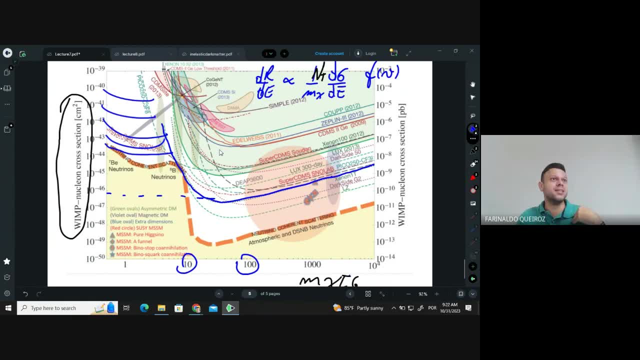 i know which direction is coming. it's coming from the sun. dark matter is around the whole galaxy. it's coming just from the sun. so if i know it real, if i somehow can detect in which direction the flux was coming from, then i can potentially potentially separate neutrino signal from a. 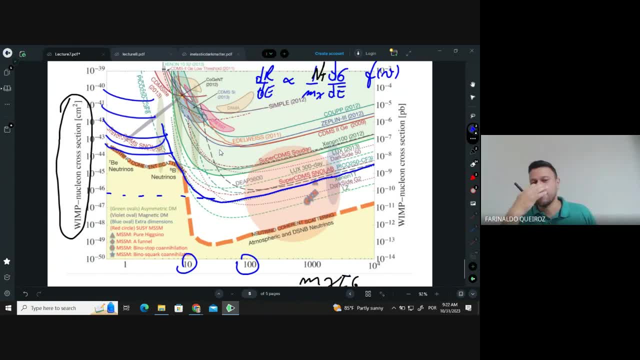 dark matter signal. okay, so neutrino 4 is is irreducible, so you cannot remove it. it will be there no matter what. so the neutrino 4 refers to a reducible back round from the center model which mimics the effect of a dark matter recoil. 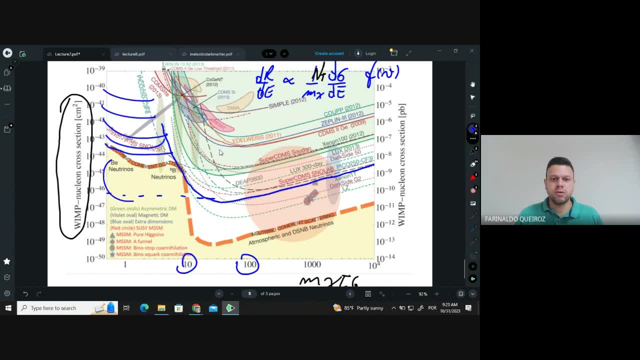 okay, and that comes from the sun, this one in the corner left and this one comes from atmospheric neutrinos and these ds and these supernova neutrinos. so you have solar, atmospheric and supernova neutrinos. they will always be reaching us, no matter what you do. we've measured. 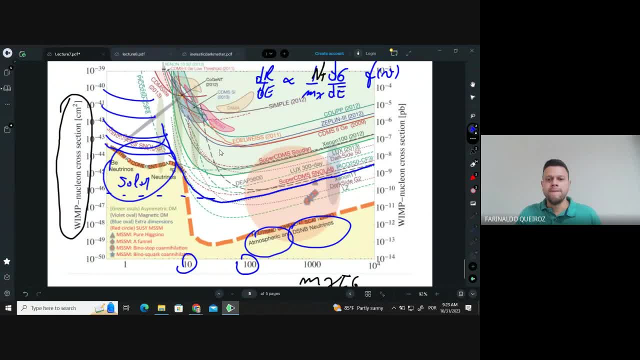 that's why this: there's a line there. we measured. therefore, as you can see, these experiments are like, uh, let's say, tours magnitude away, but as we move up, move down the sensitivity, we at some point we're going to be probing cross sections that will be like this red line here and then okay, and how? 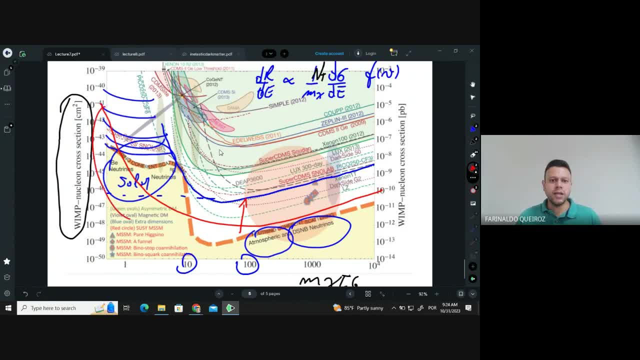 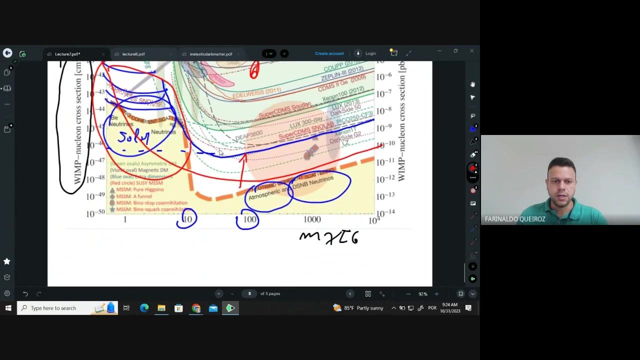 how come did you, how did you drive a limit like this one? you are deep inside the neutrino floor, okay. so if, in order to do this, you have to know really well yours, because you're saying, look, i observed some flux, but remember what they they do is and i've observed, let's say here, i observed. 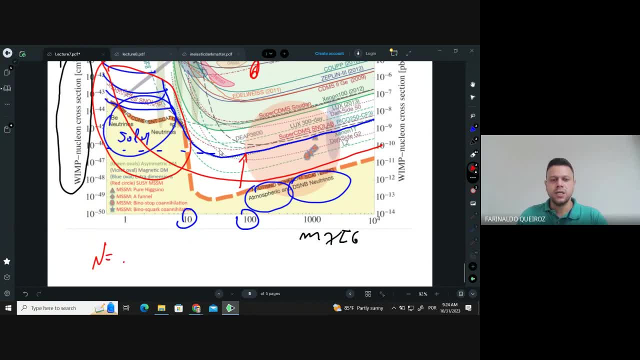 a number of events here and which is number of background, let's say back ground events, plus number of events from dark matter plus number of events from neutrinos. but i'm here in the red region. how do you know this is neutrino signal or dark matter signal? 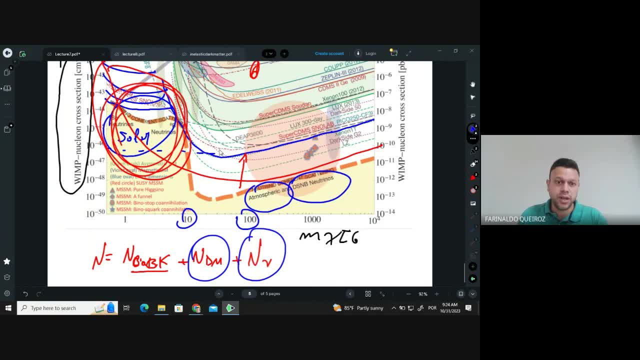 you can't know, you can't tell them apart, because if you are here, remember you. if you dare say: okay, i observe these number of neutrino events, but this, the measurement we have for neutrino flux down there, is not superior. you know, the dsl is only one in the next five seconds here and then not great enough. there are an additional information last part. or can i go where i really am? only am going through the Bear's nave. you can 여 چ espí property. okay, so 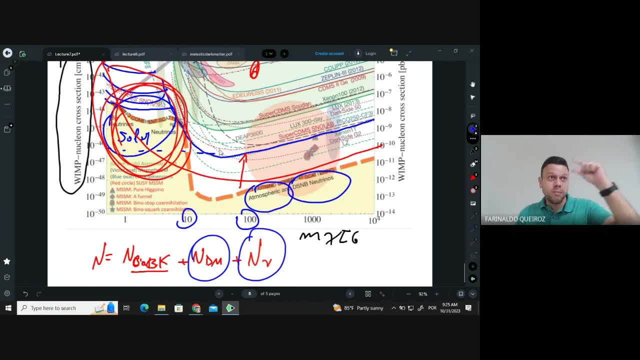 so precise. There's some error bars. So if you observe, the number of neutrino flux is huge, It's really big. So let's say you observe 10,000 events, But from dark matter you're expecting two events. 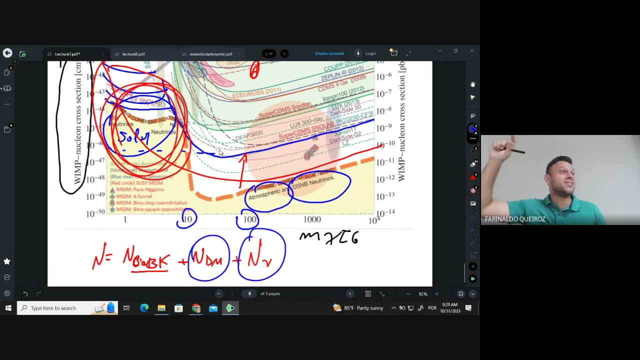 So you will always be within the error bars of the 10,000 events. There's 10,000 events plus minus 100. So the dark matter signal could be buried in this error bar and you wouldn't know. So that's why now you limited the sensitivity. 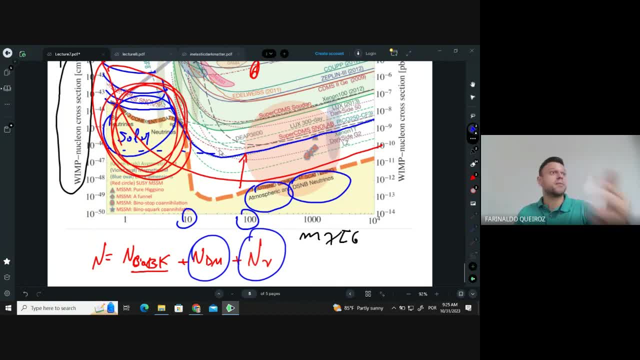 of the direct detection experiments of probing any dark matter signal, because the dark matter signal will be buried in the neutrino floor. That's the way they code. Oh, the dark matter signal is buried in the neutrino floor, is buried in the neutrino floor. 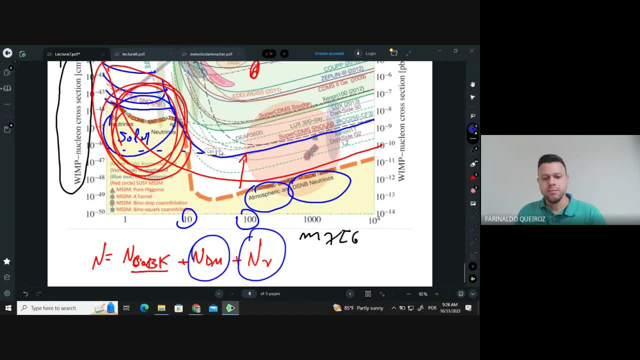 because you just can't tell the difference. Good, Any questions. I always thought about that. I mean in this block the dark matter has a function of the dark matter. In the case of neutrino floor, They are placed in the dark, the neutrino nucleus. 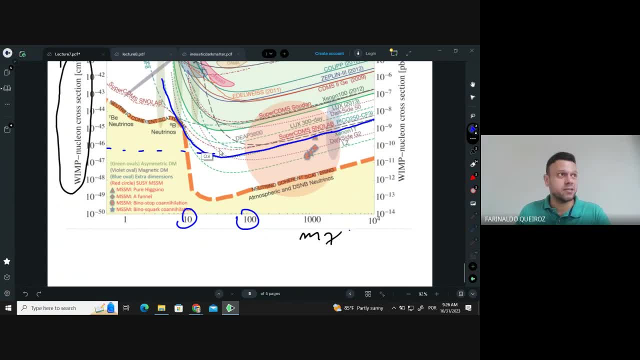 nucleon scattering cross-section as a function of the energy. Oh, OK, Yeah, sure Yeah, they have to convert into energy And the energy of the dark matter. The dark matter, I know, in relation to its mass. 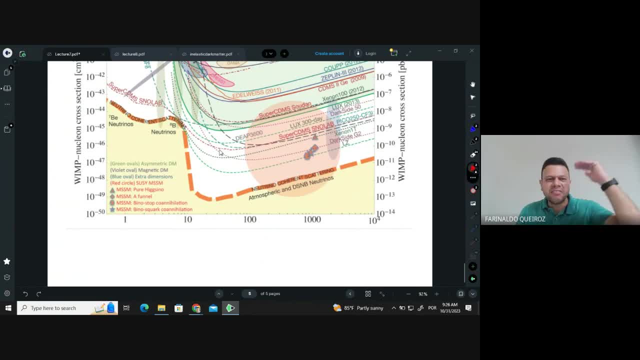 So that's why this line here is not really a face value line, because the velocity of, let's say, the energy of the dark matter is mv squared over 2, right, But v is not fixed, It's a velocity distribution. 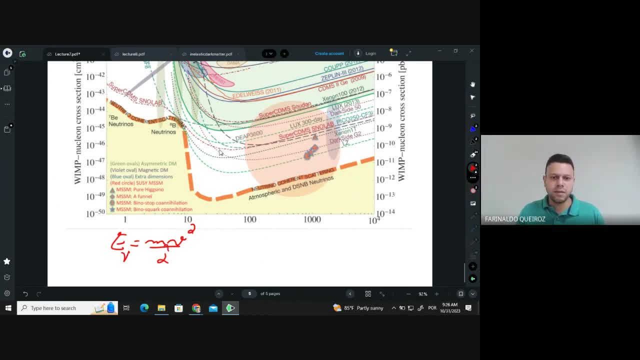 So, in order to convert neutrino and dark, relate these two things. right. So that's the energy of chi And the energy of neutrino is just the neutrino energy. But I want to convert this thing, I want to convert this thing back into this one. 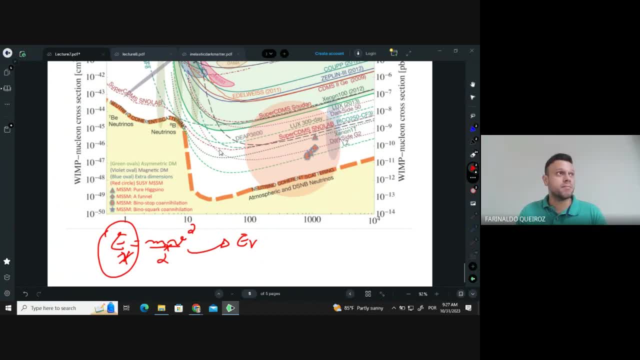 So I have to know the velocity, right, if they are the same. So let's say: now I make e chi equal e neutrino, Then I have m chi v squared over 2 equal e neutrino. Then I know the neutrino energy. 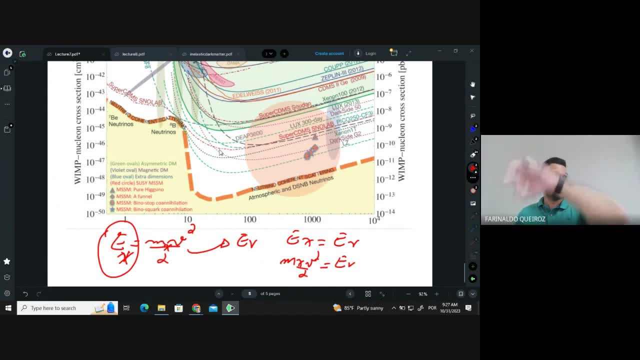 But what is the velocity you're going to choose? It's the velocity distribution, So that curve alone is not really a face value curve. That is some L bars, OK, OK, And there are some other things that I didn't mention. 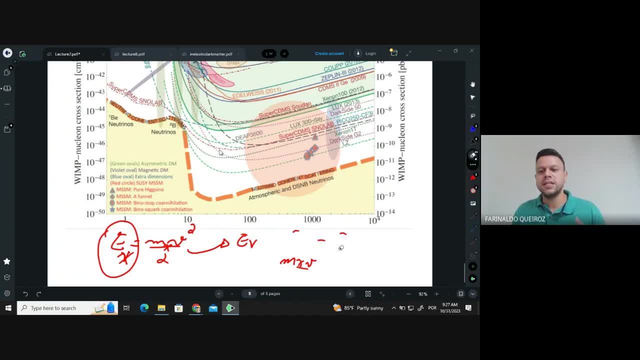 So, as you said, for instance, I said in the very beginning, I said: this neutrino floor is governed by standard model physics. right, That's what I said. But if it is not, that's it. And then he got the same. 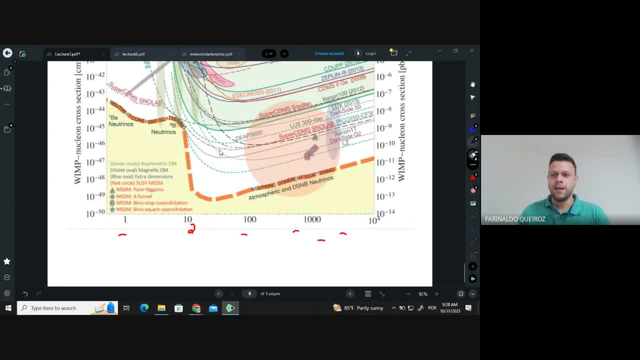 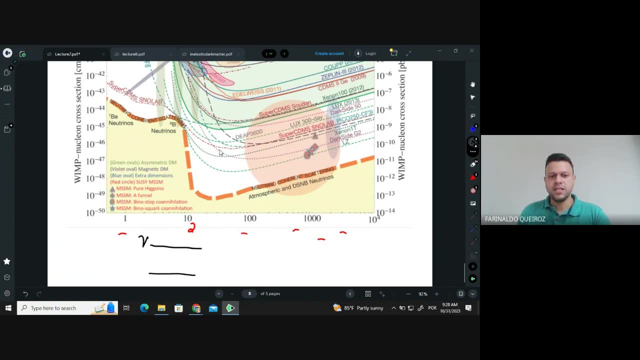 In which sense right. So let's think of the problem. So let's think of an interaction. So this interaction for neutrinos goes like this: A neutrino comes, finds a nucleus, exchange the z boson, the neutrino continues and then the nucleus is there. 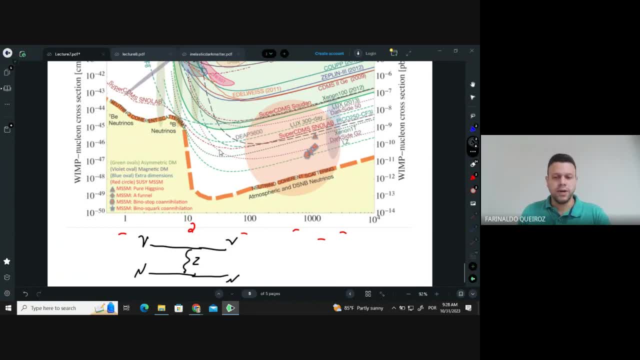 So that's a neutrino-nucleus scattering. OK, Fine. However, if I have this, so the cross-section for neutrino can increase a lot If this guy is much lighter than this one. which cross-section is bigger? This one, right? 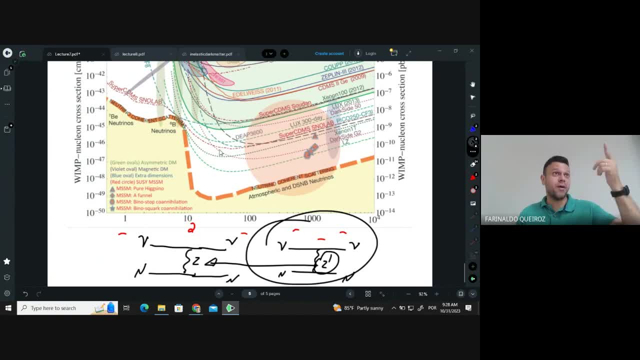 Because, remember, it goes one of the mass propagator squares to the fourth power at the end. So if I have a new vector boson which is lighter than the z boson, then the cross-section for neutrino-nucleus scattering is much higher. 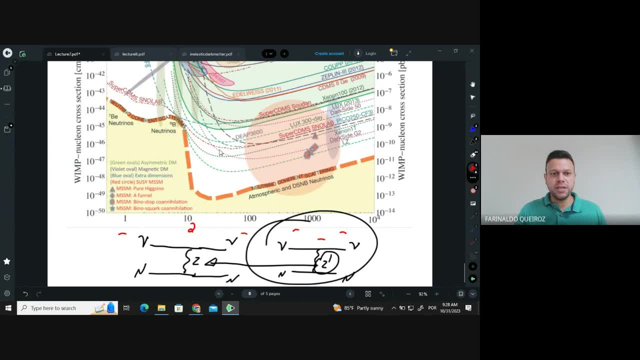 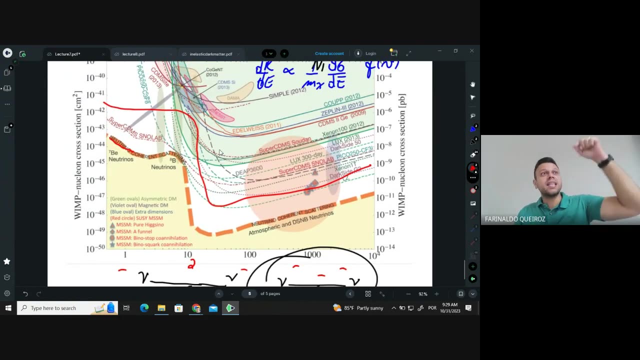 It's much higher means that instead of this curve being here, it will be around there. So it means at the end that even the current direct detection experiments might be sensitive to new forces in nature. So they are maybe underestimating the number of events. 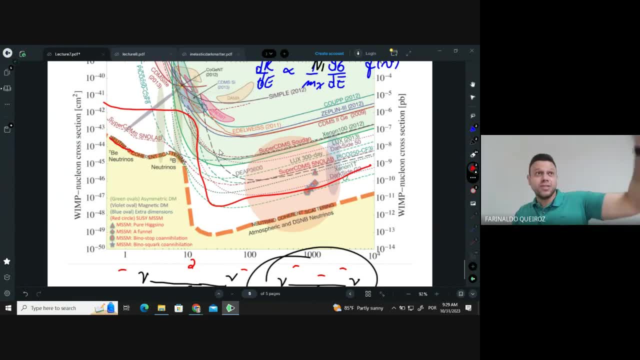 because they should have included the events coming from neutrino scattering, but they did not. OK, They underestimated the new physics contribution, because the new physics for them is not just dark matter. That could be also a new force. This is for dark matter detection. 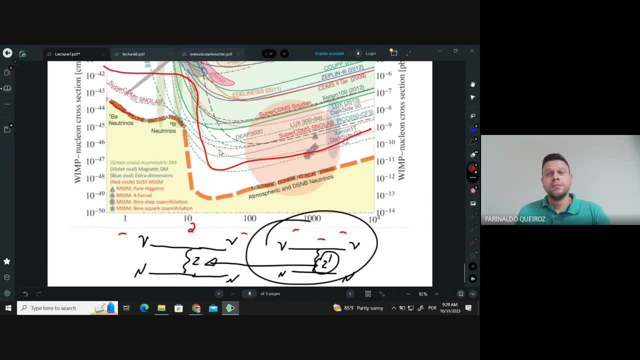 Are there any experiments that detect all the neutrinos There are That wouldn't detect dark matter at all. No, We have detectors just probing neutrinos. Yeah, but in experiments dark matter would be detected, but it wouldn't appear if it was there. 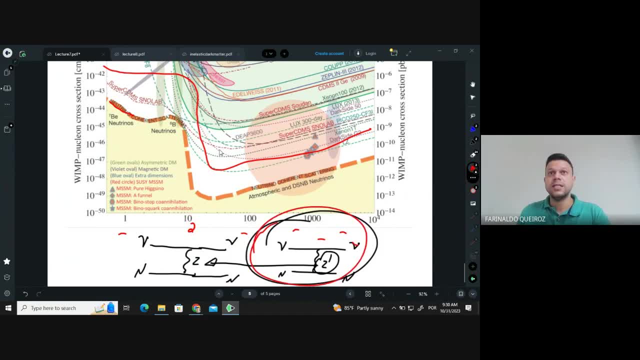 I know, But in this case here, the one I just circled, there is no dark matter whatsoever, right? This one, there is no dark matter. This one, there is no dark matter. Yeah, yeah, I know, I wasn't expecting that. 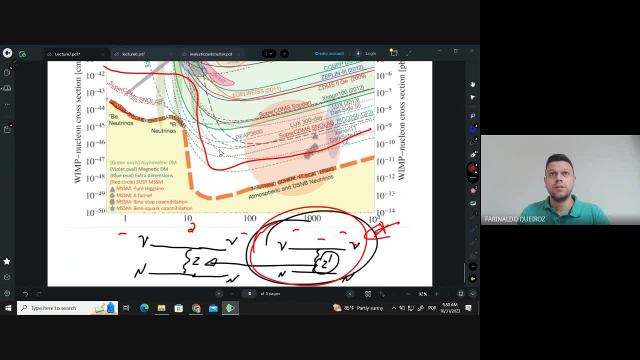 There are neutrino experiments, neutrino direct detection, experiments that are not sensitive to dark matter. Wouldn't we know if that was there or not? No, There are experiments that can distinguish between dark matter and neutrinos. It's only a neutrino experiment, direct detection. 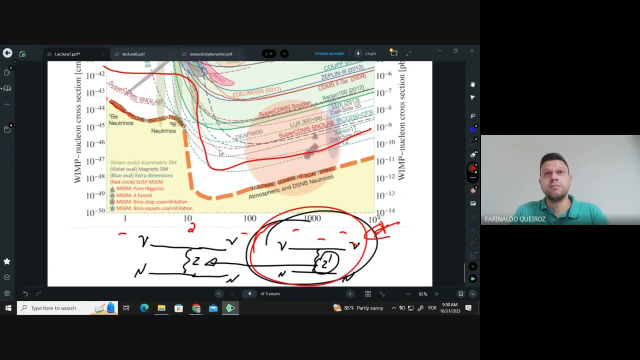 Yeah, the only seen neutrino is that. Yeah, Wouldn't we know if that perception, that scattering was possible from that experiment? Yes, but the constraints are not as restrictive as those from direct detection. So we can probe limit, We can place limits on new forces. 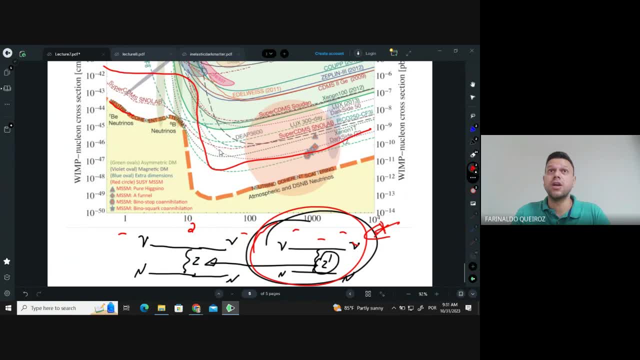 Using IceCube neutrinos, an IceCube detector, We can also probe. There's another one called Antares, which is the same. I mean we have others, ChemE3Net, We have SuperK Kamiokande, We have neutrino detectors, just meant to detect neutrinos. 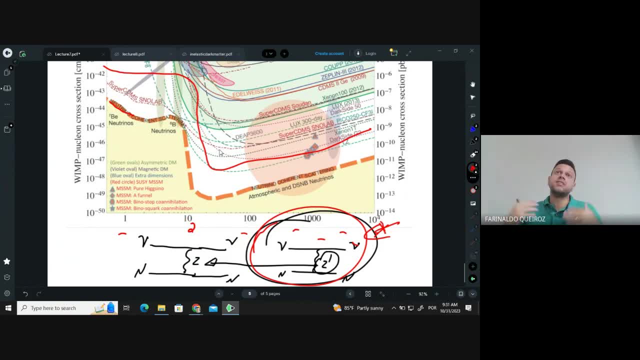 And using the neutrino flux they measure. They say, look, observe this number of fluxes of neutrinos. If there's a new force coming in, so then the flux should be different from the one I measured, then I place a limit. 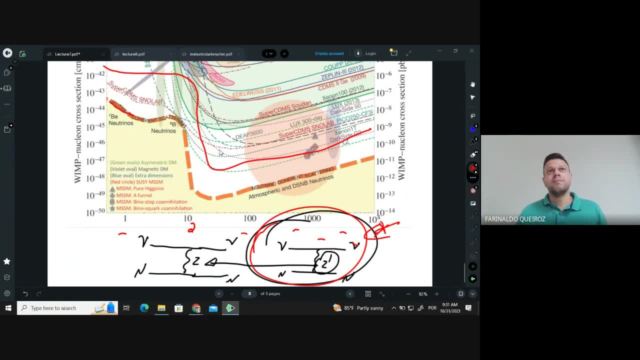 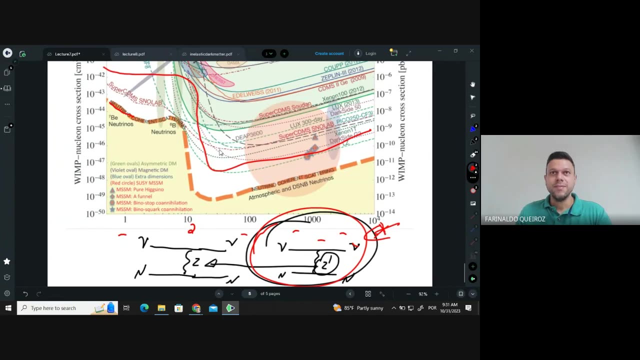 on the contribution from the endophysics. OK, But the level of precision they acquired, this is still far from those from direct detection experiments. So we cannot rule that out. No, And even the cross-section itself is very different One. we are talking about a neutrino interacting. 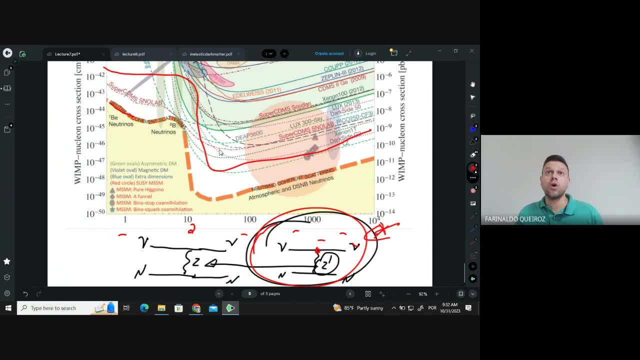 with a neutron, with quarks, The one that they measure in neutrino. telescopes are using just charged current: Neutrino, an electron and a W boson. It's just based charged currents And the lights they produce are different: bluish or less bluish. 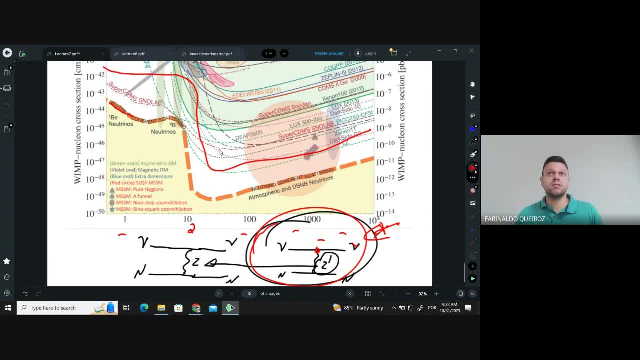 Depends on whether what's producing a muon or an electron neutrino, That's, an electron scattering, for example. Yeah, Yeah, Yeah, but this is just about neutrino experiments. But I mean, because it would be something that kind of mimics. 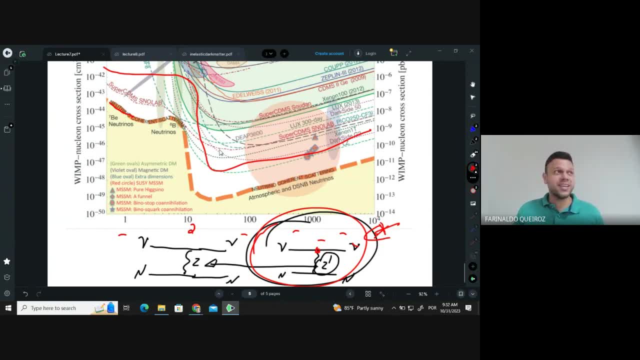 their methods. Yeah, For neutrino electron scattering, that's a different thing. Then you could also place a limit, But the bounds for neutrino electron scattering are much more restricted actually than these neutrino nucleus scattering, But it still is different. 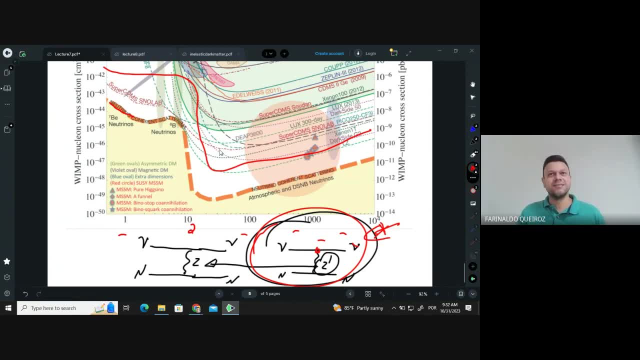 Neutrino electron scattering this neutrino nucleus. So in here you're probing a coupling between neutrino and quarks. OK, That's what you're probing. The one for neutrino telescopes, they're probing just the charged current in the leptonic sector. 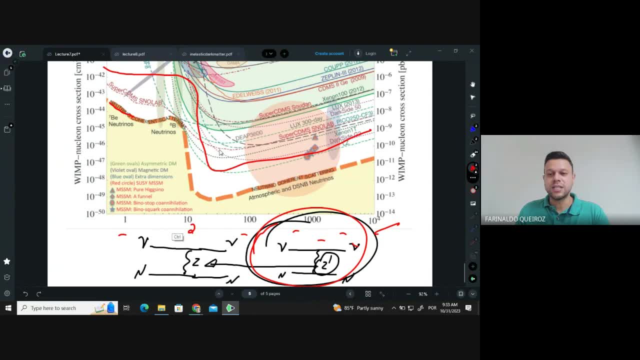 That's not the whole story, because there was a new result came from a collaboration called Coherent, which measured the neutrino nucleus scattering for the first time ever. They measured this in 20. 2017.. OK, So the lesson is direct detection is tough business. 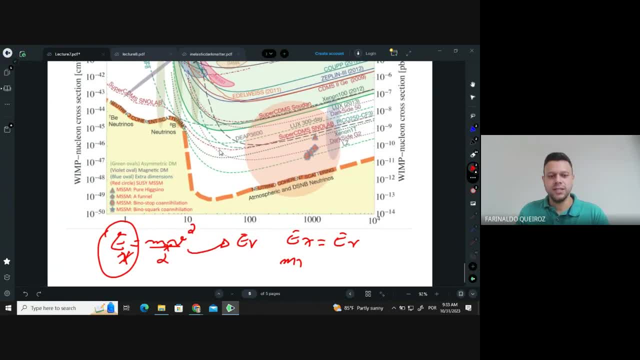 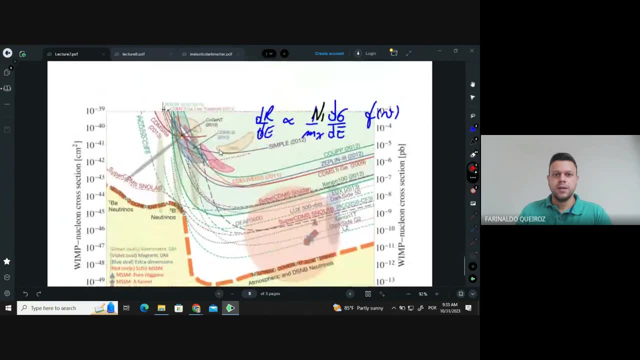 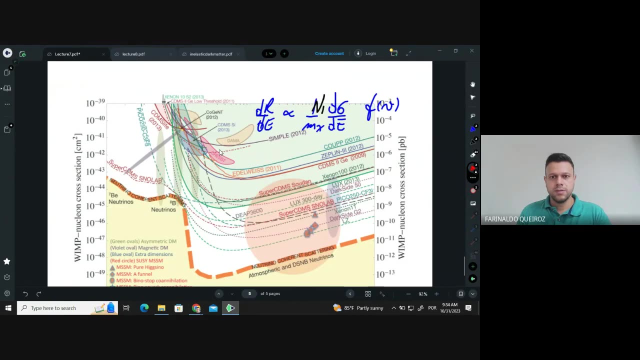 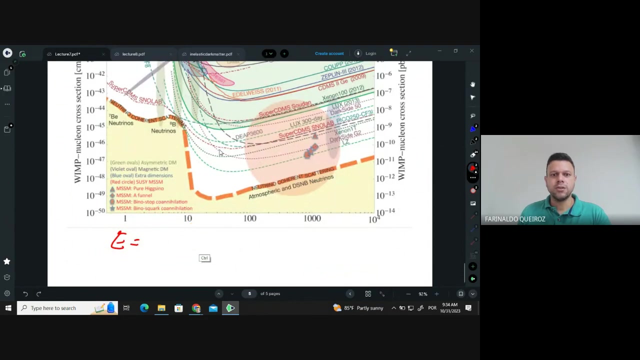 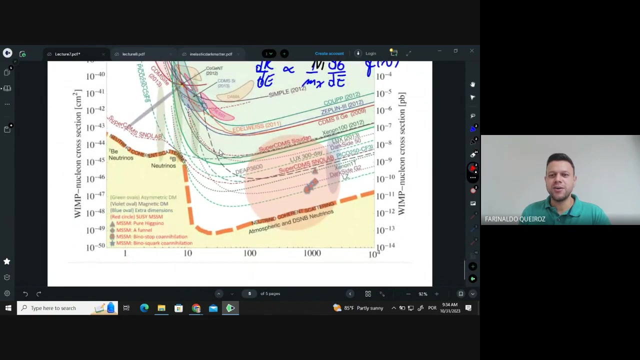 It's very tough. Is there any questions from this slide? No, OK, Hold on, Let me erase. What's that. What's that? Ah, OK, So they're just saying, for instance, this was from someone's lecture to hey, my favorite model. 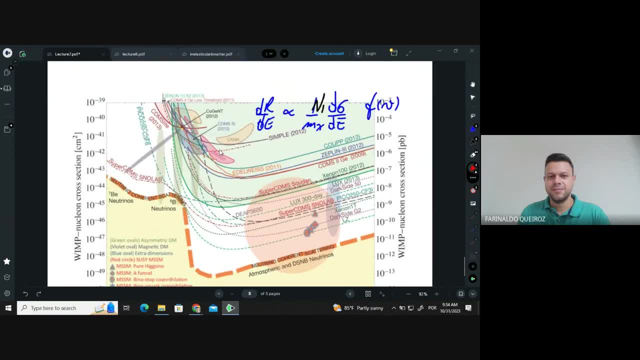 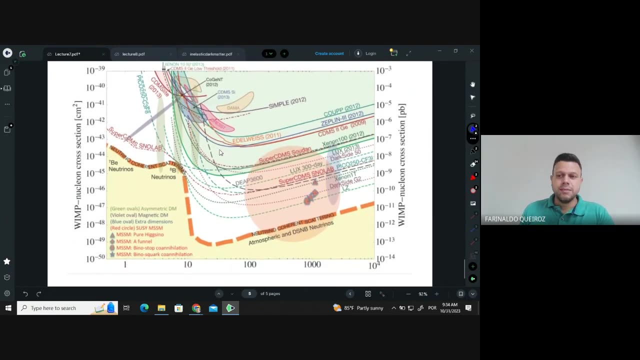 lies in this bubble, in this ball. OK, OK, That's what it is. So one thing I should emphasize also is that I'm glad for your question. because of this, Now I remember something. So typically people thought that dark matter- WIMP dark matter- would appear somewhere around. 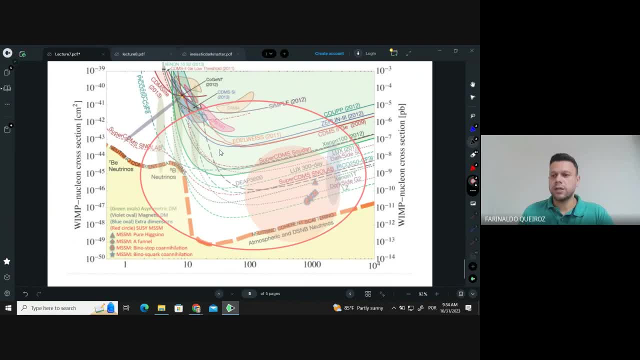 here. So that's where the region for WIMP dark matter would appear around there. So this is the vanilla, the expected region, where you see a signal. If you haven't seen so far, okay, there are two orders of magnitude still to cover. 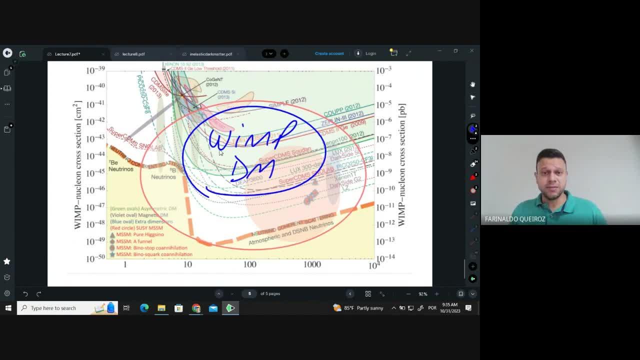 But you haven't seen any. And then people started realizing, revisiting their assumption about thermal production of dark matter. Was really dark matter thermally produced in the early universe? Was dark matter coming just from the abundance, just computing the chi-chi bar going to fermion? 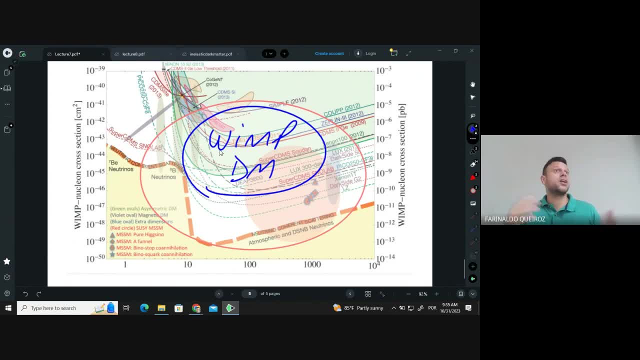 chi-fermion. What could be something extra? Could the other channels being produced producing dark matter, contributing to the dark matter abundance? Could be non-standard cosmology, something beyond lambda CDM, something extra, some extra cosmology would change the Boltzmann equation. yes, would change the Boltzmann equation. 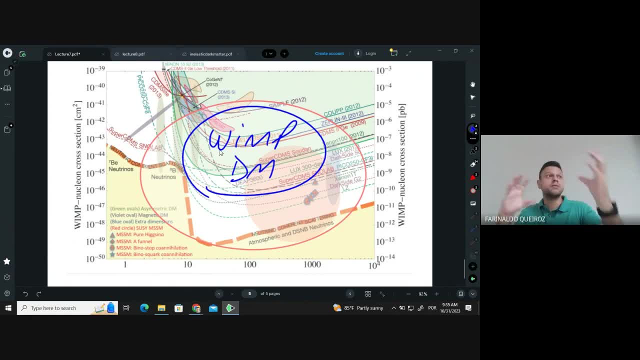 Where those regions, favorite regions, would locate. if you start changing your premises And then they realized that as you change your premise, then these favorite regions could be around here, could be around there, Could be around here, could be around there, And then you don't have now a fixed favorite region. 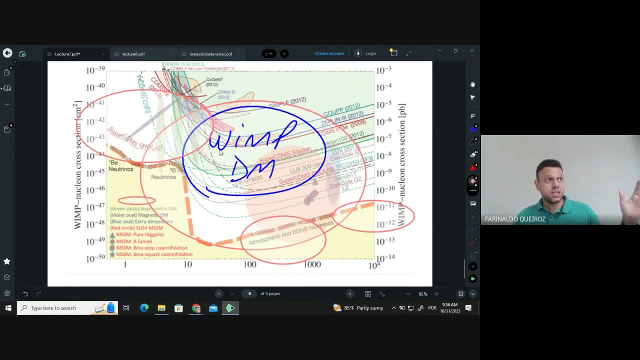 So this region for WIMP, which is just historically speaking, is just a region where people from supersymmetry expected dark matter to be, So this what people refer WIMP region. actually, you can just remove it and say: Susie expected region. 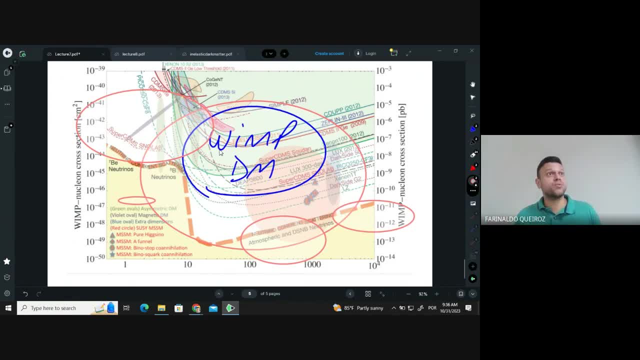 And that's what it used to be. So the WIMP searches were really driven, heavily driven by WIMP, by Susie. So to have an idea how seriously the American and the European community takes the dark matter search is the following: So DMSM, the Minimal Super-Symmetric Standard Model, does have a dark matter candidate called 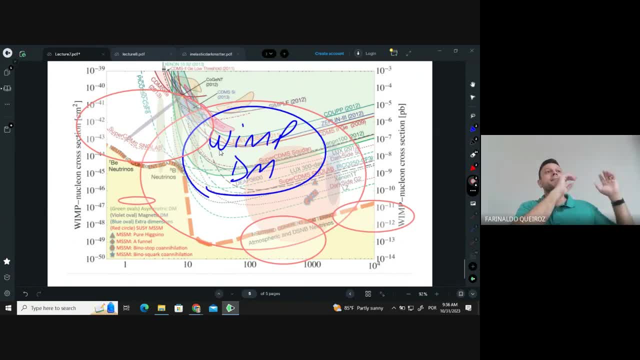 Neutralina. Okay, Okay, Okay. So the theory is that the experiment at which the drug detection experiments reach a cross-section, which removed the Neutralina, to be dark matter, they gave up on the MSSM. MSSM cannot be the theory because the Neutralina is excluded. 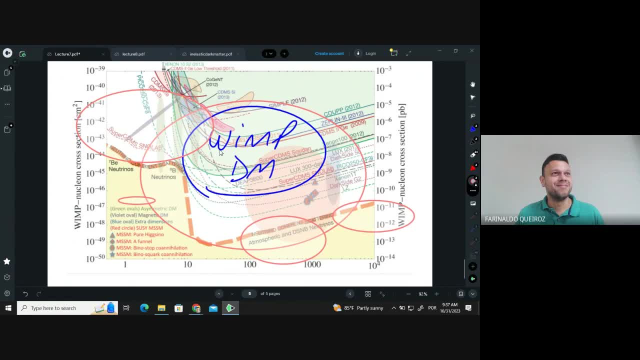 Because there must be dark matter If SSM. MSM is not a theory, So it has to be an extended MSSM. Okay, So they came up with another one: PMSSM, MSM, next MSSM: changing the supersymmetry. 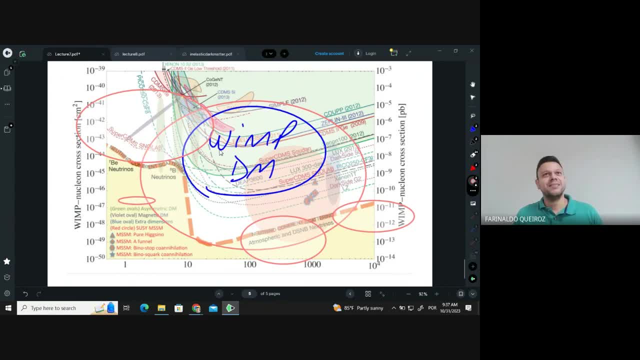 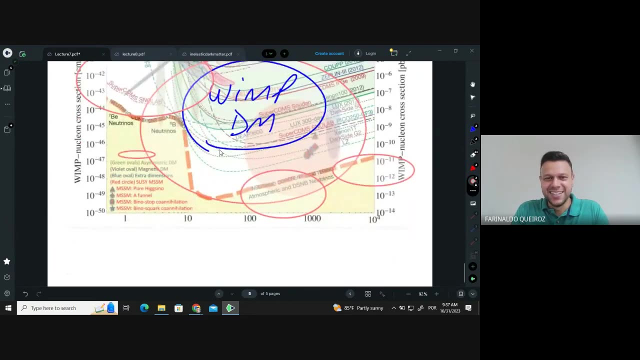 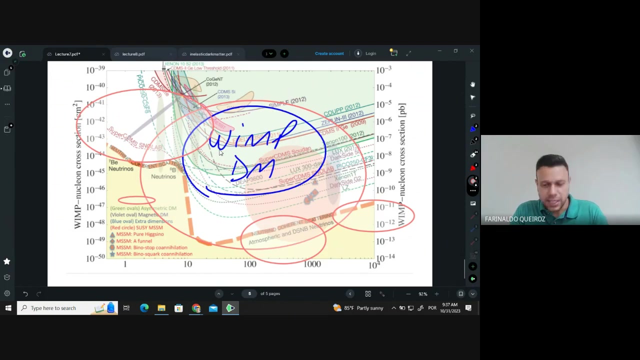 to accommodate the dark matter limits, So they are changing their theory in order to have a successful dark matter candidate. Okay, So that's how seriously they take the dark matter events. But they were also biased in some way Because they expected the signal to be there. but it doesn't have to be true. 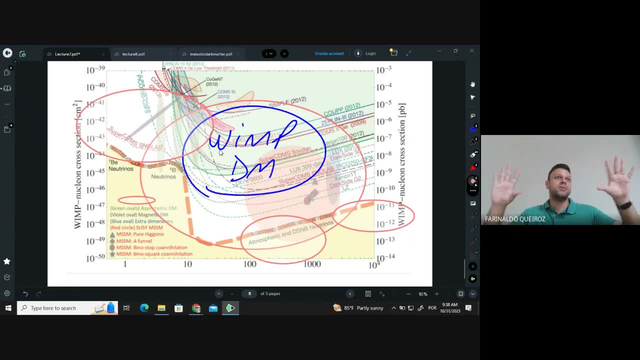 If? well, if you separate now dark matter from supersymmetry, because dark matter is the evidence, for dark matter is much more compelling than supersymmetry, which is none. Today, according to data right, there is no data favoring supersymmetry whatsoever- none. 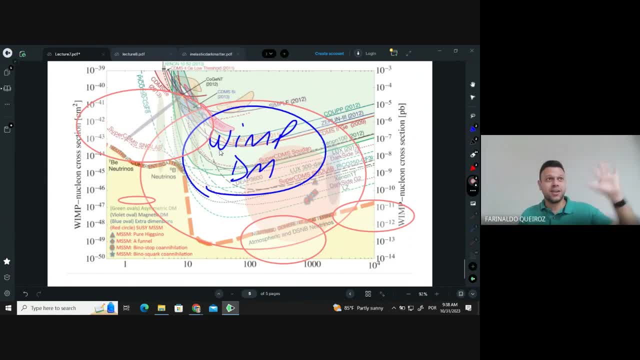 There are theoretical arguments but no data. And for dark matter we have data. Okay, And then if you separate those two, then one has nothing to do with the other. Then you can do have dark matter candidates, which has nothing to do with supersymmetry. 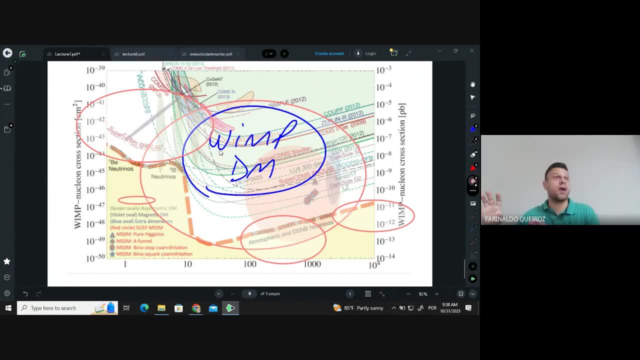 which can have different regions, where the relic densities is correct and doesn't have to be within the first ellipse that I drew in here in this region, right there, This one, This big one, Doesn't have to be there. It can be scattered in different places of this plane. 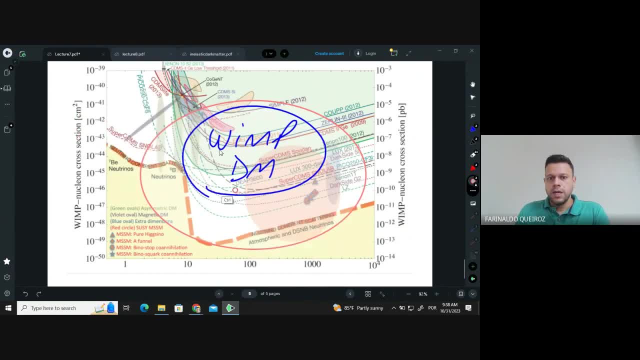 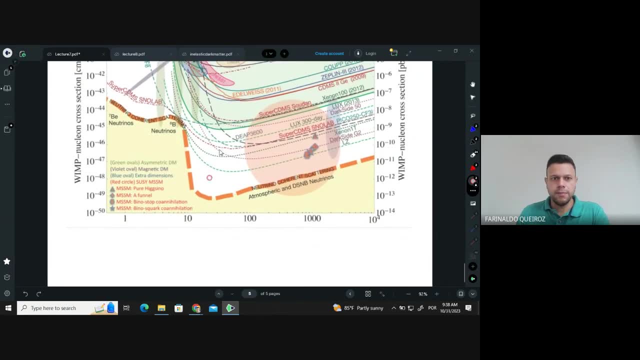 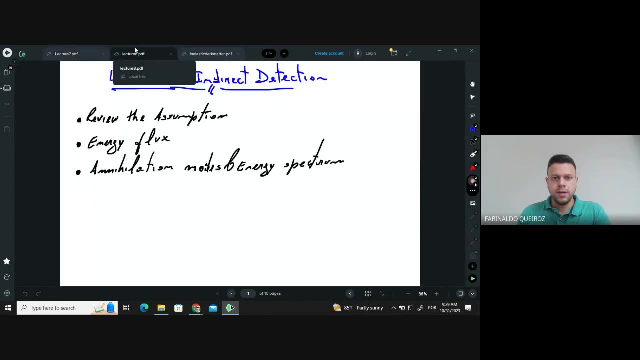 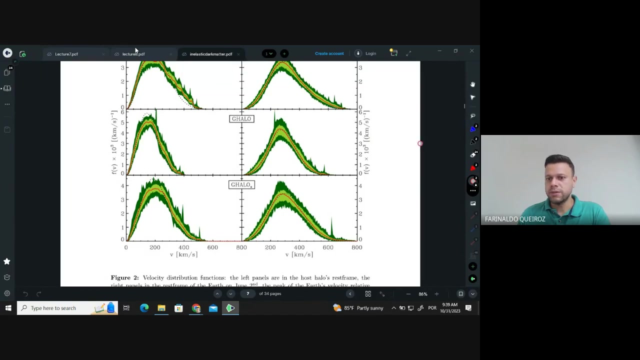 Okay, Any further questions? No, Okay, I think I'm done for this seven lecture. Yes, Before I move to direct detection, let me cover something that I haven't covered before. It's still in the aspect of direct detection, So you can see in this paper, this paper, what it is is about. people have simulated 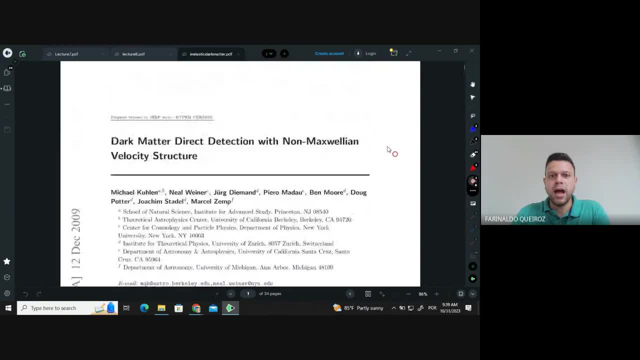 this is a very interesting paper. This is a paper. It's about the- I think it's the- the formation of our galaxy using dark matter particles. And one thing I haven't told you is that the density of dark matter in a galaxy is related to the velocity. 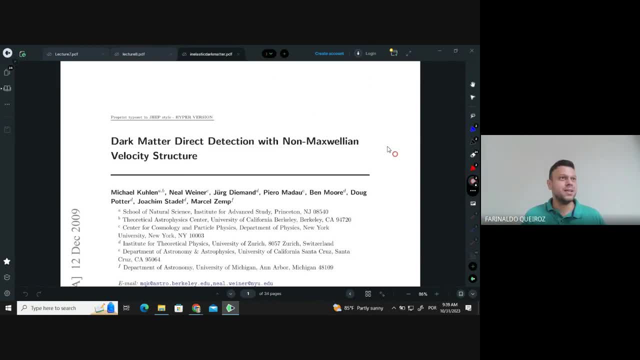 distribution of dark matter particles in the galaxy. So velocity distribution is not disconnected from the density profile, They are related. Actually, you have to feed in the velocity distribution to get the dark matter density. Well, it's sort of reasonable because you have to know how. 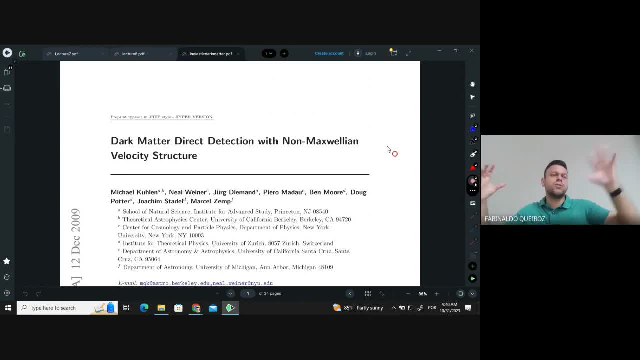 these dark matter particles are moving, to predict where they're going to accumulate in formed structures. So one is connected to the other, But in order to have a density profile that fits the data we see in galaxies. So you have this. You see the stars moving with some velocity: galaxy rotation. 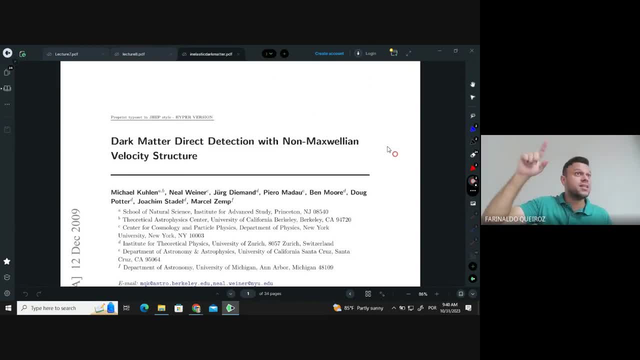 curves and so on. In order to fit the galaxy rotation curves, the velocity distribution you have to fit in in your simulation is a maximum Boltzmann, close to a maximum Boltzmann. So the data from the distribution of dark matter in 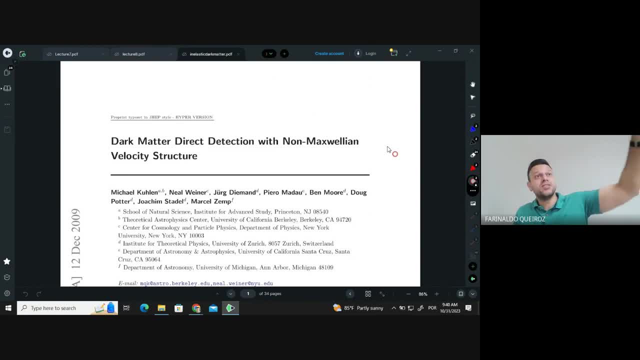 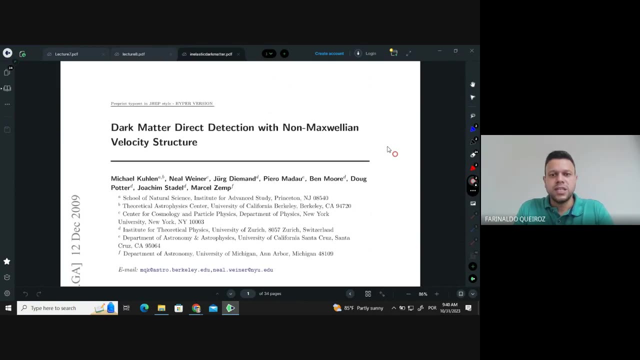 galaxies is telling you that the velocity distribution of dark matter particles to form a galaxy has to be close to a maximum Boltzmann distribution, And one of the first papers that discussed this is this one, So back in 2009.. First, now, let me show you how our community is very different. 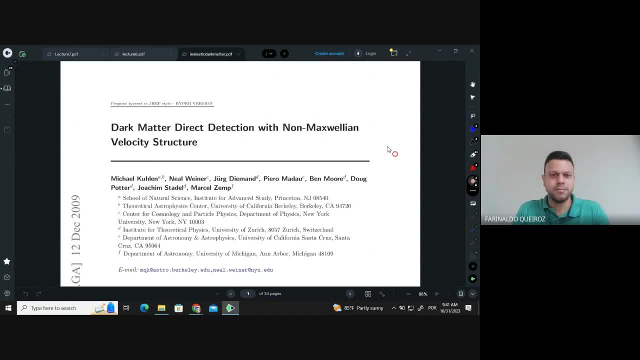 from others. This is a well-known paper And this well-known paper was published in Jhap, Not in Feast Review Letters, not in Nature. it is in Jhap. It is a well cited paper, published in Jhap. Okay, Thank you. 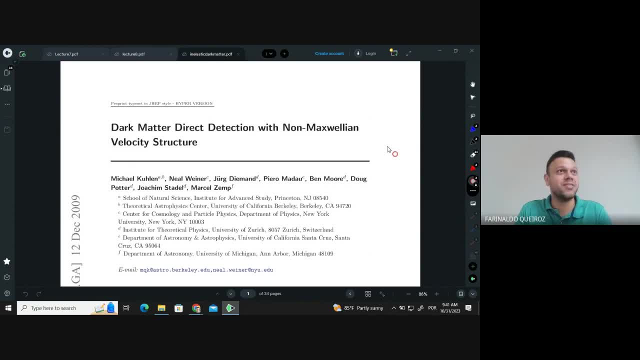 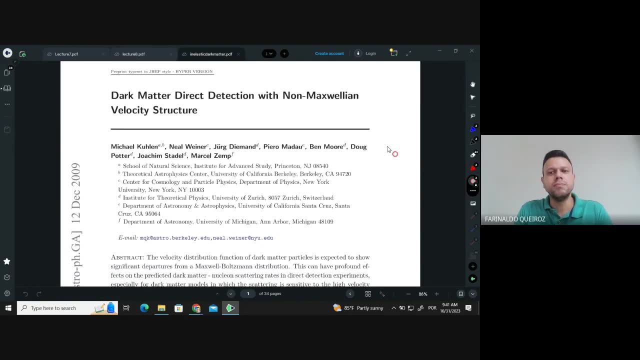 Bye-bye in nature and not in science and not in physical letters. okay, so what they discuss is was: what is the impact? could be the velocity distribution of dark matter be known maxwellian could be different from maximum distribution. that's what they're trying to assess. they were motivated by something. 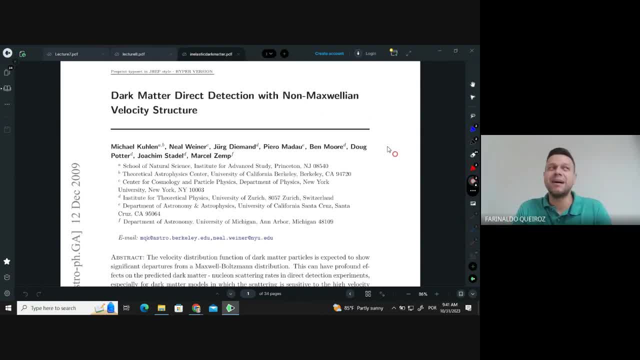 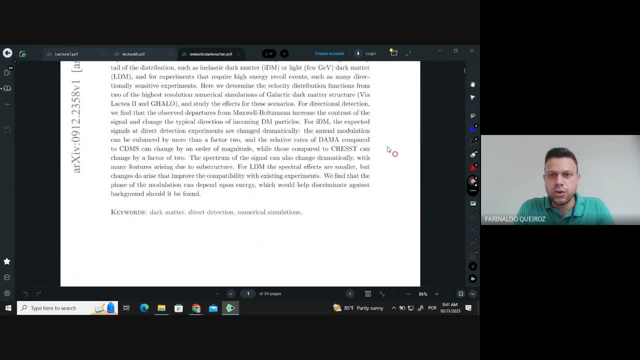 which is called the dhamma modulation. but i won't have the time to cover this, but let's, let's let me show you something. so they use two simulations: one is called hold on, one is called viado and the other one is called gallo. these two 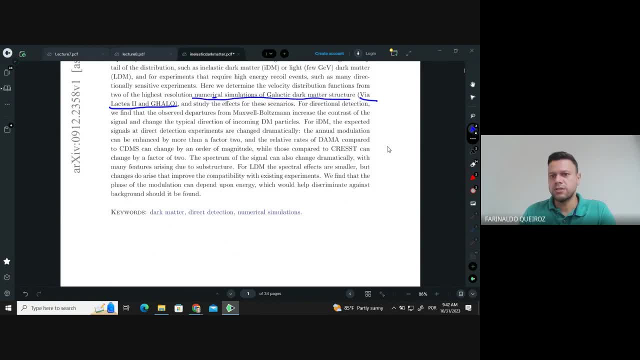 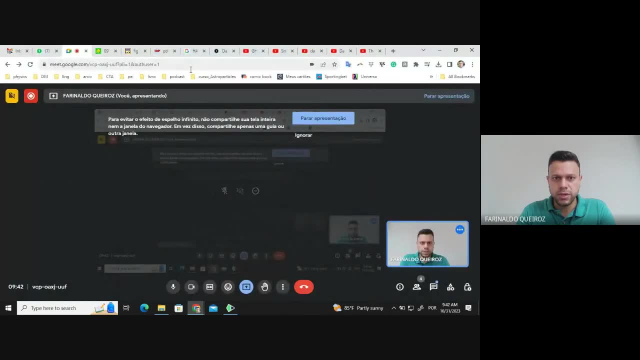 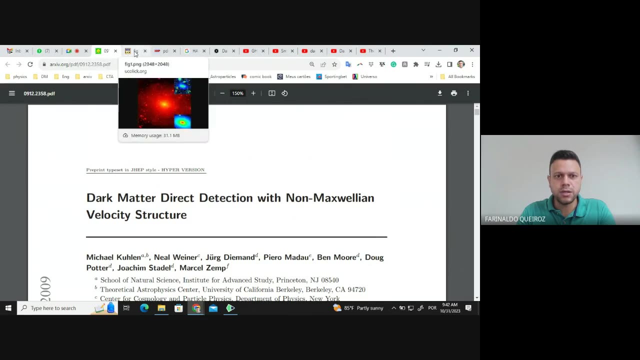 simple numerical simulations of galaxy dark matter structure. so now i'm gonna show you the picture of before i show you the results. let me share the picture of them, this one so the paper i just showed you and this paper which is on archive. they had a supplemental material. 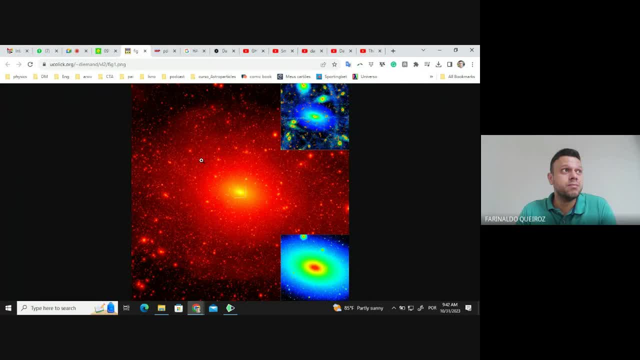 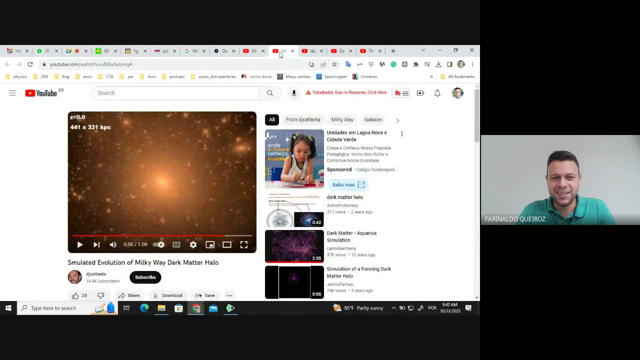 which is this figure. so that's the figure they got from the simulation. okay, it's quite nice, and i was searching if they had a video for that simulation. they don't, or maybe they didn't make it public, okay, so nobody can you know? steal that data or something. 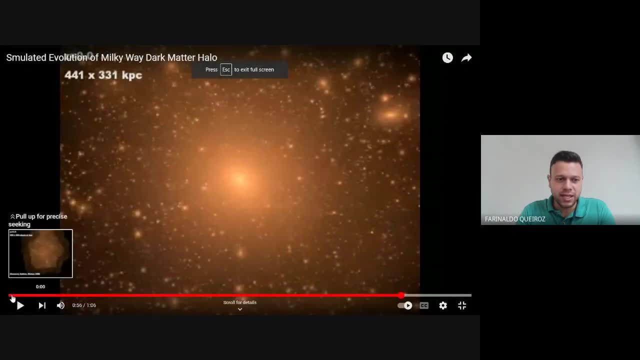 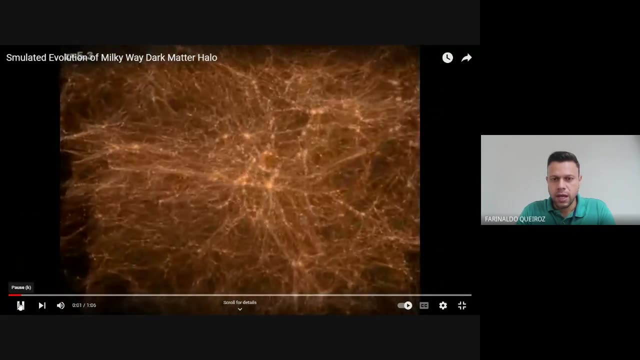 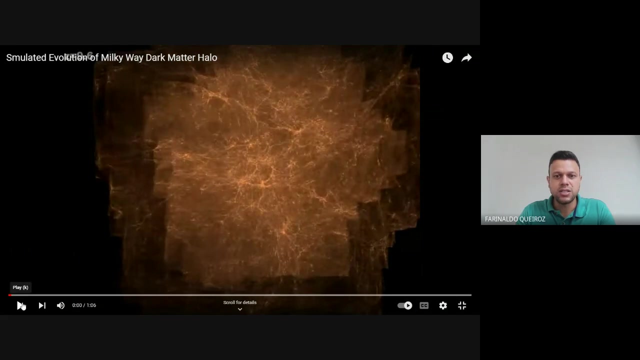 and, however, i'm going to show you something that means the same thing at the end of the day. so this is a dark matter simulation. so they, so every single point of light you see, is sort of a solar mass like dark metal particle, every single point of light. so it's like a galaxy with 10 to 14 solar masses, which is our. 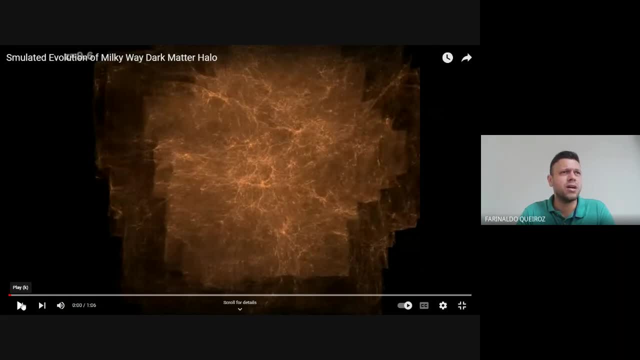 nuclear weight our liquid has into 30, 15, 10 to 12. i don't remember now the number, exact number: 10 to 12 solar masses. so there are 10 to 12 dark metal particles of a size of a solar of the sun. 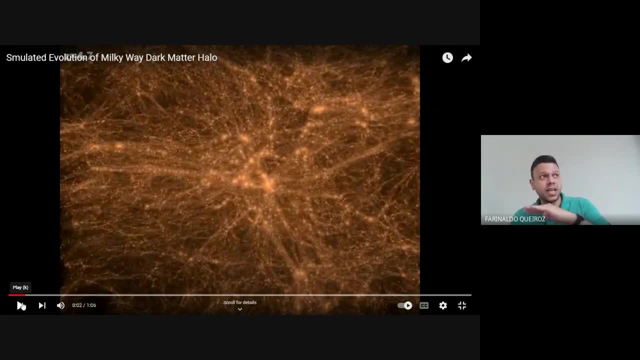 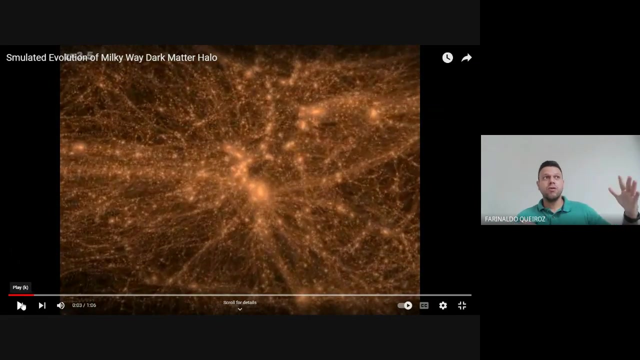 and then then they assume that just gravity takes place and there is a perturbation, the density consistent with the one inferred from cmd, and let it grow. and the point is, let it grow, and then they see the final result. they see the final result compared with spectroscopy measurements of the cmd, of the 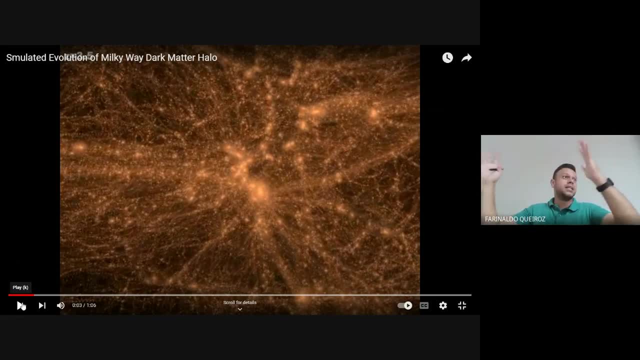 microwave. you compare the two photos and just from the two photos they do a statistical analysis to see how how close they are to each other and how long it took for the simulation to reproduce that microwave. the time it takes matches the age of the microwave. obviously they don't like to take millions of years, right, but it's somehow normalized it. 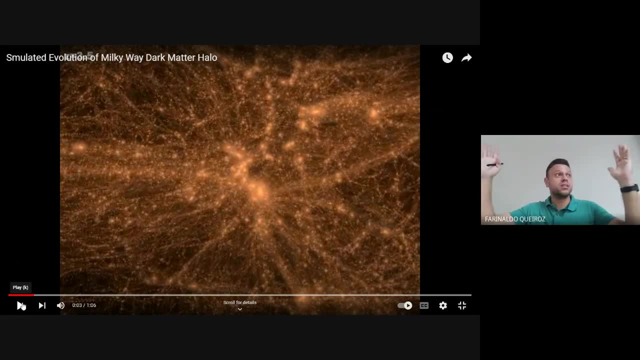 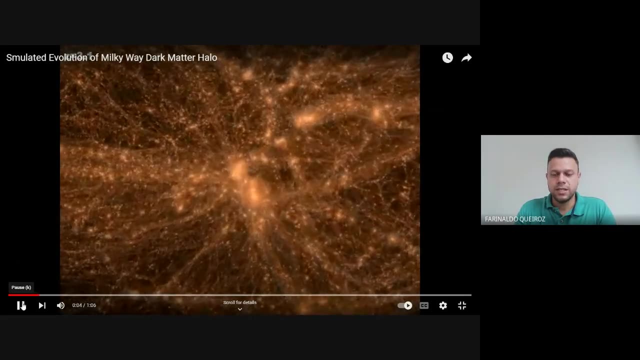 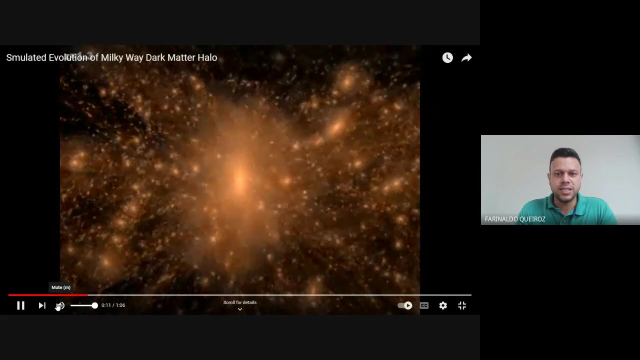 matches the age of the microwave. and the two figures, two plots. they agree with each other, just letting dark matter take place. and here's like the, the they condense, that will turn out to be the center of our galaxy. as you see, some of them are moving. 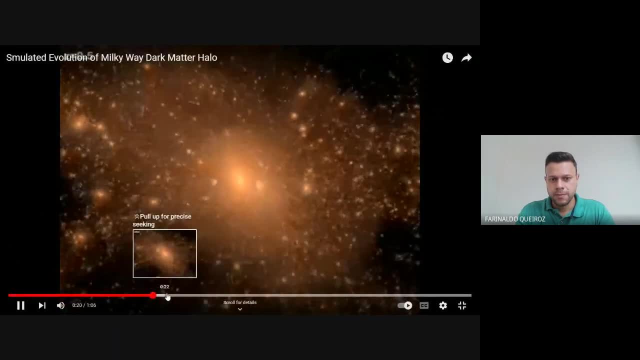 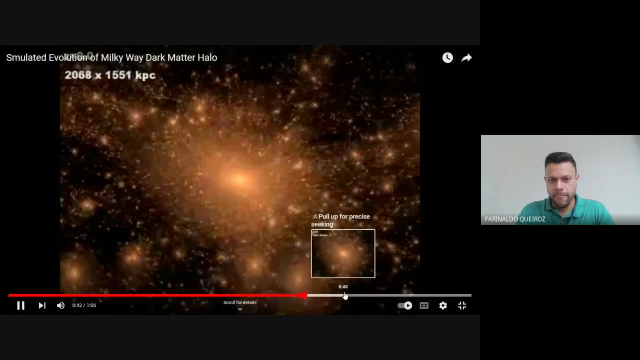 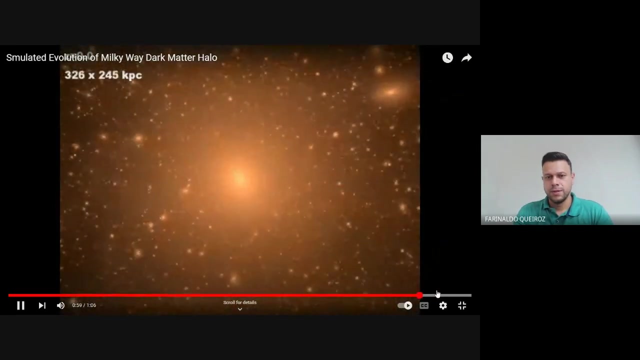 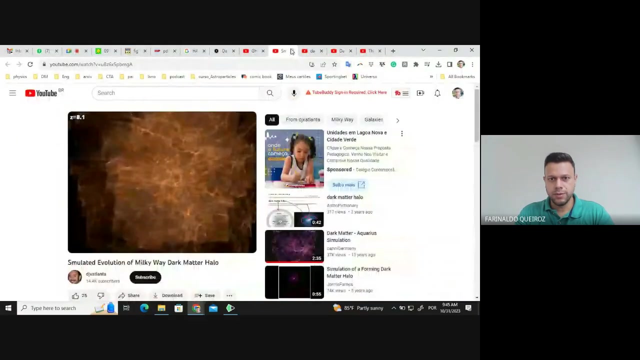 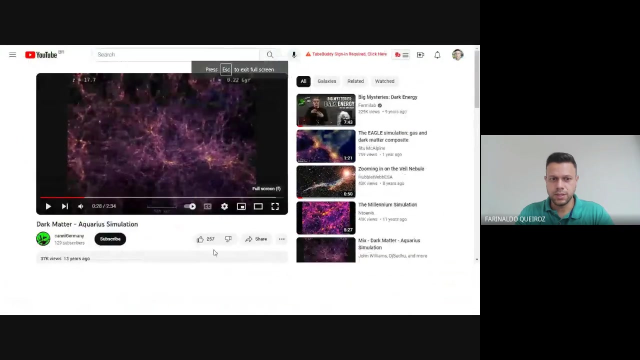 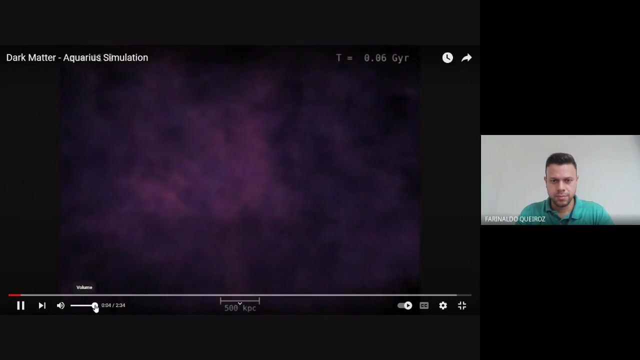 away, so let me speed up. that's the brightest, that's the center of our galaxy. let me show you another one. this one is this. this one is old, but it's the one that i saw on youtube, so it's a smooth halo. see, it started with a smooth halo. 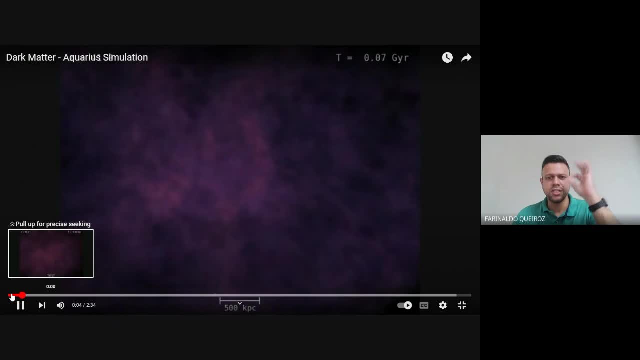 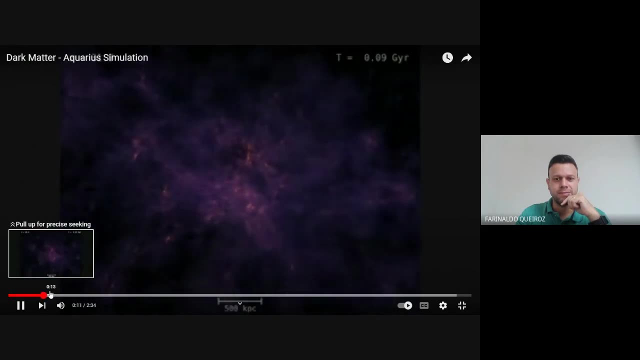 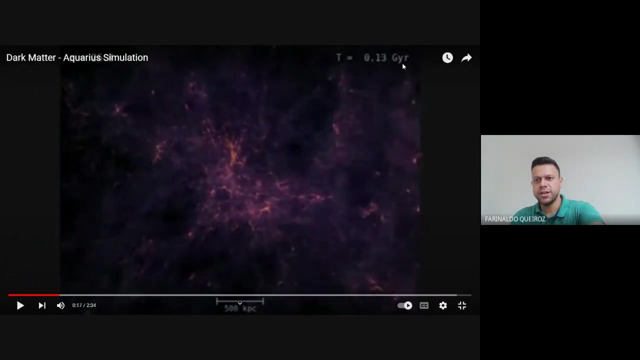 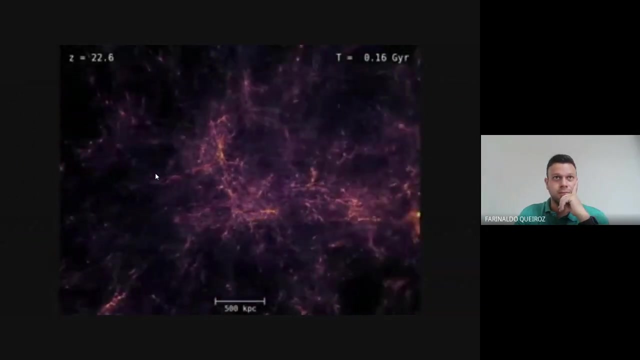 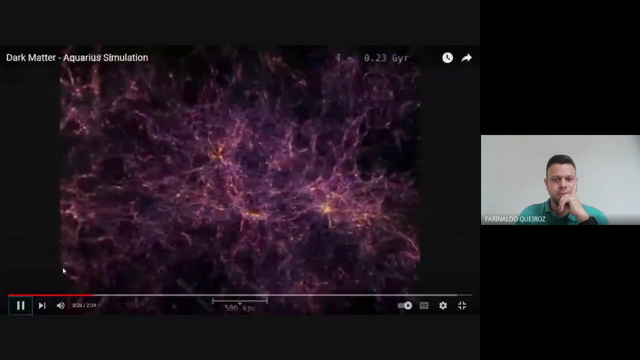 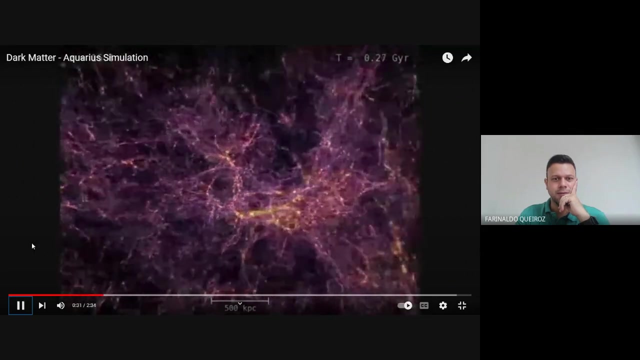 you don't see it like uniform in the beginning, but the commodities are very small and they start clumping. and that's the time here in giga years. see on the top. look at this side. that's in 500 kiloparsecs. so this one is not from one galaxy, because 500. 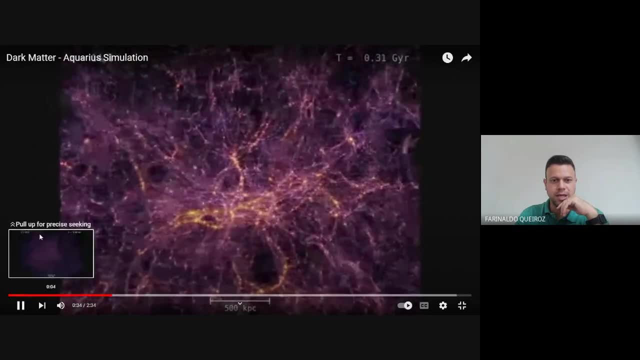 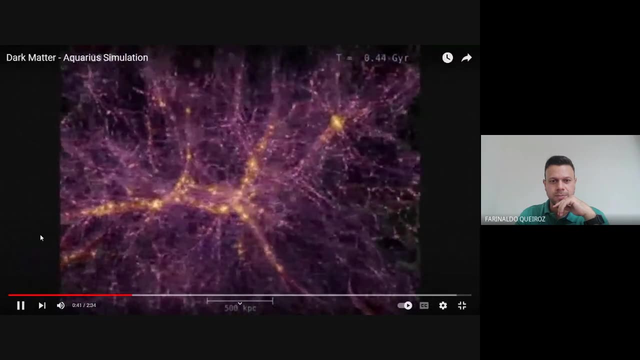 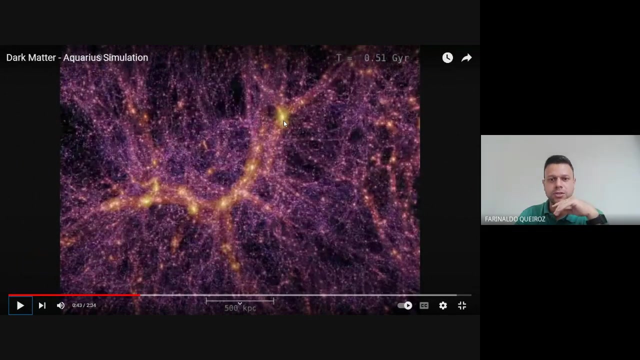 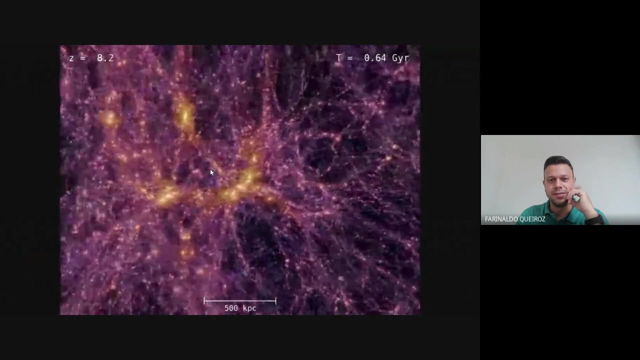 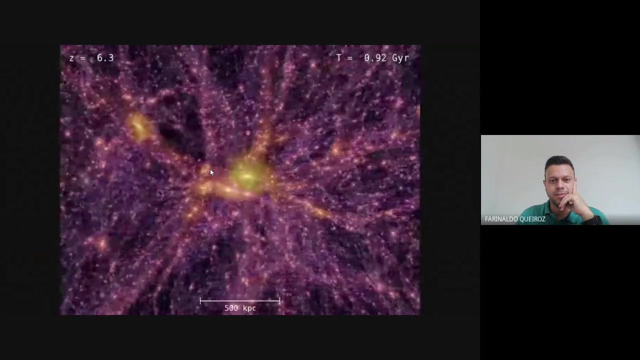 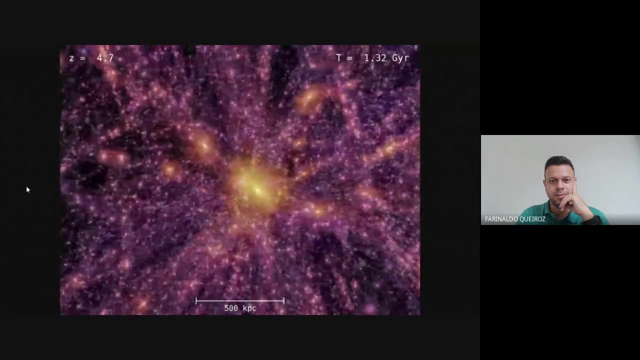 in kiloparsecs isn't right now. in every dark spot, well, very bright spot, you see, is a galaxy. basically three correct tracks and i've got three redichtet because i can see that the whole galaxy stays in it. so i saw him getting z WRONG. 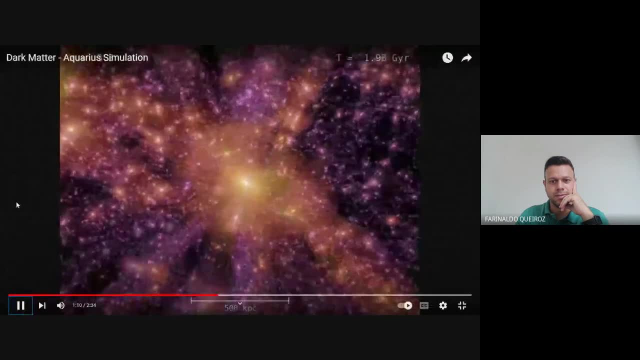 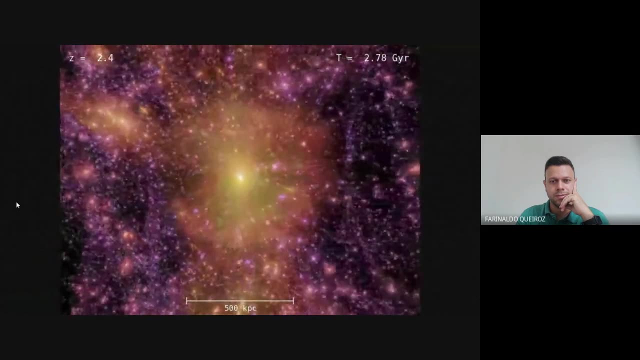 he's sleeping and i'm saying: are these gays? yeah, it's hale, wallace. he's sleeping but he's not breathing. so maybe one of the roses say: the power's going to die. what that just meant was what? now? hey, i'm yearning for an artist. 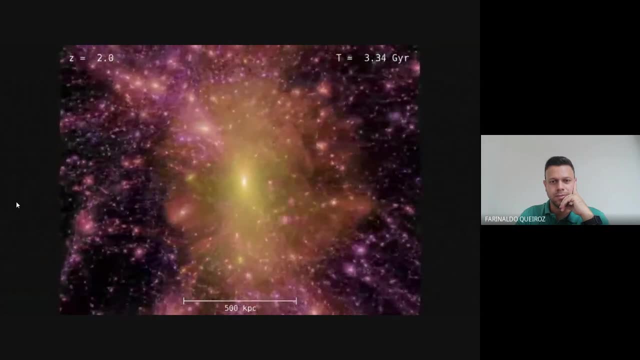 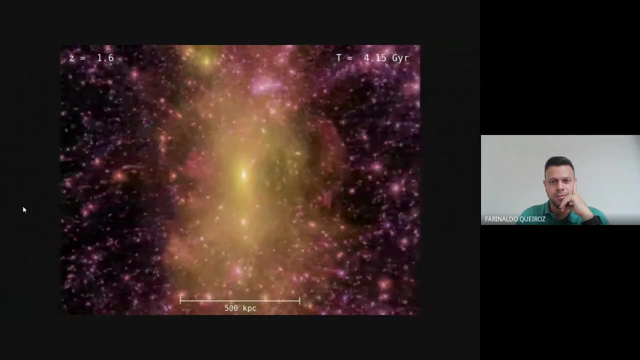 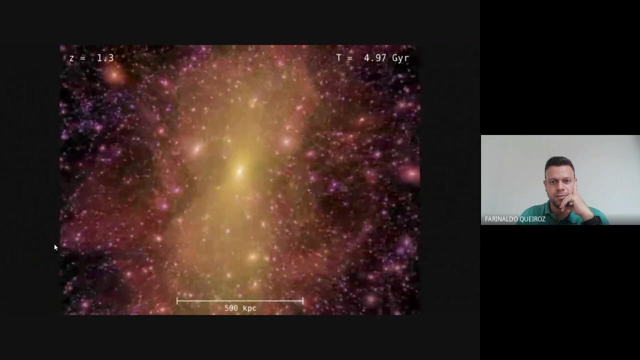 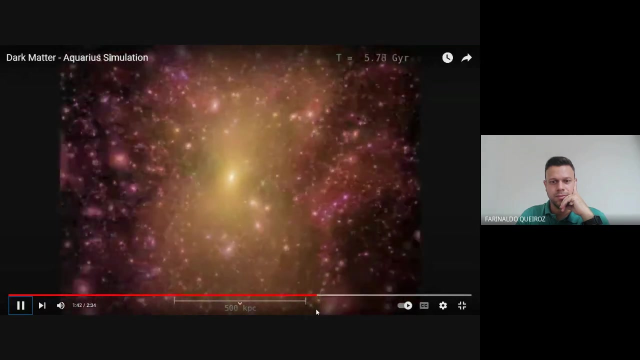 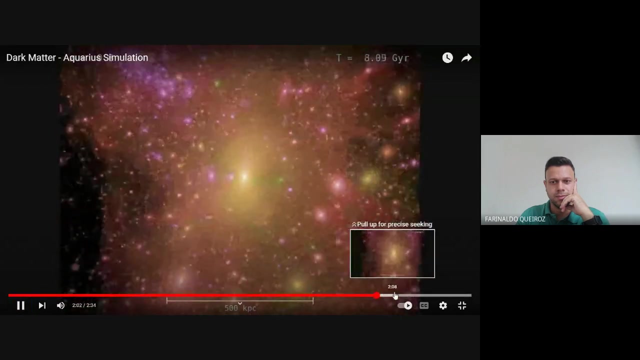 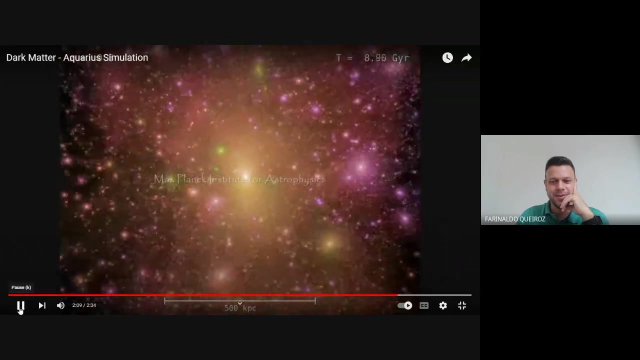 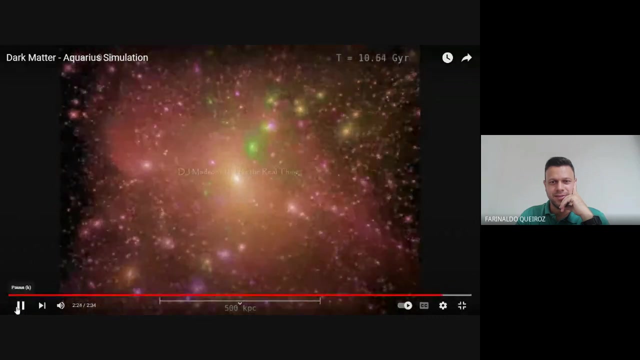 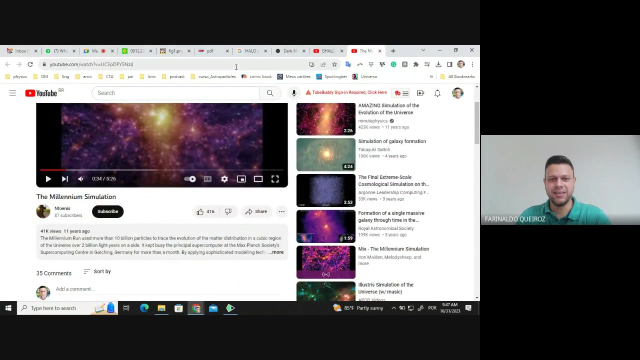 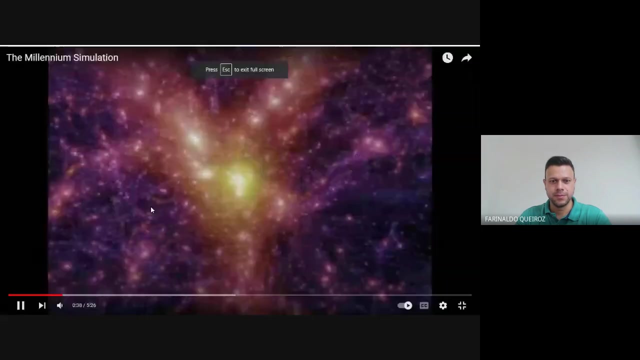 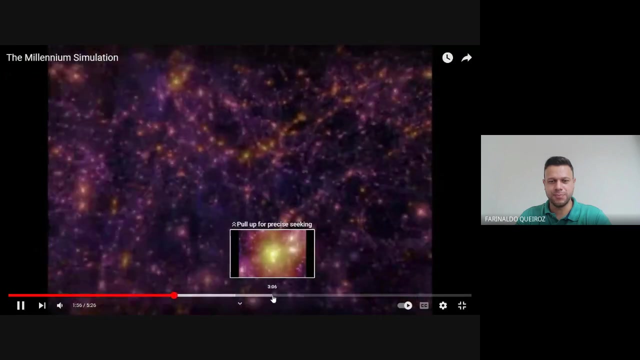 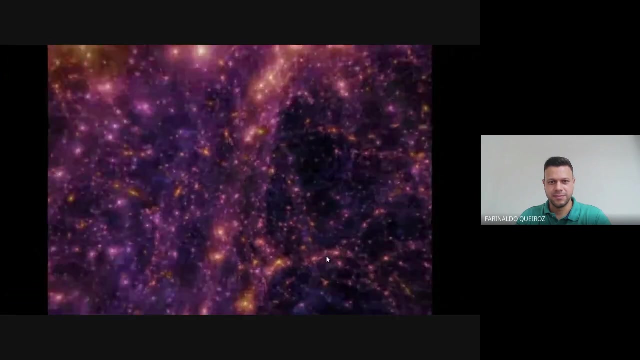 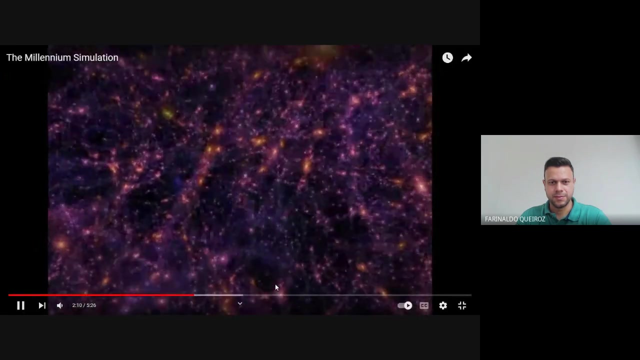 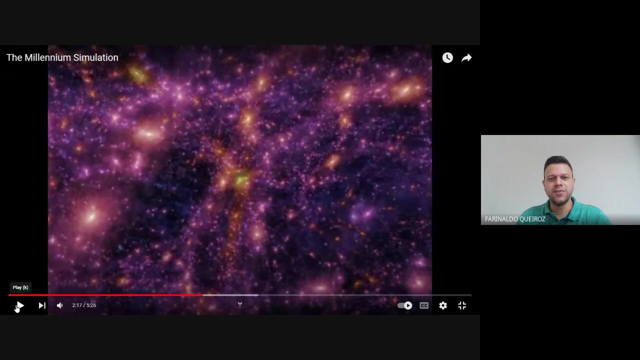 let me give you that ilah. Thank you. So this is just a simulation. Okay, I got this now. This millennium was the famous one so far, Thank you. Can we travel to the next slide? You know, what's funny is that you saw these filaments of structures, right? 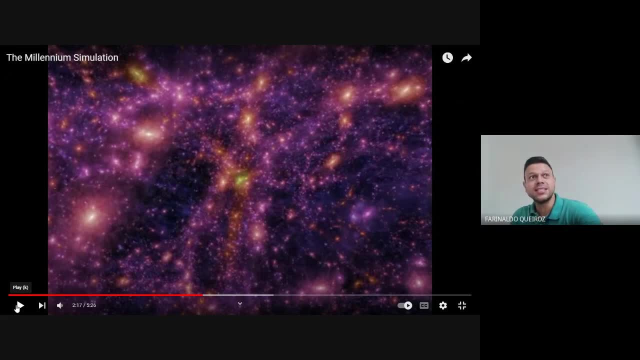 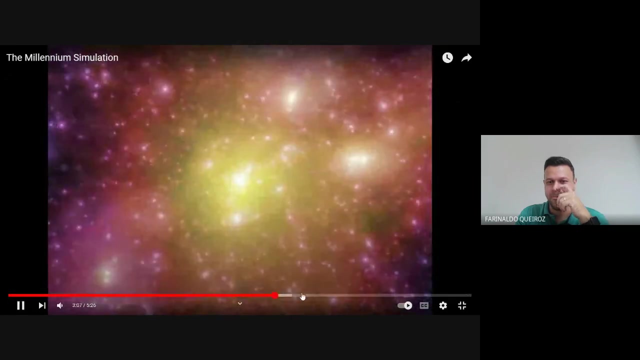 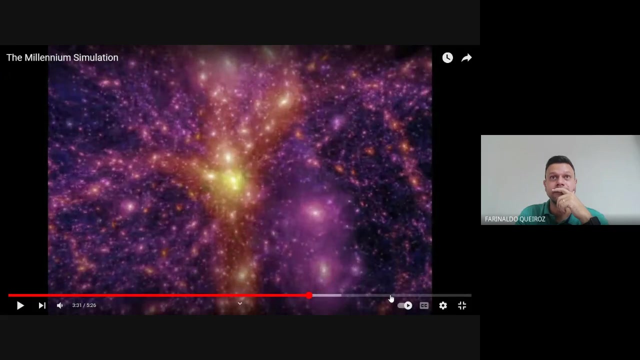 Would you write? And the size of these filaments are the size of the filaments we observe in the universe today using a simulation. and it's pretty amazing When I see this. they look like neural networks and stuff like that Big record gravity right. 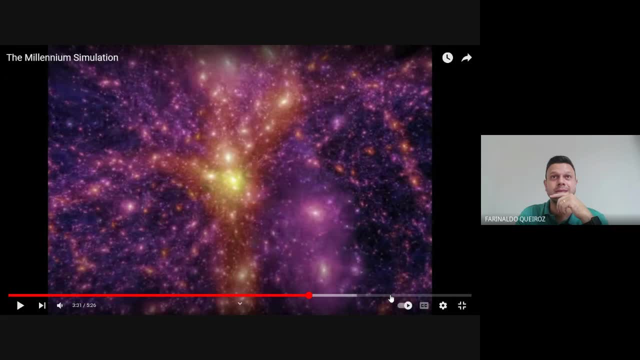 Why don't they? Because at some point the nonlinear regime kicks in. It's not linear, It's nonlinear, So you cannot just assume they'll be a spherical thing and so on. We don't know, So predict the formation of plants is highly non-trivial. 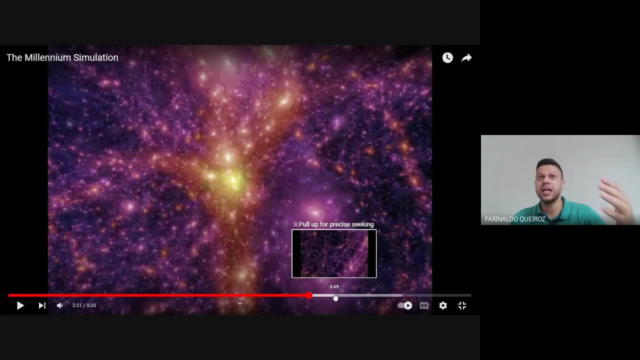 Sorry To predict how is the formation of a planet is non-trivial because this scale is too small. A very large scale. the universe is isotropic and homogeneous, But as you decrease the scale, then the nonlinearity becomes so important. 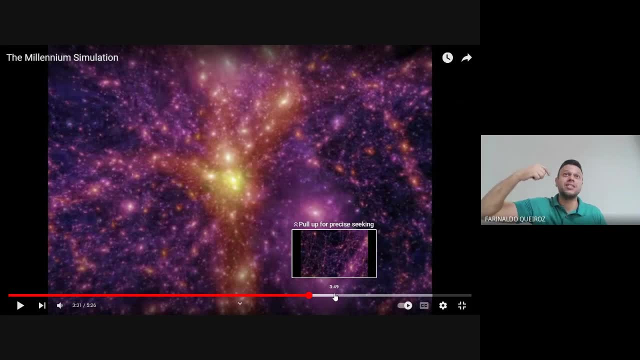 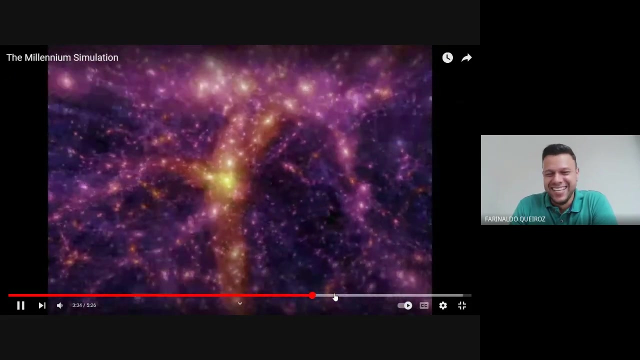 That's how you can scale down and take into account all these nonlinear facts at low scales. We don't have the computing power and knowledge to do so. I mean, why do the plants look like spheres? I'm not the one to answer that. 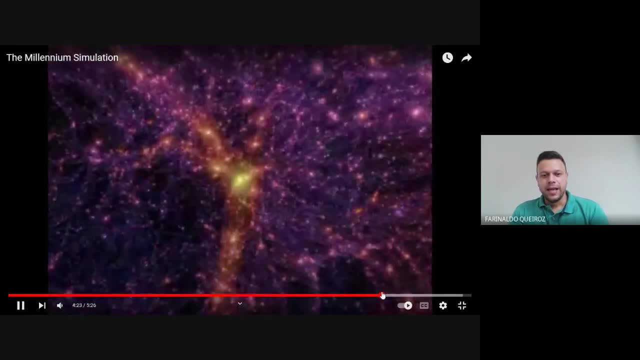 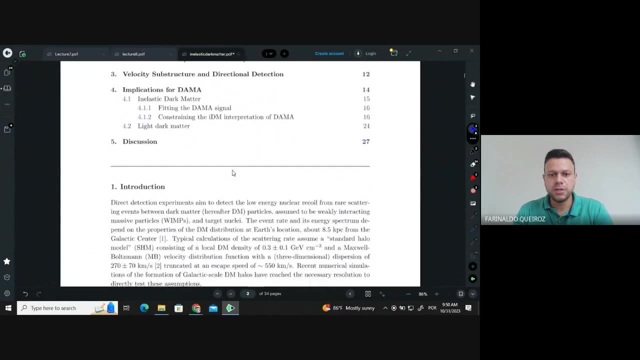 Anyway. so what I want to show you is that these cosmological simulations show that the dark matter distribution should be closer to Maxwell-Boltzmann. Now I'm going to show you the plot they have. So that's a very famous plot. 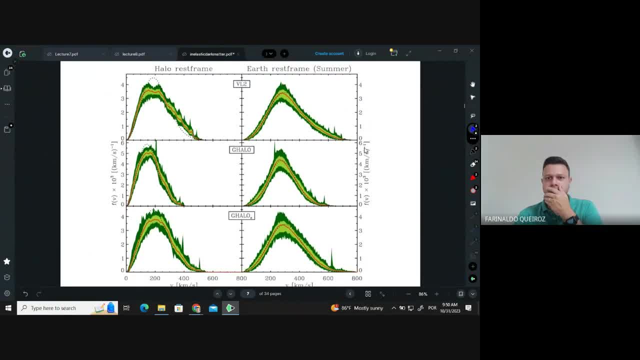 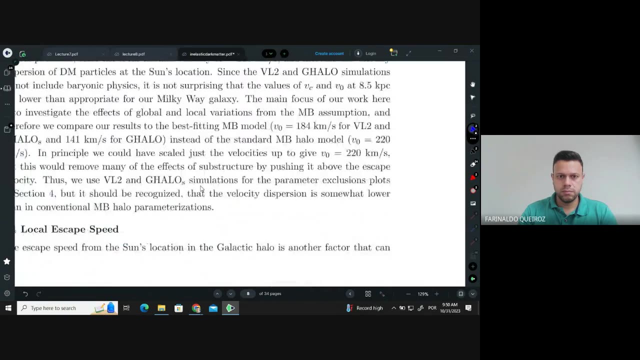 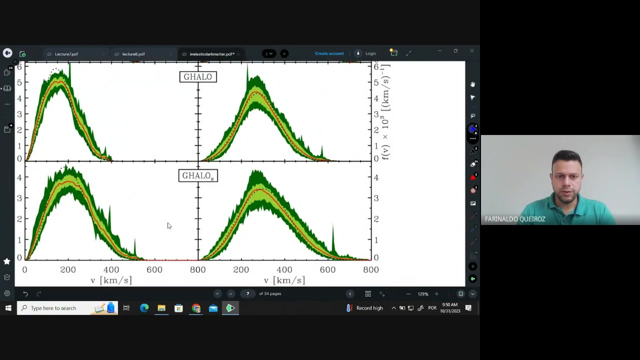 Let me show you this one So you can see, here in the head, the yellow grass frame. this is like this dotted Oops, That's 14.. Yeah, So you can see this one. for instance, They have different simulations called S Gallo, blah, blah, blah, VL2.. 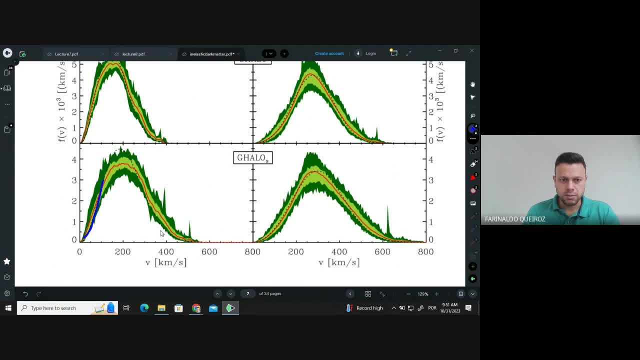 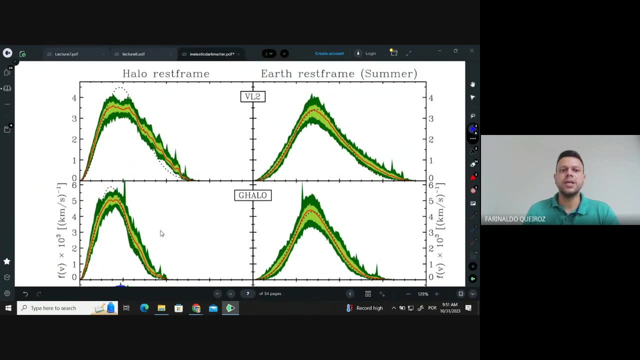 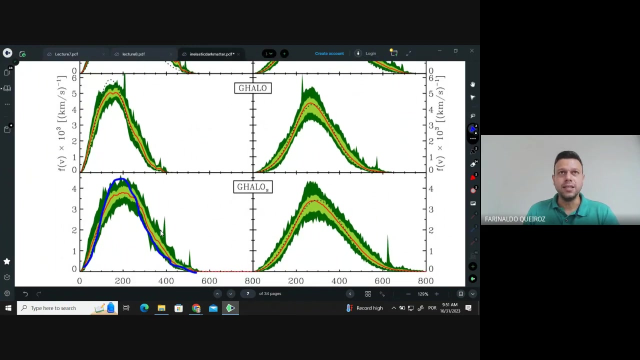 The dotted one would be the Maxwell-Boltzmann See. It has a reasonable agreement with this simulation. So you see here and this one here. But what they're showing is the simulation showing that in some cases the Maxwell-Boltzmann distribution seems to be too spiky compared to what we actually see. 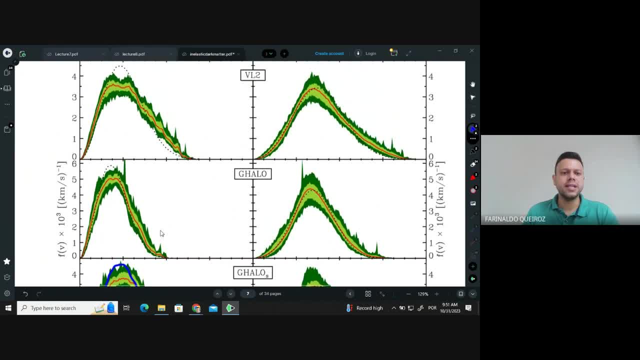 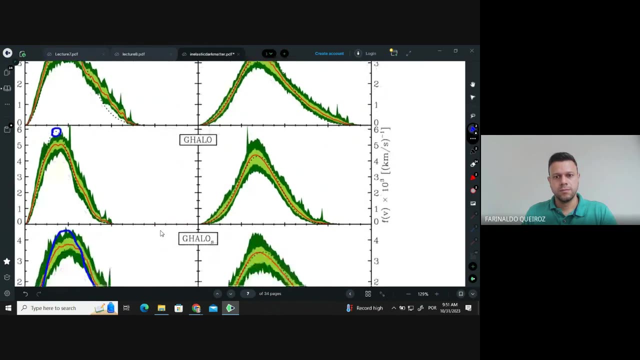 Okay, So maybe we are overestimating the highest velocity We have, So we have a different velocity than what we have for Maxwell-Boltzmann, compared to what real data, mock data would look like. What was the data from the HALO right? 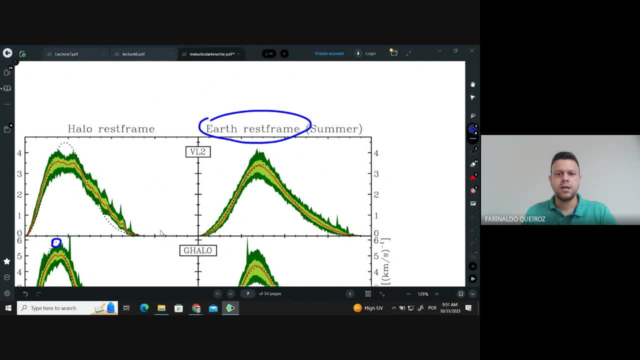 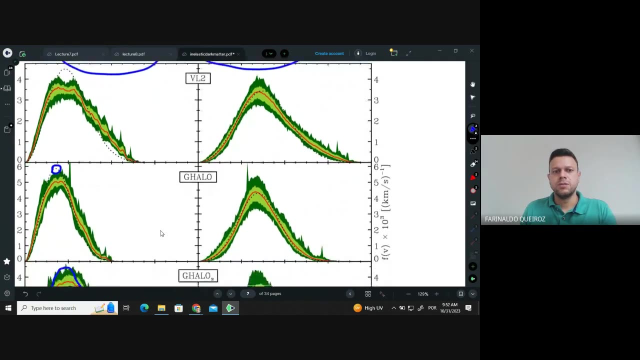 No, this one is just: you are just changing the frame- Earth frame and HALO frame- So it would be from the sun location. Then we have a different velocity towards the HALO right, So it's smoother When you're at the Earth frame. 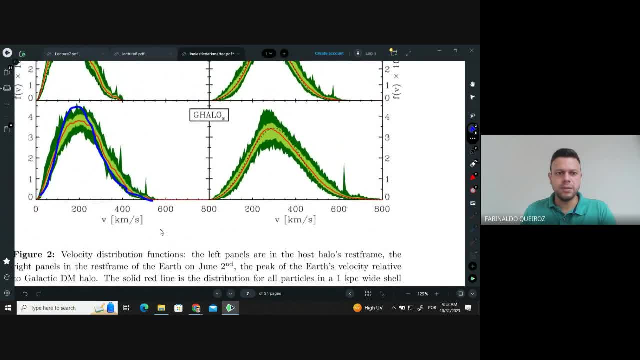 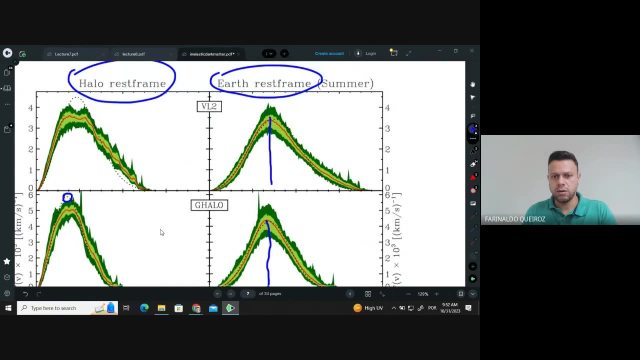 Anyway, and then they all point to a velocity. You see, the most likely velocity is around 200-something, 200-something. For instance, at the sun location it's around 250, 250.. Basically also close to 250, 240, something like that. 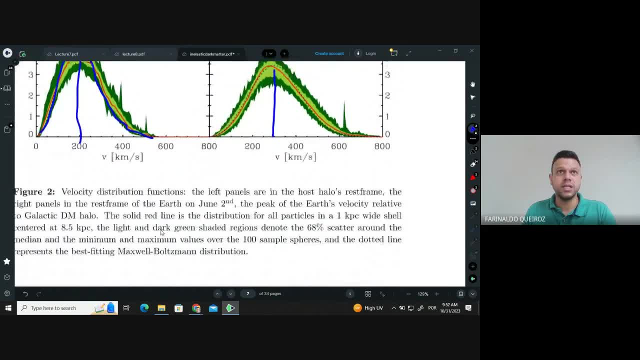 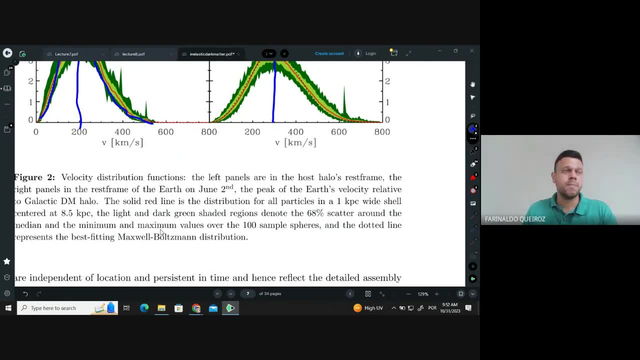 So that's the most The average velocity would be. It's around this: When you take the average velocity of integrating the Maxwell-Boltzmann, you get 200-something, 250.. Integrating from Vmin to Vscape. 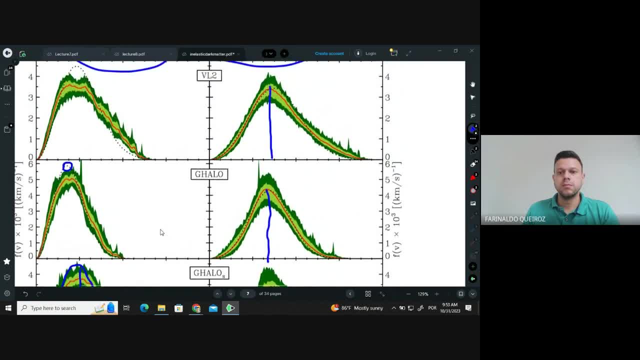 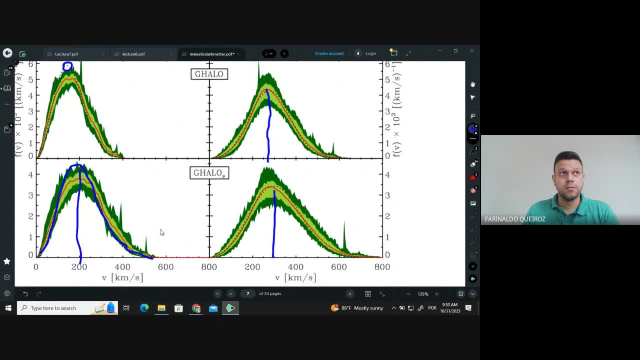 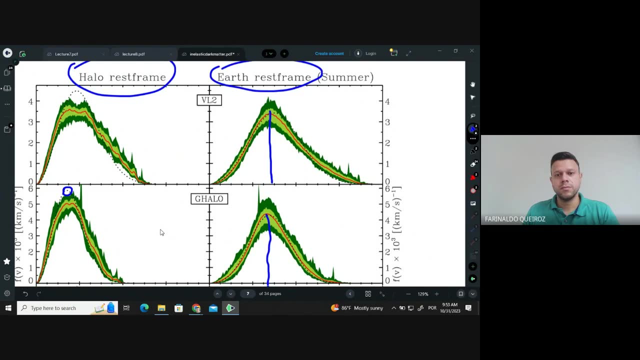 What, What, What Mm-hmm? Right there. So This time it's Here. so Yeah, Mm-hmm. Yeah, So the Maxwell-Boltzmann has a very good agreement. See, Since we have. 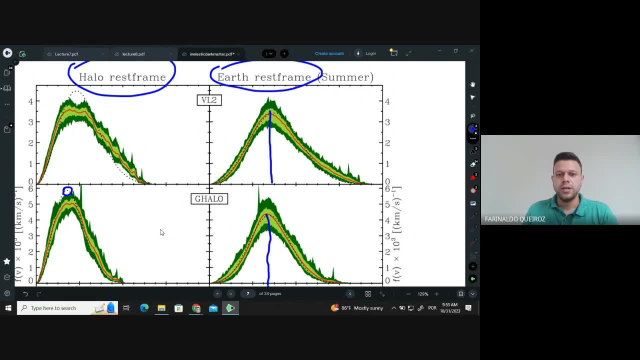 The detectors are here. What he's saying is that the detectors are here. So, as the detectors are here and the Maxwell-Boltzmann fits pretty well what the mock data tells us, right? So, And then there's another thing Why they were discussing this. 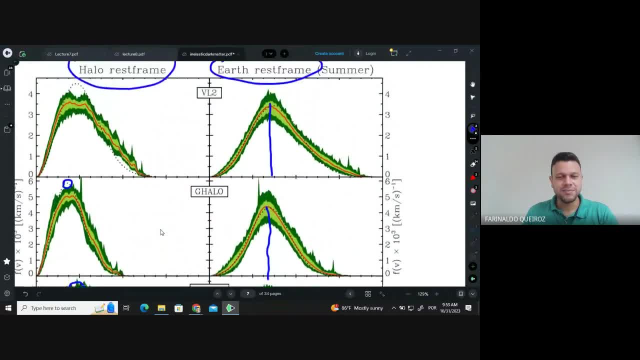 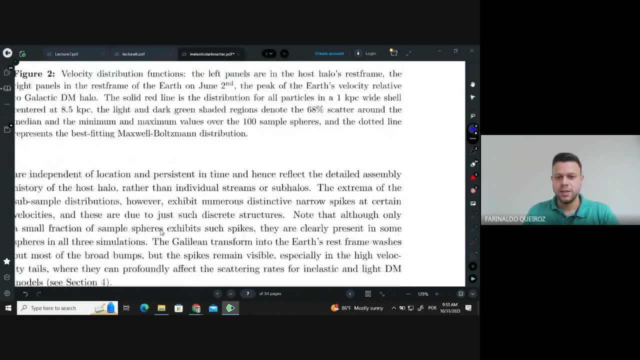 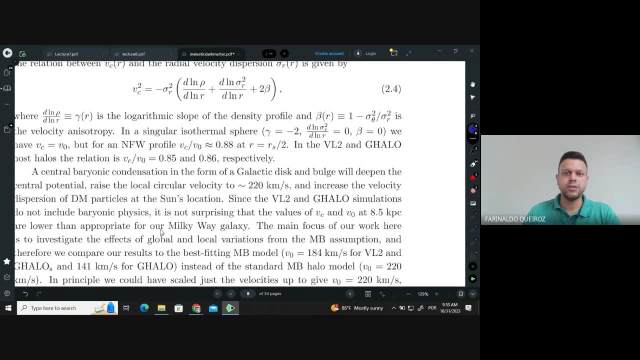 Well, they were not interested in this. actually, They were interested in trying to address something called inelastic dark matter, Which is something that I'm gonna explain now, So let me go to. So here they just relate how the number density, the halo profile, is related to the velocity. 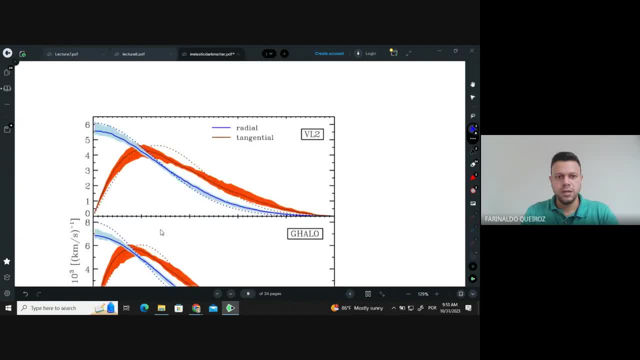 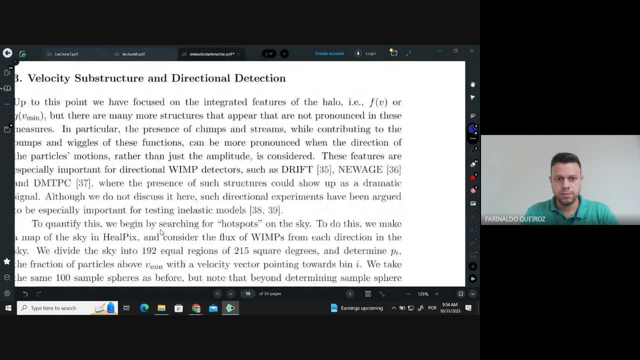 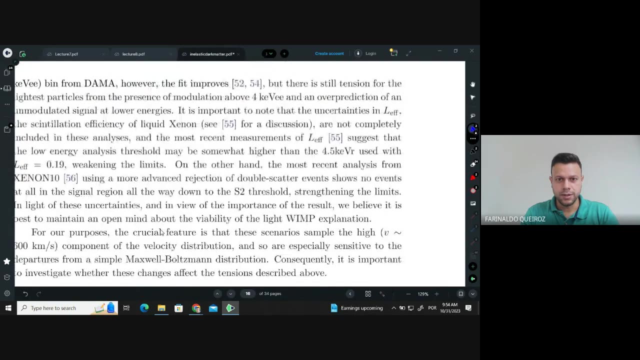 And they compute the whole thing. But let me discuss something else. Hold on Implications for the Yeah, So let me discuss. Let me go back to figure Slide seven, Cause we're seeing direct detection. The way it goes is the following: 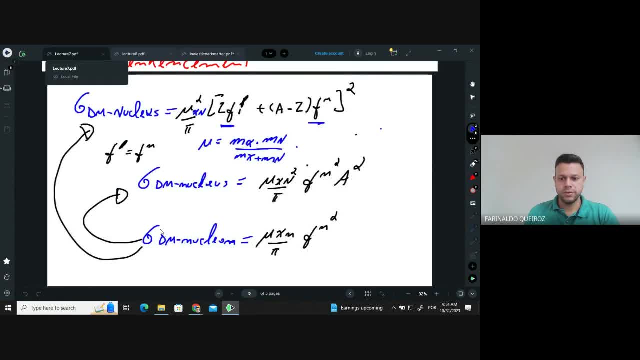 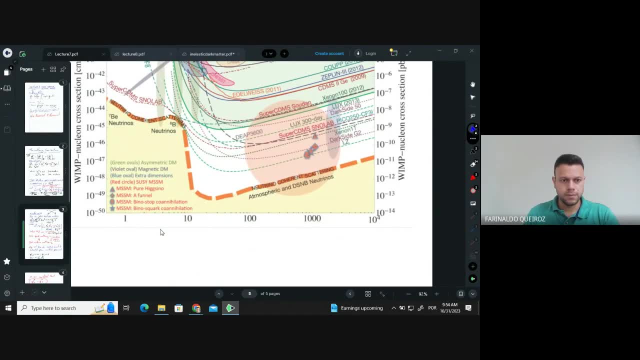 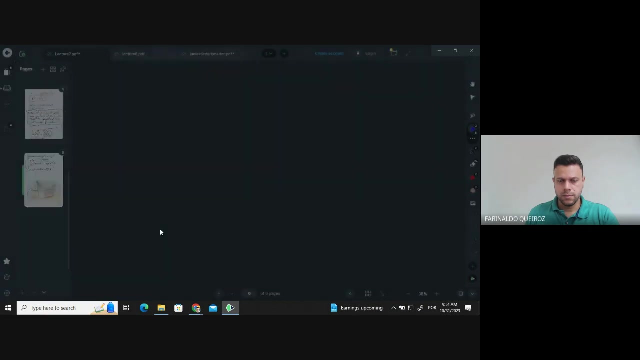 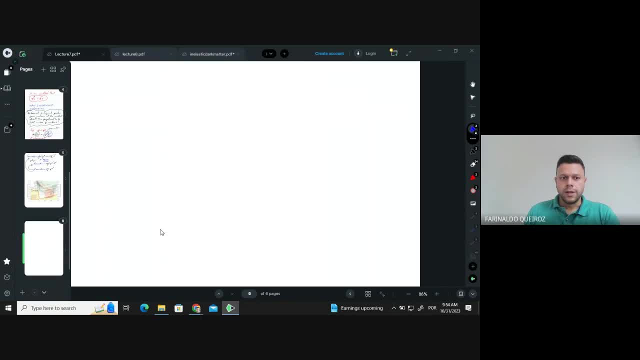 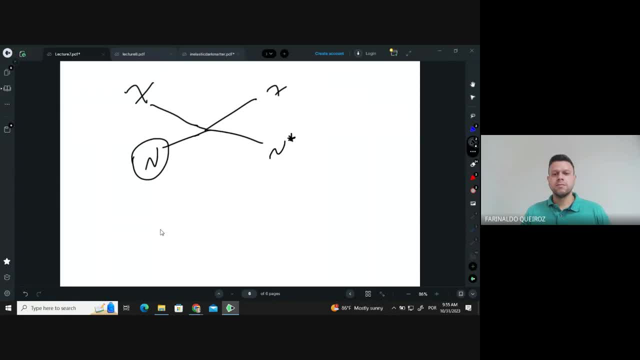 i have an energy threshold, right, that's what it means, energy threshold. now let's, let's think of the following. so the detector is still the same, the target is still the same, comes the same dark middle particle here, but in my model, my part of this model, this chi n chi n star, does not exist. 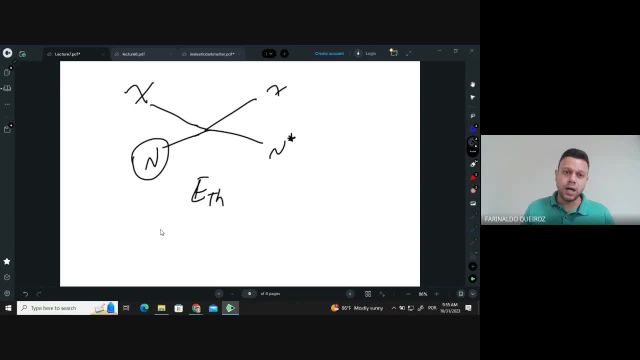 in my model. what i have is chi 1, then chi 2. i have two dark particles and i'm gonna assume that chi 2 is minus chi 1 is equal delta, so n chi. chi 2 is heavier than chi 1. now pay attention to this in order for this scattering to take place. 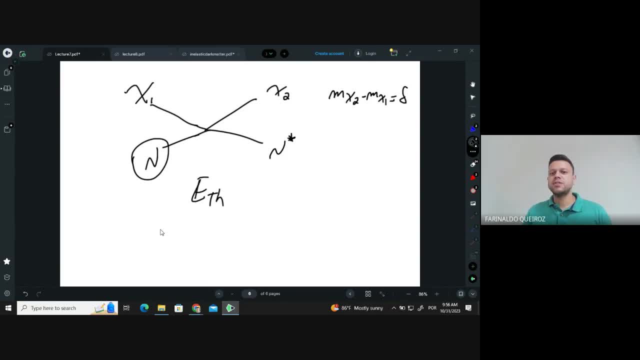 okay, in order for this scattering to take place. this seems to be not dramatically possible, right, because chi chi 2 is larger than chi 1. okay, but actually it can happen if m chi 2, for instance, i come with a chi 2, comes here, kicks in, and, and then the velocity. 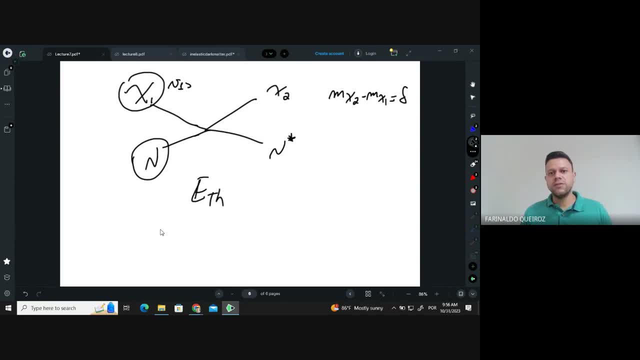 of chi 1 turns out to be larger than the velocity of chi 2, okay to compensate, because it's not just the mass as the energy right, the energy has to be conserved, that's fine. but as long as v1 is larger than v2, then it's okay. i compensate for the mass difference, fine. 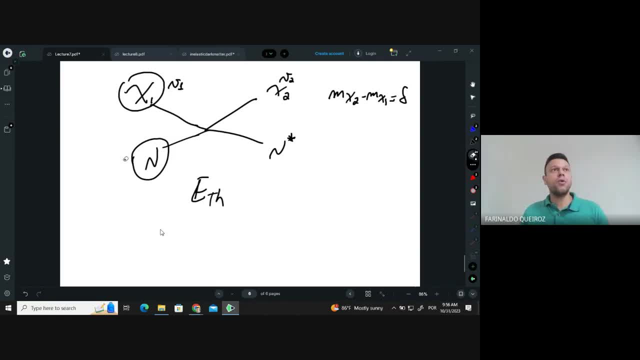 so this model, where i have chi 2 heavier than chi 1, is called inelastic dark matter has nothing to do with this. carrying being elastic as like being deep into the nucleus. what what we refer by elastic is just bump. you see the whole thing. the nucleus is a hole. 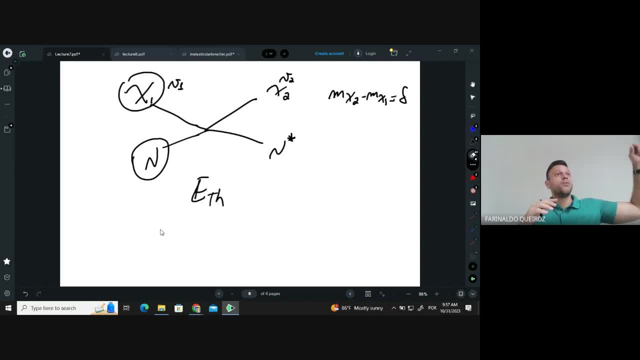 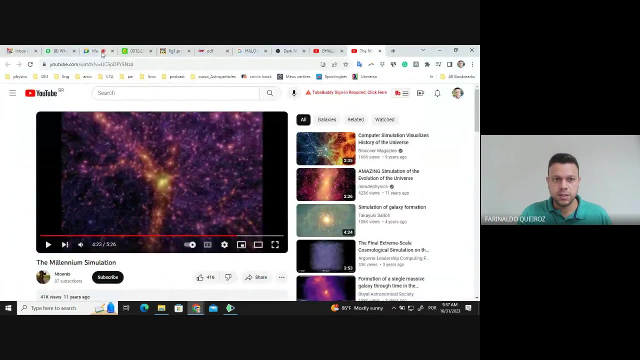 in the last is when my, my, my wavelength is too small, and then i can see the whole nucleus right inside. i see the nucleus that's called inelastic deep inelastic. scattering in the last means i see the whole thing inside. let me just close this. this is what's happening. 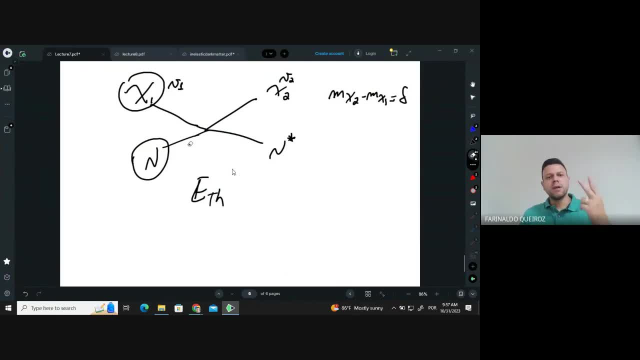 in this case, in the last dark matter we first decade, where i have two dark metal particles. one is heavier than the other. but look at this, this velocity of v1 has a maximum value. right, it cannot be anything limited by the maximum distribution. okay, so look at this. if i go to light dark metal particles very light. 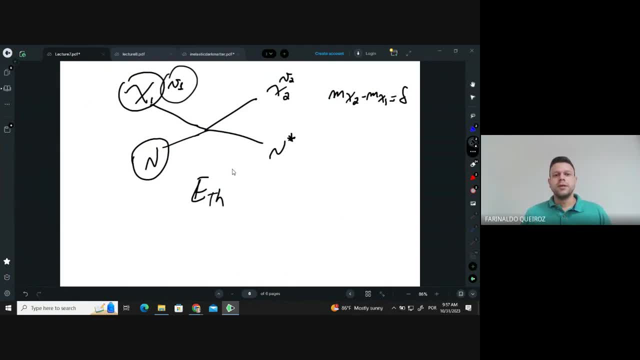 very light dark metal particles. remember if i, if the dark matter is very light, let's say 1 gv, m chi is 1 gv, and then i can see a signal. if darkness 1 gv, let's say: i'm right there, the threshold of observing this scattering, and then i can see it. if dark matter is lighter than 1 gv, i cannot. 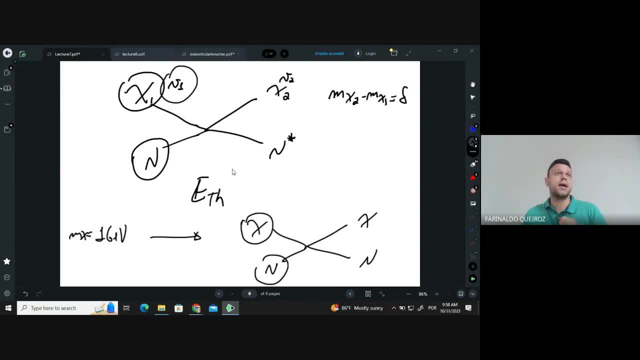 see it because the energy deposited is smaller than my energy threshold. okay, small, i can't see it. it's very hard for me to see it. there's a velocity distribution, but still very hard for me to see it. fine, then look at this. if i go to the you, then you get a different target, heavier target, the heavier target. 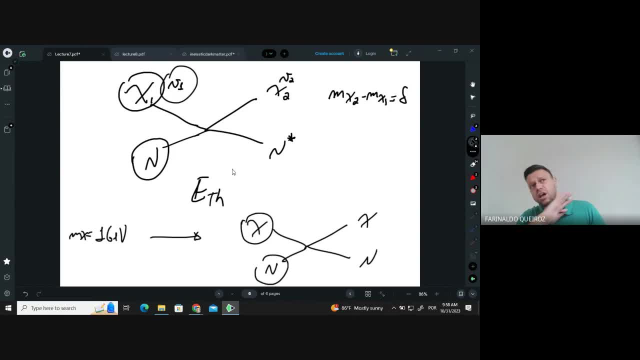 assume the energy threshold is the same. you definitely not see that signal, right? because, remember, the energy threshold is the same for those i'm assuming to be the same. simplify my, my reasoning: they have the same energy threshold. i have a light target, i see it. i have target. won't see it, because the energy department will be very small, because increase. 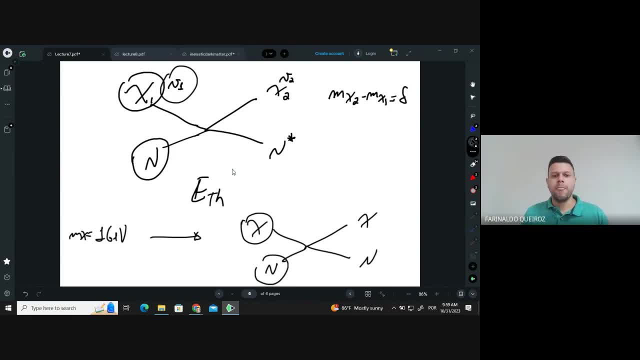 the mass make sense. fine, now let's go to this complicated case. i have chi one and chi one comes in, and chi one is light for me to see a signal that velocity of chi one has to be at the tail of the maximum distribution, because it's too light for me to see it. so only the events, the 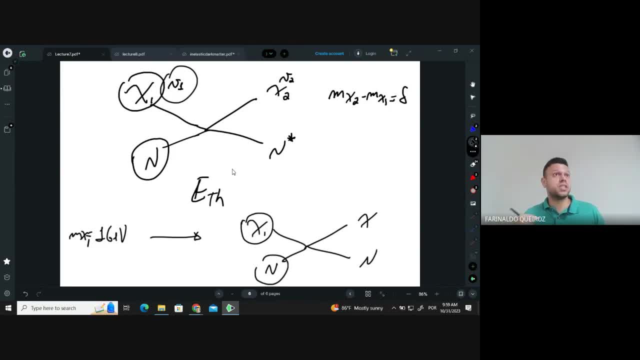 particles that are the tail of the velocity distribution will produce a signal. for me, right. and then imagine, for a target which is heavier, no way at all, they're gonna see a signal because they have a. they have a heavier target, right? so then, in order to ensure that the other detect won't see a signal, what i do is: 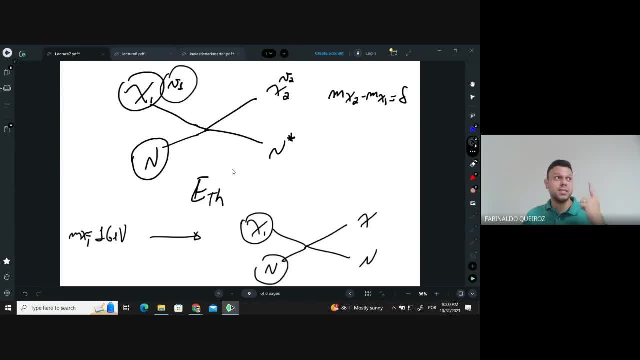 i assume that my dark metal part is not just once. this is two chi one and chi two, and then, for this event, chi one here, produce a chi two. v1 has to be larger than v2, right, right. so i have to be really at the tail of. 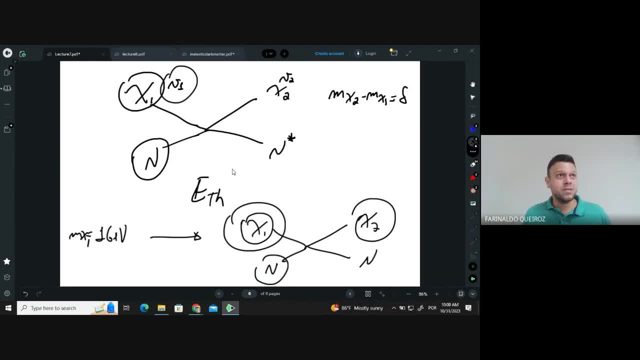 the velocity distribution to produce a signal. so i'm forcing my signal to happen at the tail of the velocity distribution and then in this case, i can make sure that a heavier target will not see a signal whatsoever, because there is no velocity larger than how it's gonna see a signal. v1. 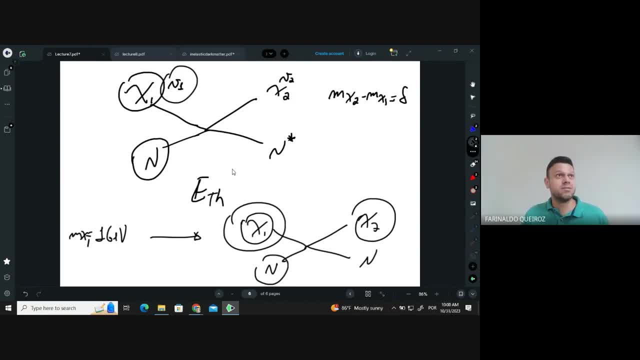 because we don't have to be really at the tail to see a signal. right, okay, obviously there is a game here between the mass and the velocity distribution and so on. but this idea of inelastic dark matter came why? this was proposed because cogent had observed a signal, and also short and even before. 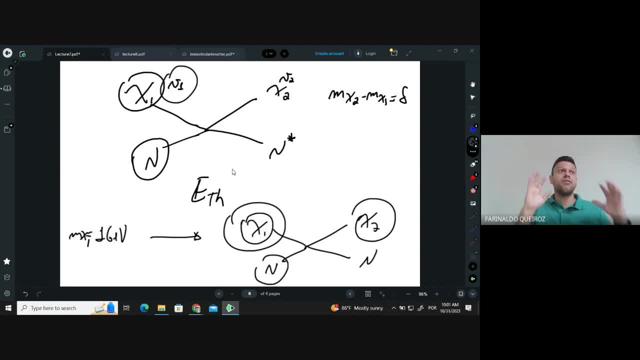 that dhamma also observed a signal which was consistent with wimps, measuring, scattering, nuclear scattering of wimps before cogent appeared and the regions where you could explain the dhamma signal and the cogent signal. they overlap and their favorite light particles and people say 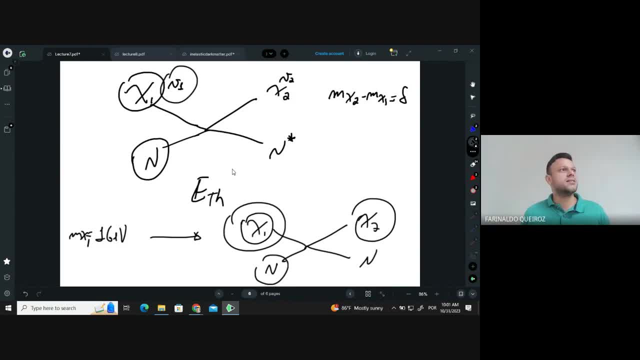 okay, but how can you explain? xenon is not seeing it. people said no, but you know, is that heavier target is a heavy attack, so you need to be at the tail. and what people said, okay, let's be now at the tail, near the tail, the velocity: i picked the velocity to be, the mass to be 1 gb. 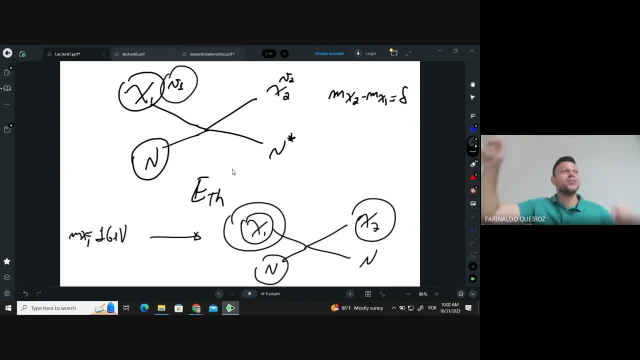 and only particles at the tail will produce a signal. if this is true, how xenon is going to see a signal then? because there's no velocity larger than the tail. so let's say: i'm at the tail, right, i'm right here, so let me draw the tail. the maximum distribution. 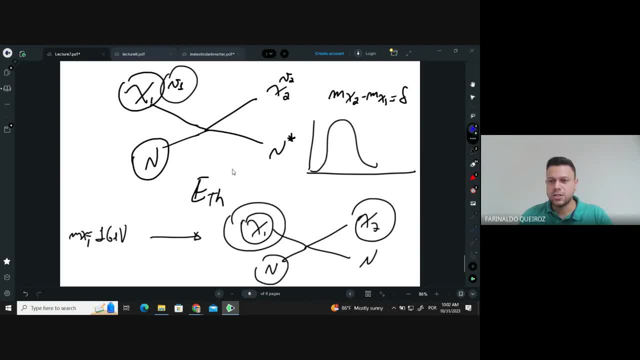 and i'm picking a mass so that just this contribution of the tail, you produce a signal. i'm right here. so this one will produce a signal that i can see. so any heavier target will not see a signal. this one will not see a signal because they would need a velocity higher than this one, because they have a heavier target. but 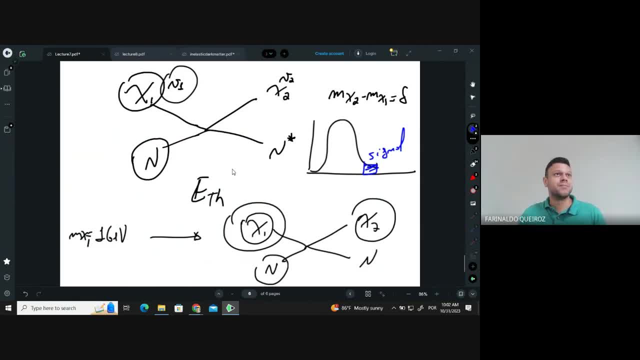 there is no velocity higher than this one, then, is a way to make sure that, while explain why, definitely, conclusively, why heavier targets have not have not seen a signal consistent with those observed at quotient and dhamma, and to make sure, even by kinematics, was this in the last dark matter? 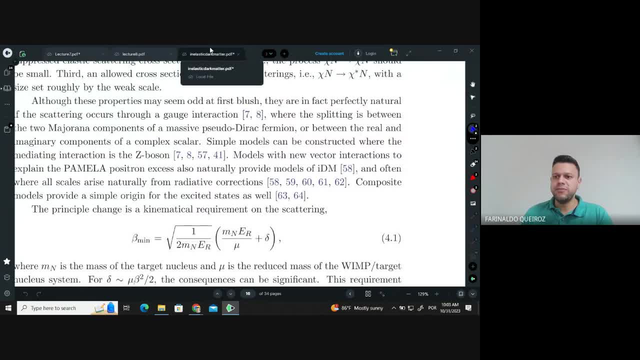 and what i'm going to show you here is the very minimum velocity you need to produce a signal. so you need the minimum velocity, as usual, but there is some delta. delta is the mass difference between chi 2 and chi 1. so, as you see here for the mass of the target, 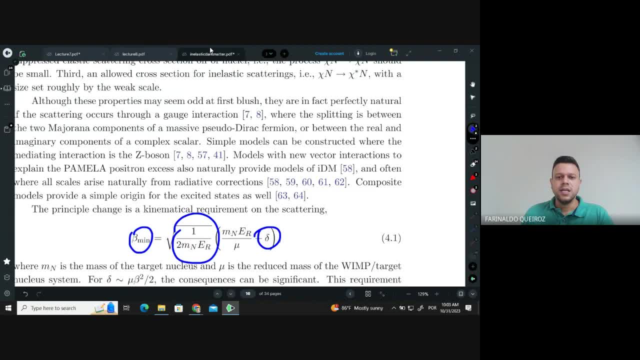 is used to reduce mass. so it means is as as soon as i increase delta, increase the mass difference between chi 2 and chi 1, the larger the velocity i need for v1. v1 has to be larger and larger. just look at the figure here. 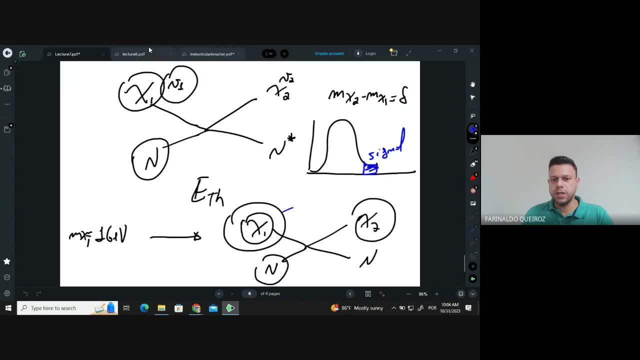 this one. so for this guy to produce this one, v1 has to be larger than v2, and as i increase the mass difference, the larger will be v1. but as i increase and tune the mass difference i reach a point that v1 has to be larger than the escape velocity. so i'm just making impossible for 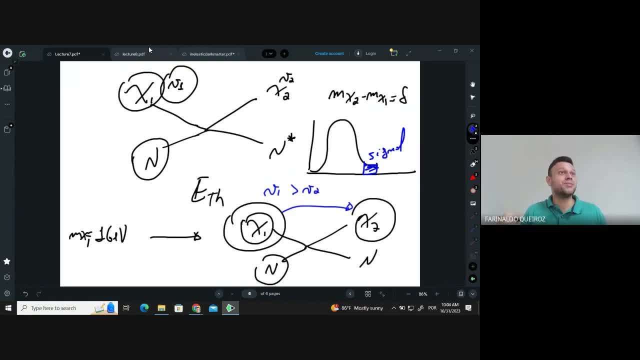 all the targets to see it, because i tuned the mass difference to be so that v1 has to be larger than the escape velocity make sense and there's a tuning. it's a fine-tuned model, okay, it's not something else. okay, that's very natural. so, but it's a tuned model. to explain why some of the 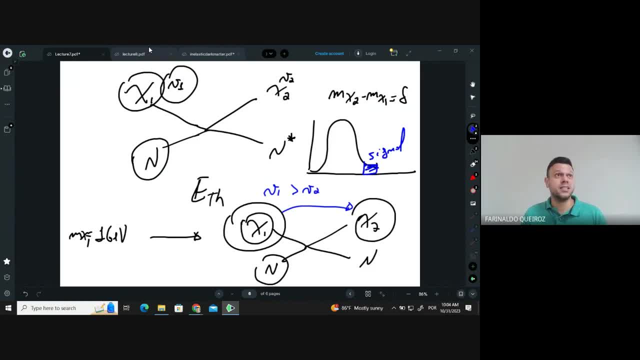 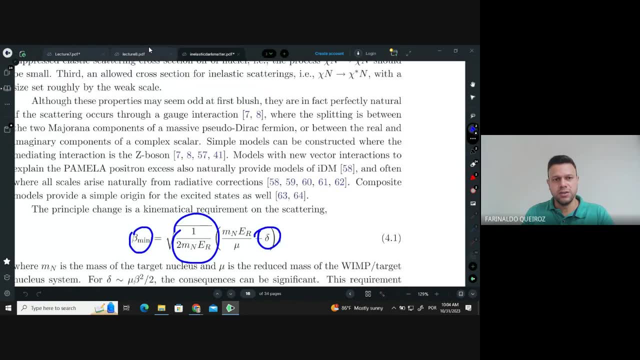 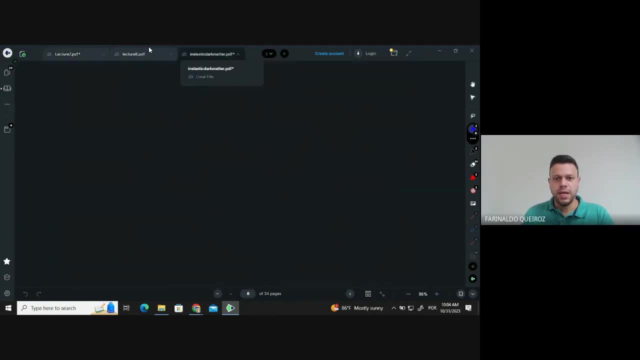 textures have not seen a signal and the others have seen the signal. so that's called an elastic dark matter- was proposed by new weiner. he's a professor from uh university of new york, new york, nyu. so that's in the last dark matter. and then let me see if i have- they have the figure here. 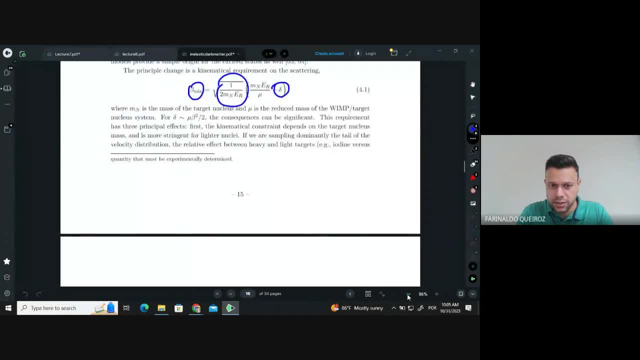 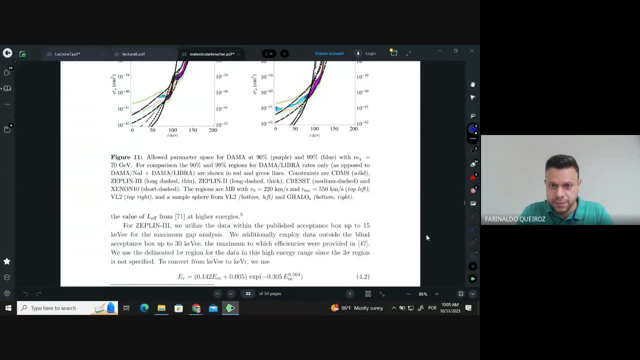 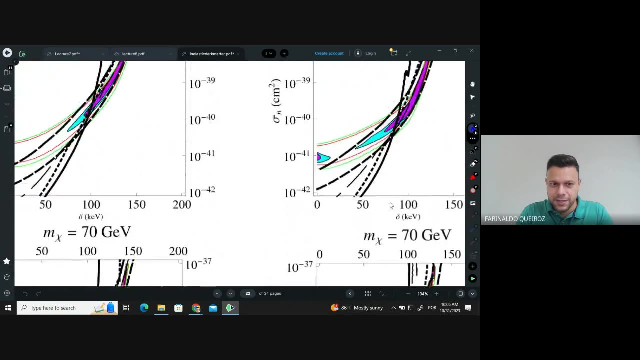 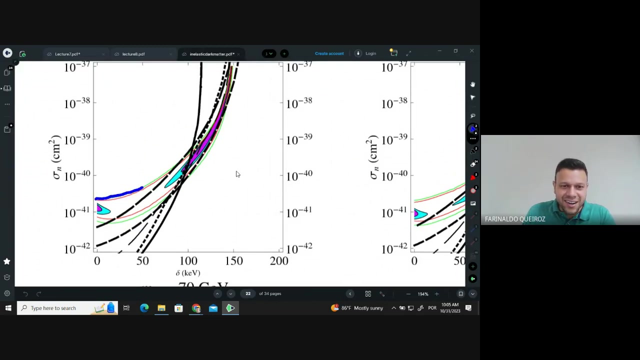 let's just show you, uh, when you take that into account, whereas if here, look how fine-tuned it is. so they change delta, the mass splitting, and now there is a region here which survives. the limit is really fine-tuned, see, because those limits are excluding everything to the the other side. 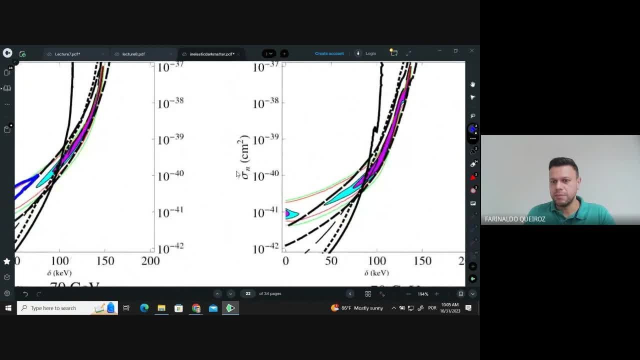 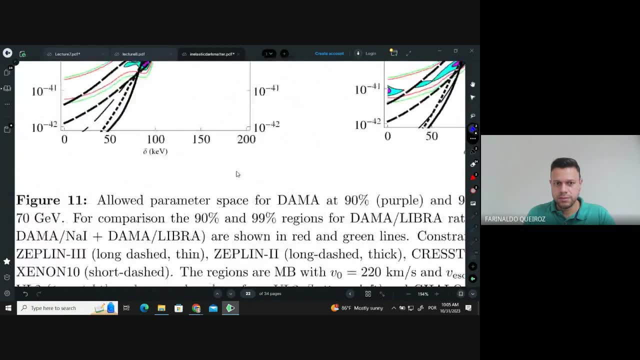 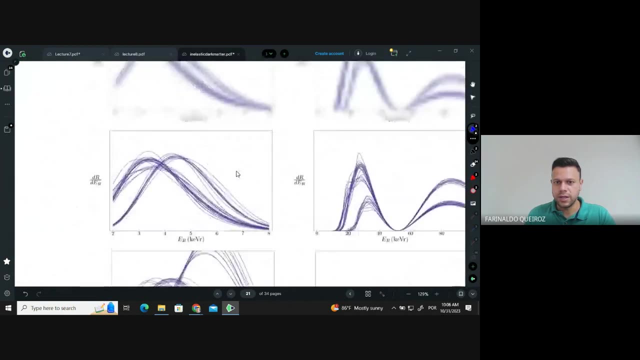 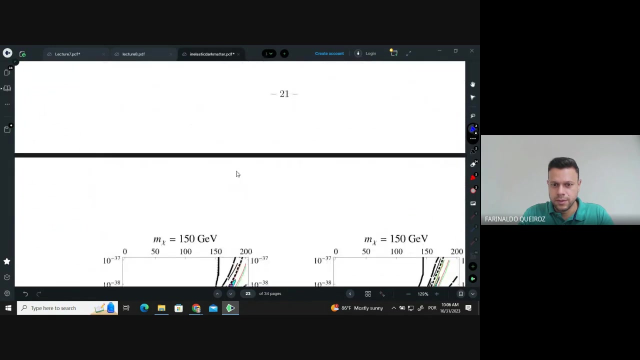 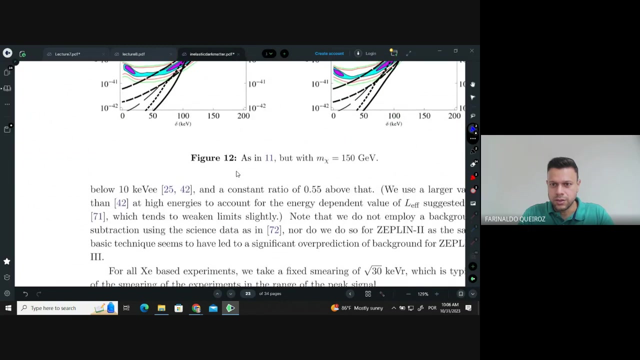 so, as you go to heavier, let me see this one, yeah, this one, this one, let me see. let me see what. there's one which is clear than this one? okay, uh, no, it's here. okay, there is more visible. yeah, so now they are picking different masses. as they increase the mass, the limits decreases. 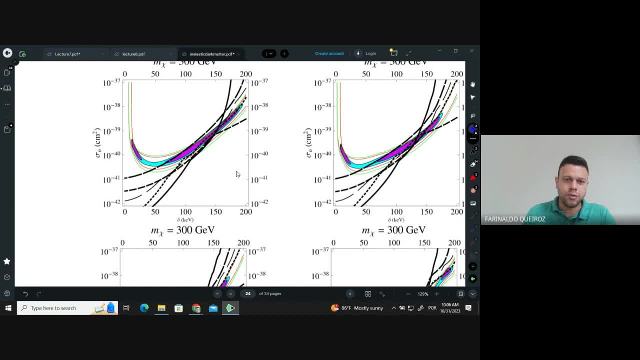 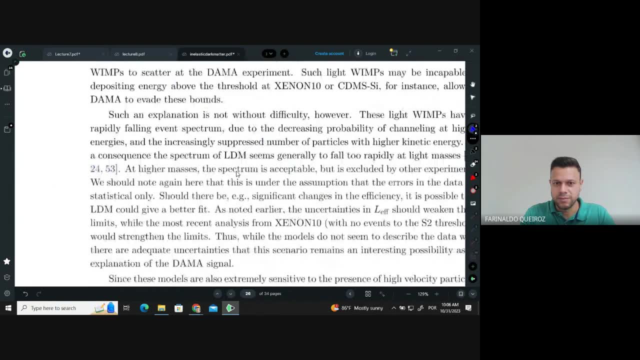 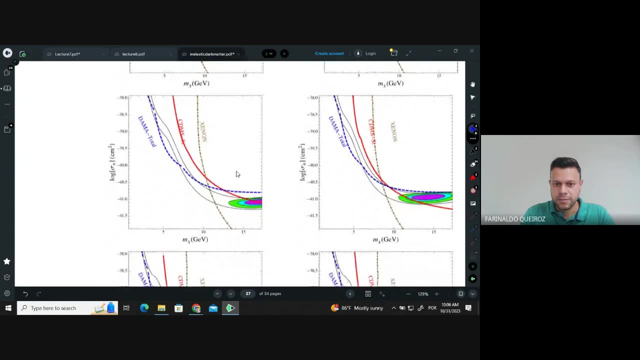 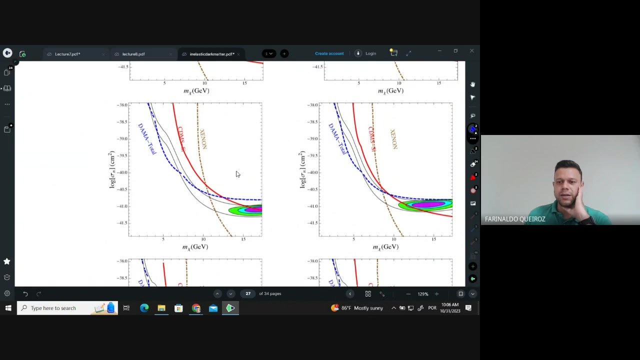 and then they go see here, now you have a whole region, which is okay, and then there it goes, many masses, and so on. now, for instance, this one is more clear because the scattering cross section friends in this case. okay, it's clear. so look at this. so this is the scattering cross section, where everything above the scattering 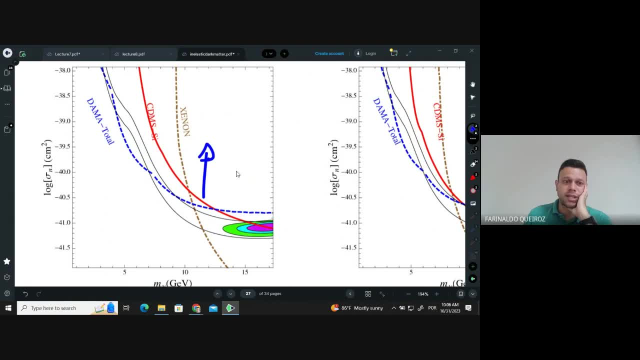 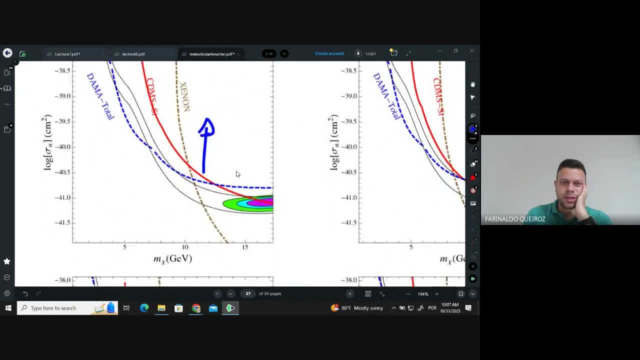 cross section is excluded, right, so you cannot have you know any event above. so now they are picking the mass and say, look, if you want to explain dharma and cogent, let's say you have to be within this best fit region. in this case, so far there is no inelastic dark matter. so i see, let me see. 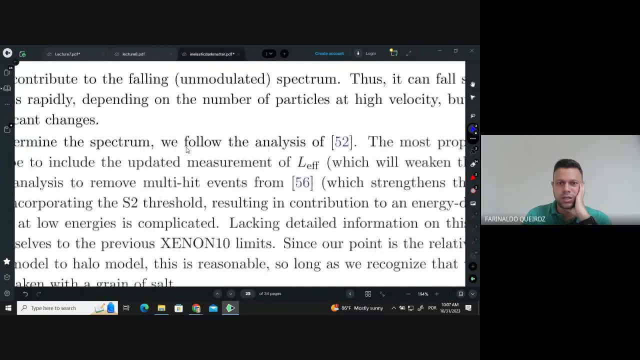 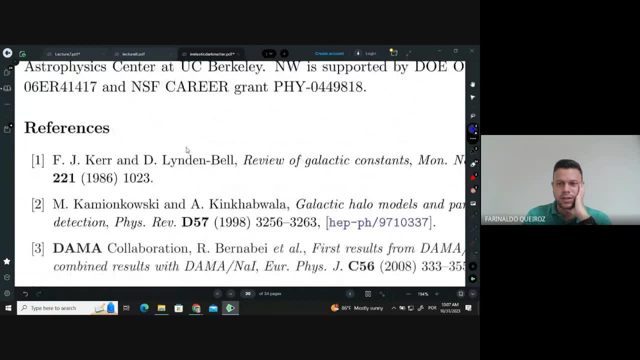 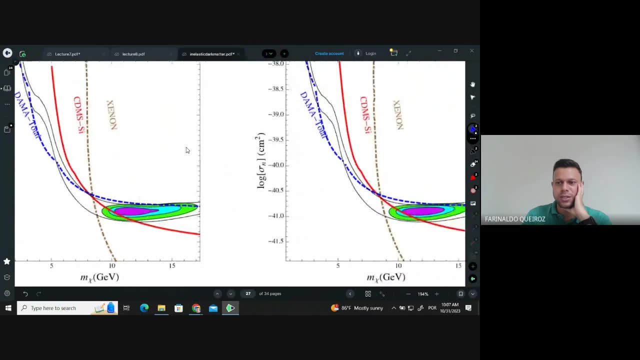 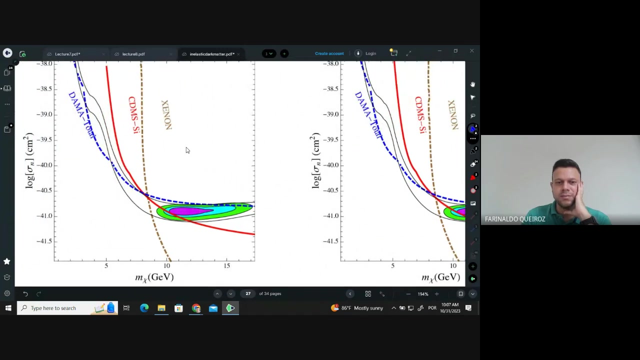 no, they just take a v velocity and so on. let me see if there is one. yeah, it's not there. anyway, i think the message was clear. it's just they want to tune the mass difference to make sure that the xenon signal, the dharma signal, still survives the xenon limit. and there is another discussion which i mentioned to you. 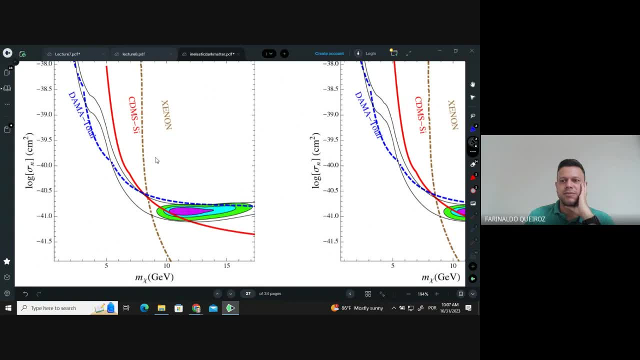 i think two lectures ago- which is, they take this limit from xenon and move to the right. so they- he appears right here- to survive some region there. based on on what argument? the fact that xenon did not know really well the quenching factor, so they overestimated the quenching factor. but this has been driven the community for. 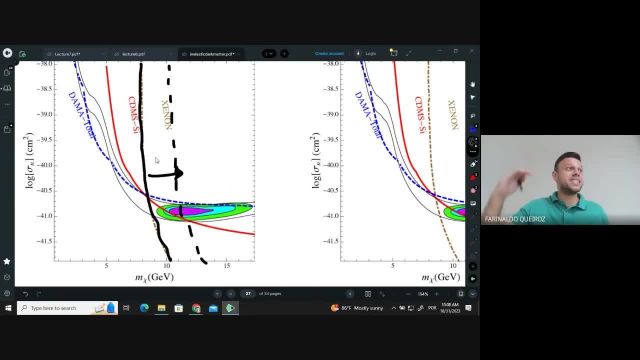 two, three years. but as xenon improved sensitivity says: look man, you can come up with quenching factor. tune the velocity in the last dark matter, i don't care, it will be excluded anyways. so the message to conclude, the direct detection part is: we observed cogent was very important. 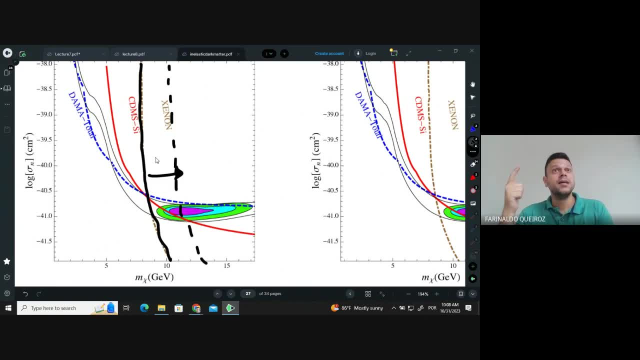 provide us a very important lesson. and dhama did see a signal from dark matter. the significance: well, did see a new nuclear recoil signal doesn't have to be from dark matter and the significance is over nine sigma. so nine sigma confidence level observed, a nine signal confidence level signal. and the signal they observed was: 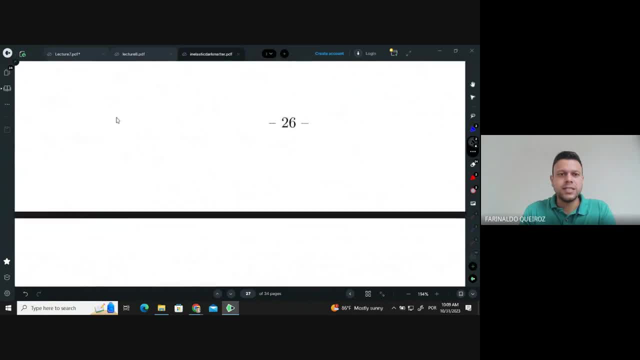 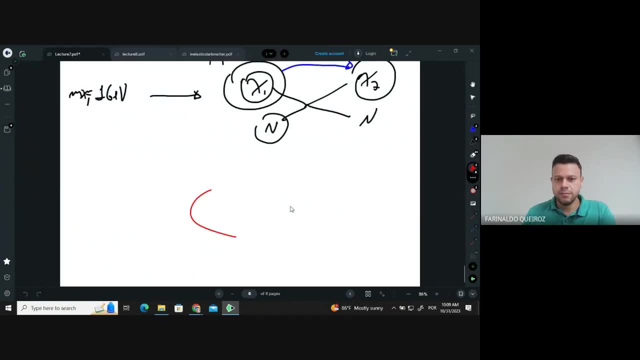 modulating time. why this has anything to do with dark matter. well, we are at the Sun. the Sun is moving in our galaxy moving. however, the earth is also translating right. so at some point, the velocity of the earth goes in the same direction of the Sun. sometimes this: 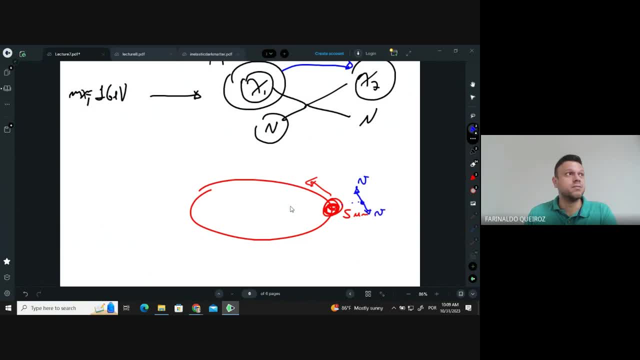 is going, moving in the opposite direction of the Sun. so it means this half of the year the earth is moving towards the Sun in the same direction of the Sun. the other half is moving the opposite direction. okay, so it means is there is a modulation signal? I mean remember, remember that the rate depends on 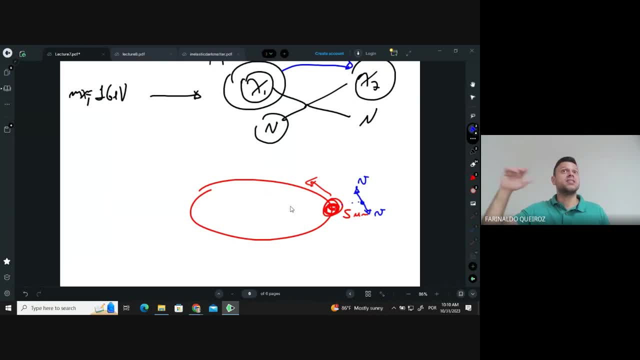 the f of V. so f of V is actually that is a, is a velocity, is a vector velocity, not just the module. so at some point this velocity goes in the same direction. they sum up, and the some half of the year they go in the opposite directions. okay, so you have. 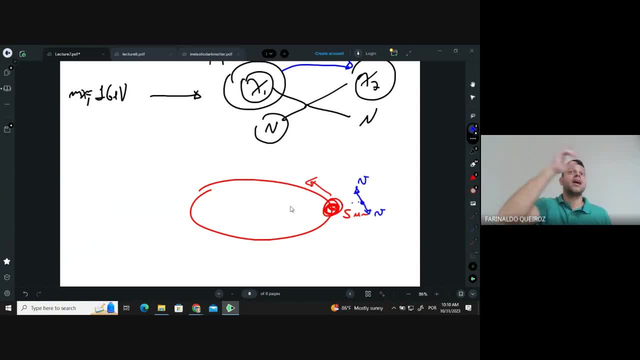 a summer and winter, different velocities, so you have a different flux or rates of nuclear recoils depending on the the season of the year. and this has been measured with: from Dhamma with a new. and this has been measured with: from Dhamma with a new. 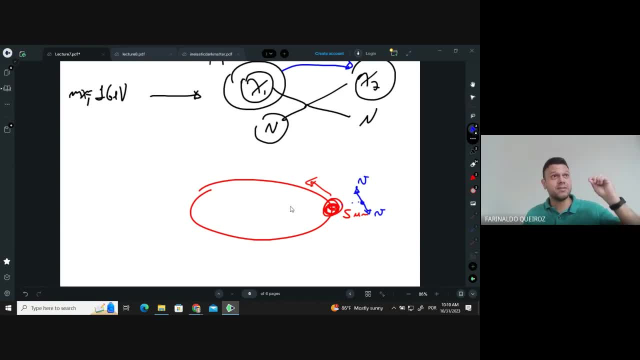 and this has been measured with from Dhamma, with a new measure, with from Dhamma, with a 90 confidence, nine Sigma confidence level. and that has been making the community crazy is: how can you see a nine Sigma signal and is modulating? there is no well-known background physics that will modulate in time, none. 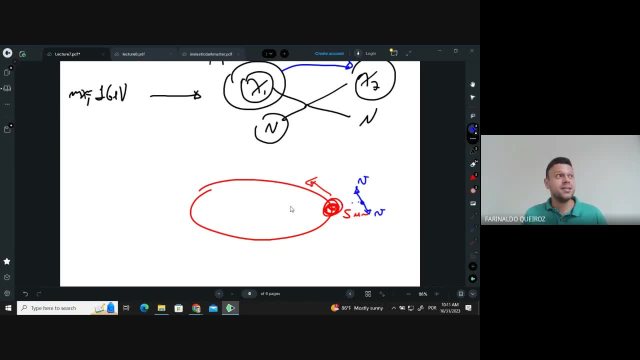 and then people realize that Neons from the Sun, they do not modulate in time. but they do not modulate in time with the same season. summer and winter modulation phase is different. the Sun cycle has a different cycle from the Earth's translating period. it's not the same face we have in ape, we have in. they have in the summer and winter. 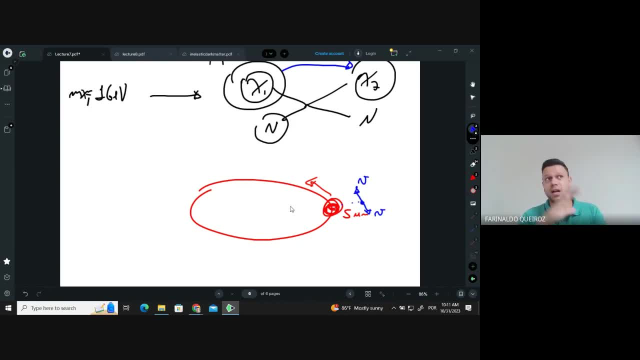 and the one from the mules from the Sun. cosmic ray mules from the Sun are different. one, the second test, they they didn't realize what it was. they built a different detectors, direct detections, called cosign. there were others to test using the same materials as Dhamma, made of sodium and iodine. this one 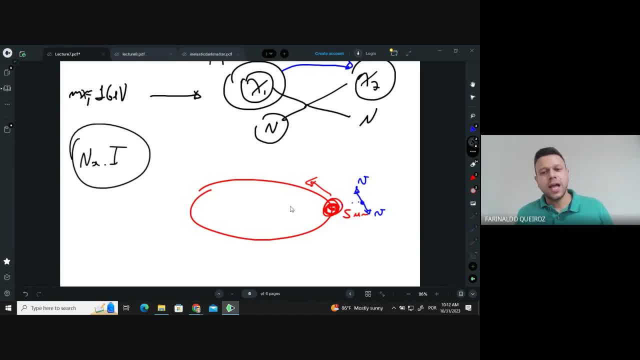 sodium and iodine, To test if it could also see a signal, to see a modulation in the number of events. They did not see a modulation in the number of events. And then people say, okay, maybe it's the location where Dhamma is, because Dhamma is. 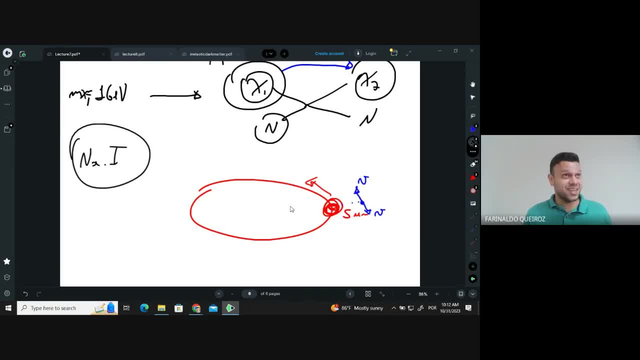 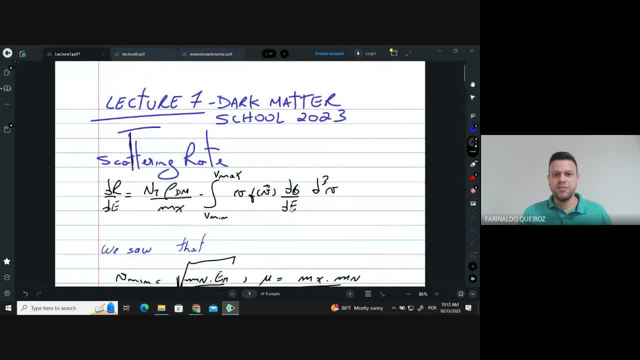 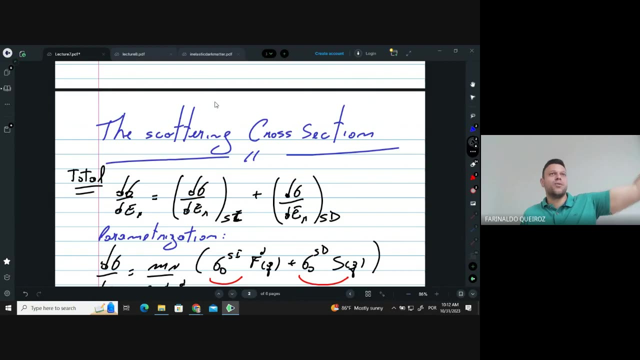 in Gran Sasso, But Xenon is also in Gran Sasso, If you remember the picture. they're basically one close to the other. Let's see if it's here. Ah, it's in the sixth lecture And the same lab. I mean a few walls away. 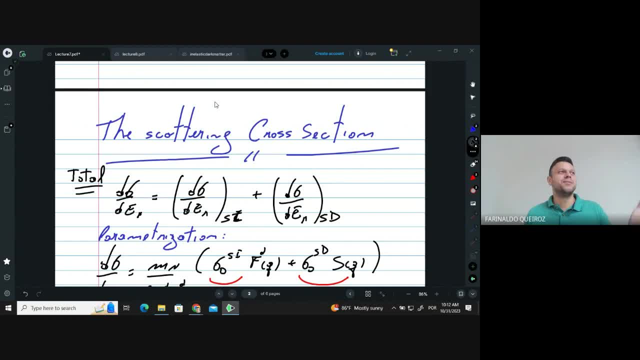 So it could not be the location. Maybe, I know, Maybe some stream of dark matter is hidden in Gran Sasso laboratory, And then what people realize- that's the most accepted answer to the modulation of signals observed at Dhamma- is that the electronics they have for some reason is leaking into. 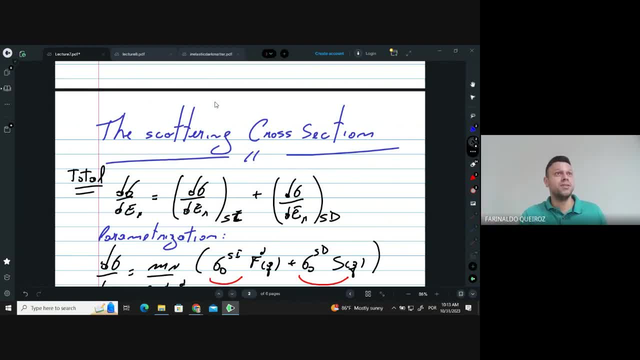 their detection. So it's not a single phase detector and producing a modulation. And, weird as that is, there are some nuclear materials which do modulate their decays. That was not known. They just realized this And for some reason, Dhamma is not a dual phase detector. 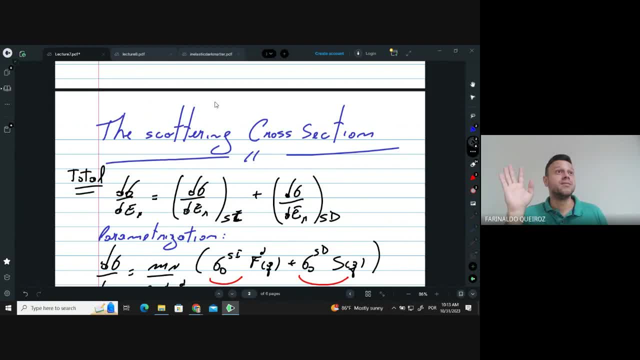 It's not even a single phase. Dhamma just counts the number of events And that's it. They have a tank of sodium iodide and detects the number of nuclear records and just counts, And they do it. They count the total number of events and say which ones are modulating time. 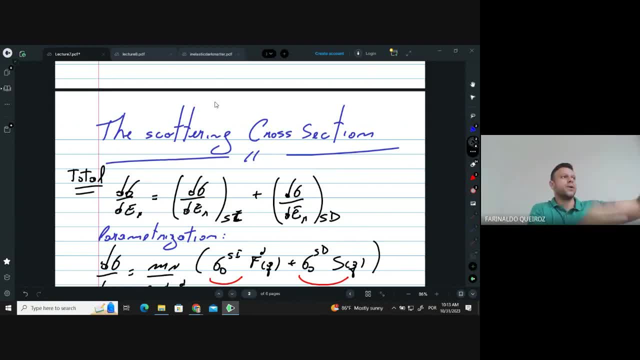 These ones? They are not. The others are not modulating, So throw them away. So they do not distinguish whether the event was coming from dark matter, from nuclear beta decay, whatever. They just sum them up And people are placing doubts. 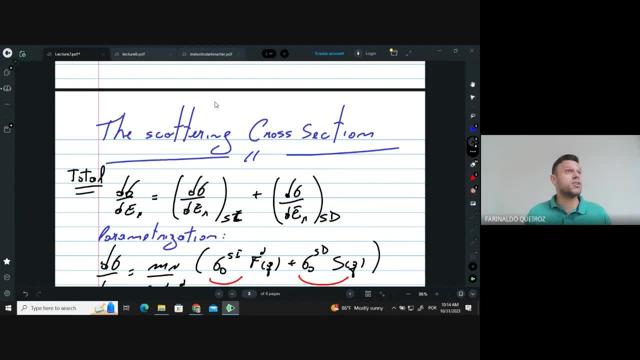 Hey, OK, So since this is so important for the community, could you show us your data, Your raw data? No, we won't, So let me test your hypothesis to see. if you didn't, No, you won't. And then, as they are not publicly showing their data to the community, then their results. 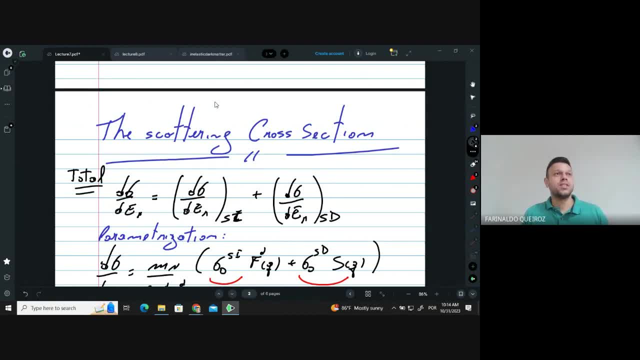 were not taken so seriously, Because if you're confident about your result, this experimental result, you should be able to make your data public. OK, Because that was like, remember, if they did observe dark matter, they get a Nobel Prize. 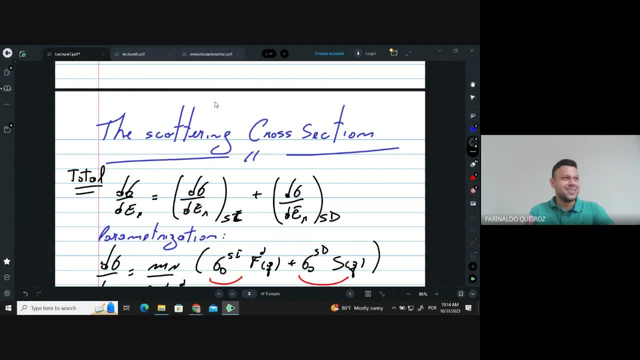 Is the Nobel Prize worth attitude. If they show it's there the Nobel Prize. So why didn't you want to show it? And they haven't shown it ever, And they have been observing a modulation signal since 2000.. I believe. 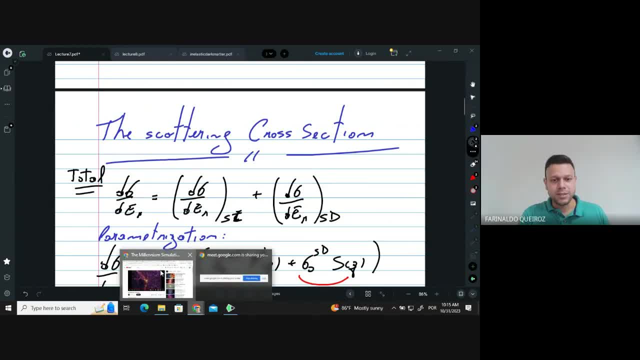 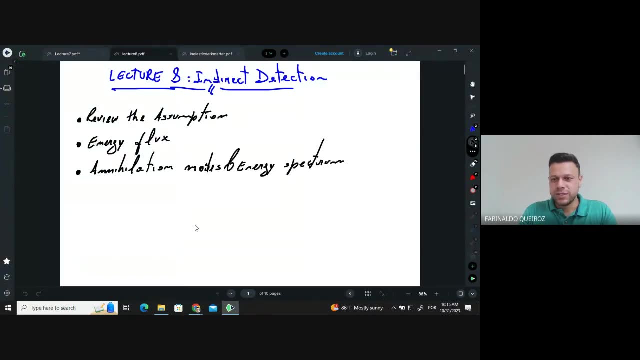 OK, So let me just up to this point. So let me just, man, I end up just talking about drug detection. So I just wanted the next 15 minutes just to start warming up for drug dark matter detection And I have to leave soon enough. 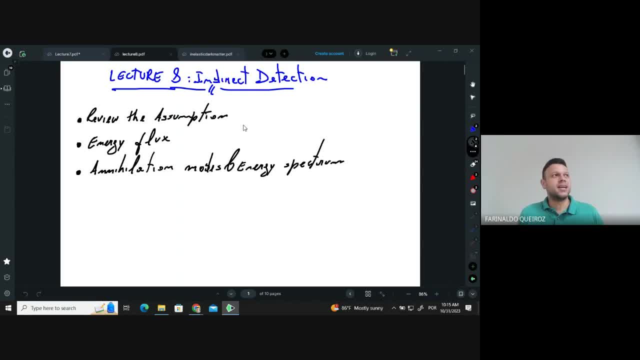 Whew, And first let me ask: is there any question? so far, No, Someone there Back there, So our girls are back, So I'm not going to ask the other girls. We have other girls there, So anyone. 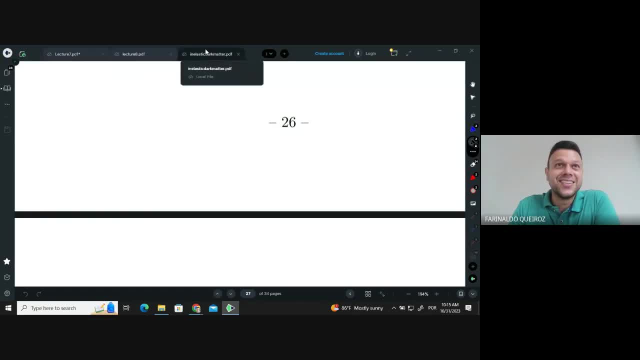 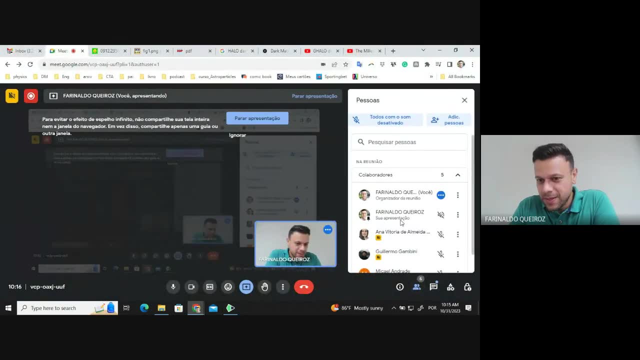 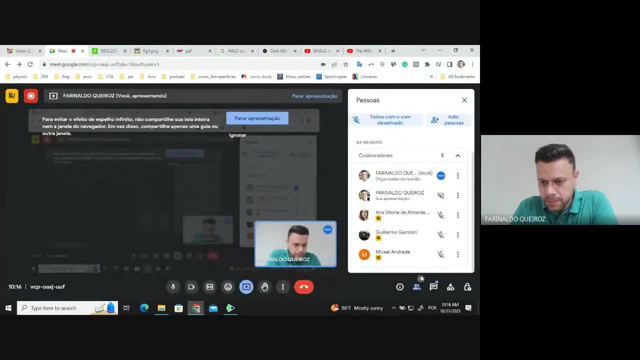 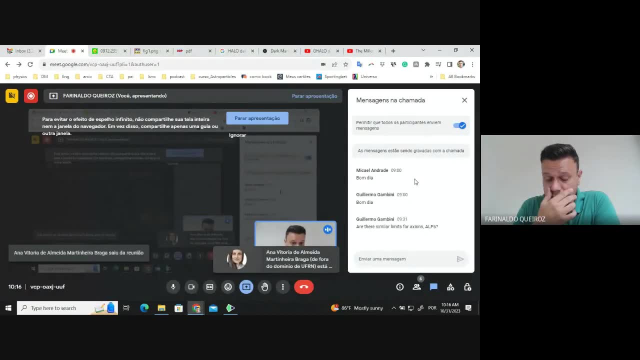 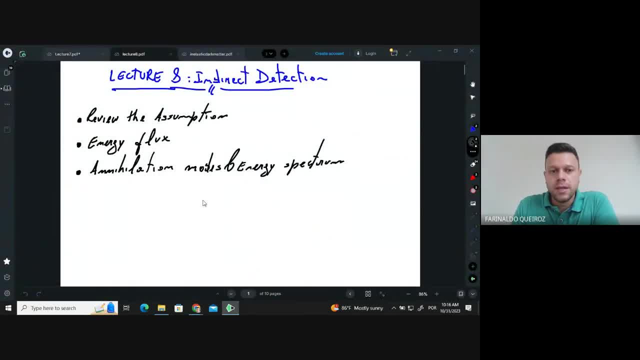 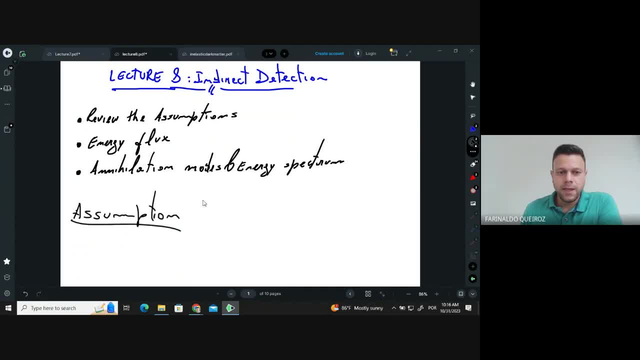 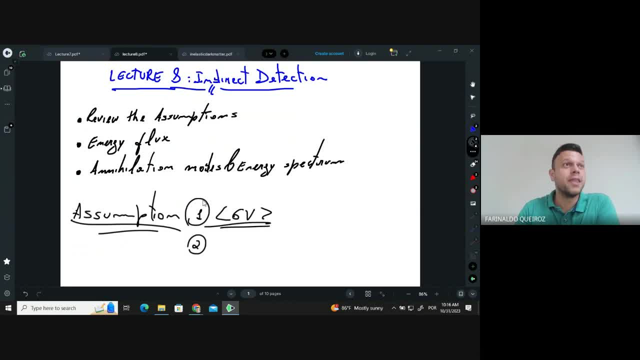 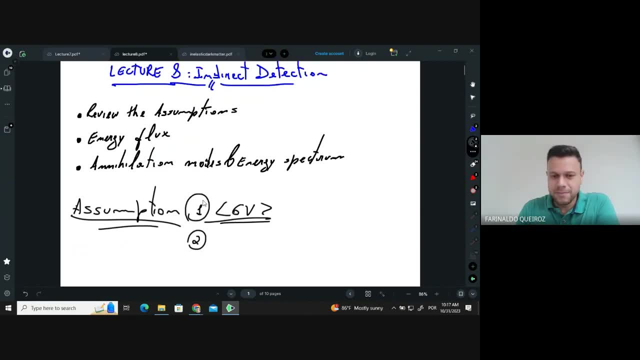 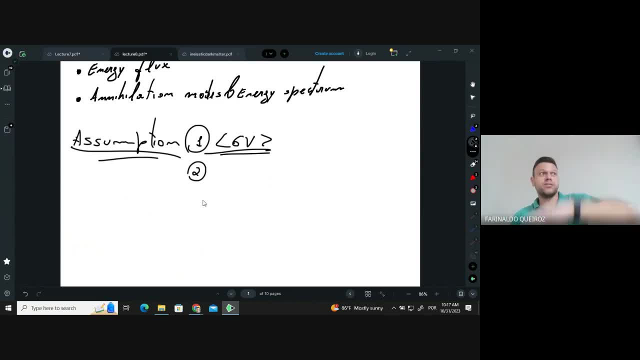 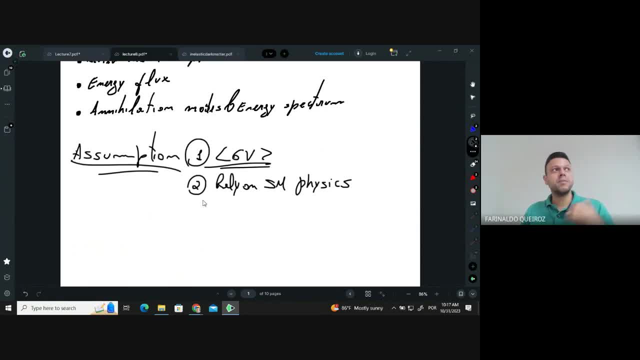 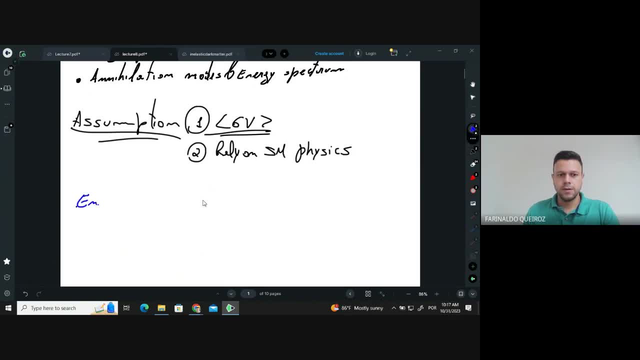 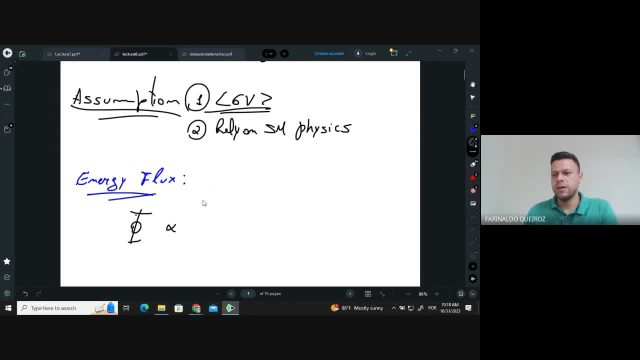 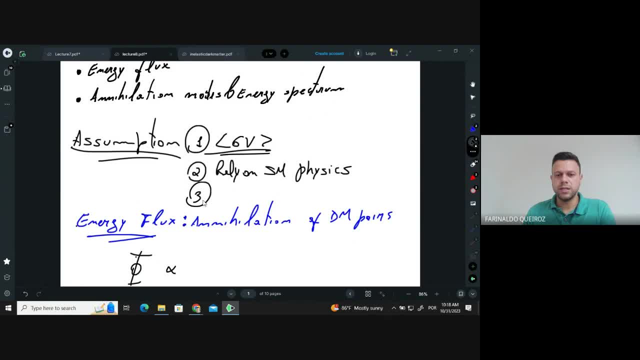 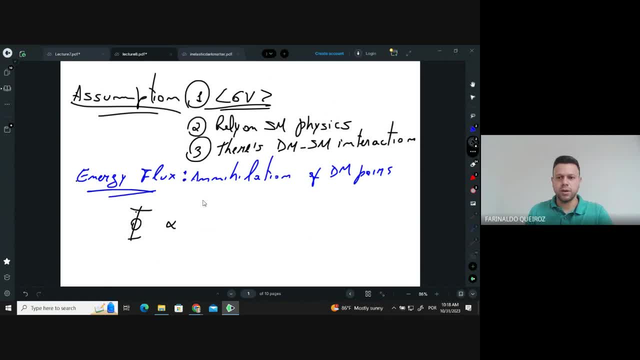 Okay, so I'm assuming that dark matter does interact with external matter particles. Do you guys know here in the room why is a reasonable assumption that I should say, okay, there could be dark matter interaction with external matter fragments. Why is this a reasonable assumption? 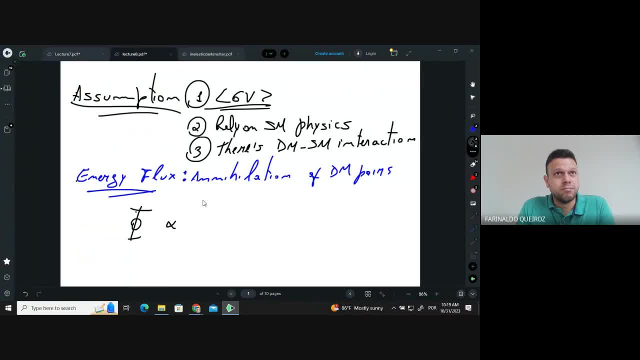 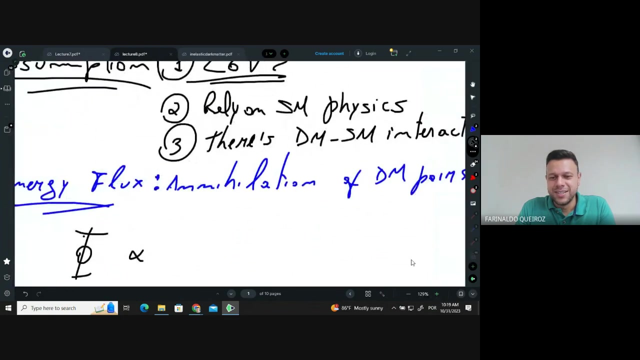 Yeah, it's impossible. okay, It's from detection, but why is a reasonable, theoretical assumption? Why is this a theoretical, reasonable assumption? Yeah, exactly So he answered. So the reason is: we started the whole thing discussing the relic density. 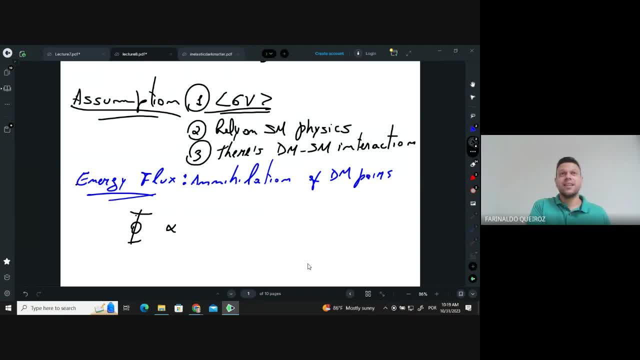 And the way to compute the relic density was assuming that dark matter could interact with external matter particles. right, And they were in thermocleidomere, Even if they were not in thermocleidomere, but they would interact with external matter particles. 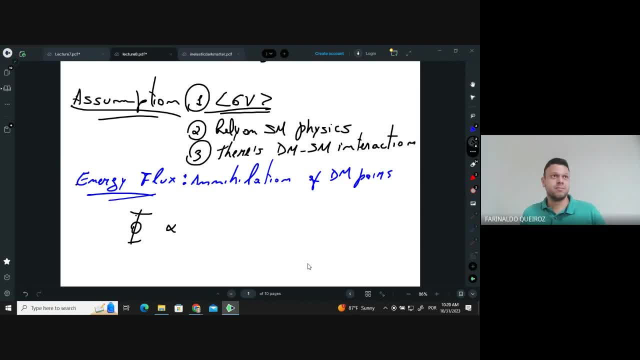 And that would determine the freeze out and so on. So if you assume that if dark matter particles were in thermocleidomere, then it's a consequence of that that dark matter might indeed interact with external matter particles today At a different rate, but it's still interactive. 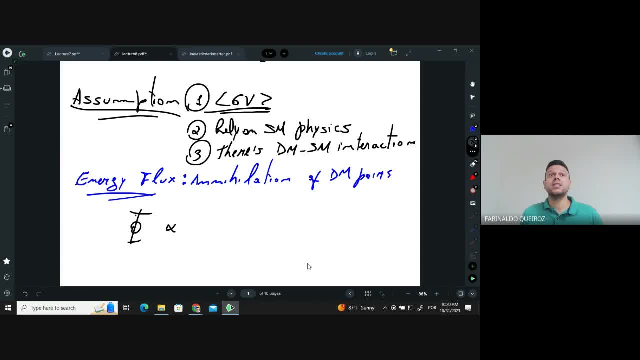 Okay, because we computed the relic density comparing the sigma V- the rate, with the expansion rate. The expansion rate is cosmology, The rate is the annihilation of two dark matter particles into external matter particles. So if that happened in the early universe, 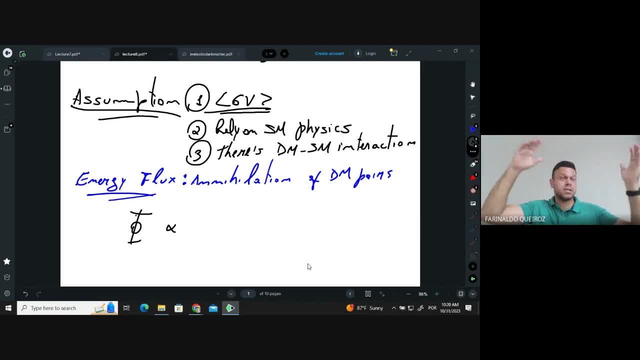 it could happen today at different temperatures, but the cross-section would still be there. Okay, not necessarily be the same, but the interaction will still be there. Makes sense. So if there was not thermocleidomere, no thermocleidomere. 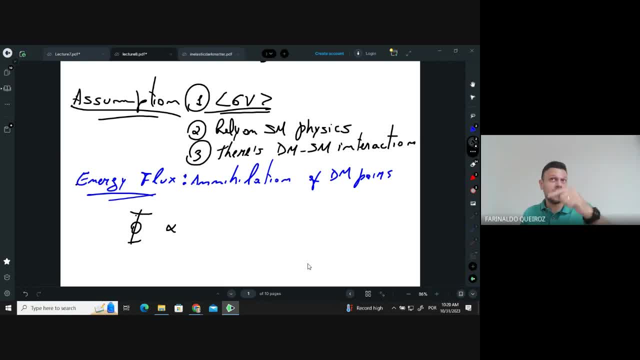 then it's tricky to say, okay, there is annihilation today, but well, if it was not in thermocleidomere back then means that the annihilation of external matter particles, if existed, was really really small in order to go outside of equilibrium. 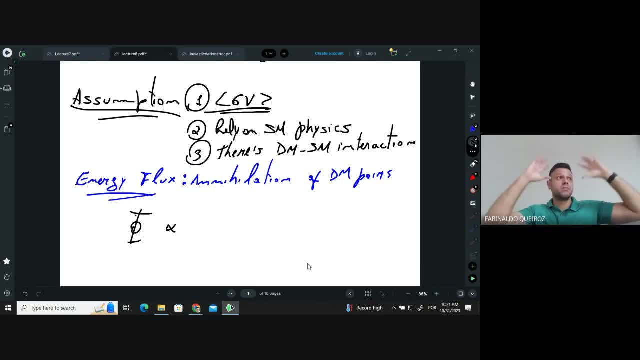 So dark matter particles were never in equilibrium with external matter particles means that the interaction between two dark matter particles and external matter were really, really, really small, It would not reach equilibrium. So this way it would go. this would not go back for it. 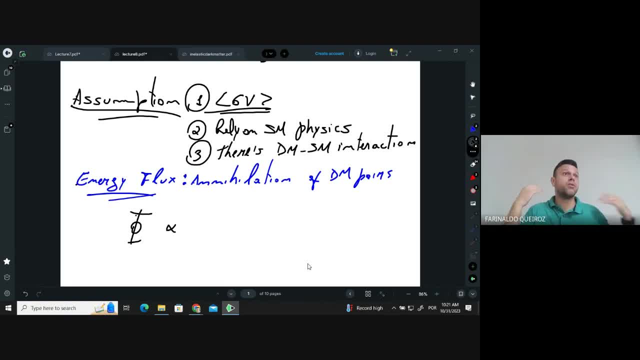 It's really small, So, but if they were in thermocleidomere, then it's a sizable interaction. It's a sizable interaction between kai-kai, fermi-fermi, fermi-fermi, kai-kai. Well, if it happened in the early universe, which dictated the freeze out, so why not happening today? at different rates might by happen today, Okay, Especially where you have a large concentration of dark matter, let's say in the center of galaxies, in dwarf galaxies. where you have a large concentration of dark matter particles, then you increase the chances of one finding each other and annihilating. But please be careful. The overall amount of dark matter is not really changing much because these interactions are really weird, So you have abundance of dark matter. 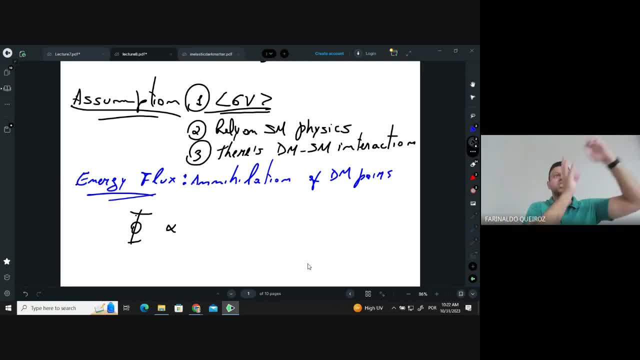 which they froze out. Remember, the freeze out means that they stopped annihilating to some amount of particle fermions and the expansion rate equaled the annihilation rate and they froze out. There was no kai-kai fermi-fermi anymore. 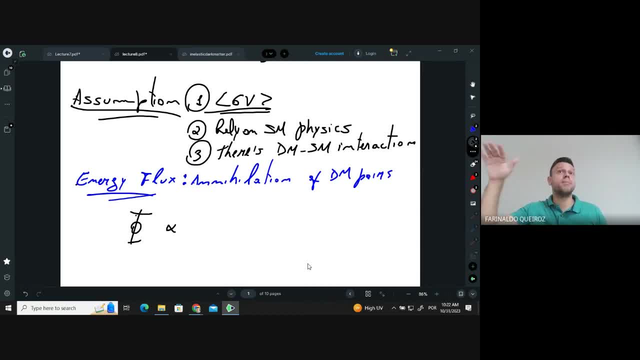 That's what the freeze out means. right, And we have a leftover, abundance of dark matter particles. But today, in large, in places in the universe where the concentration is really large, there might be, despite where, a chance of those two dark matter particles finding each other and producing signals. Okay, And these are in local, in some places, like here, like in center of galaxies and dwarf galaxies, where the density is really large, and then you include neutron stars and so on in specific astrophysical objects, But it will not change the overall of the whole universe. 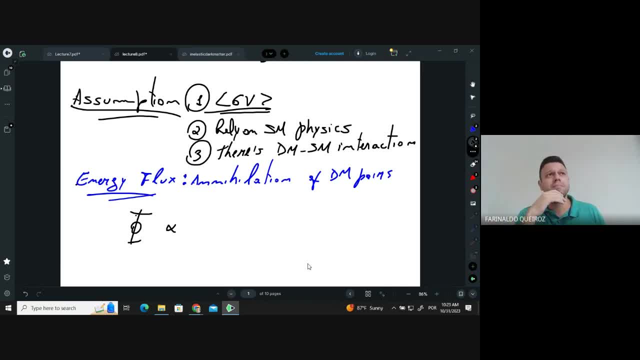 Abundance of dark matter is always not meaningful effect for the overall budget of dark matter, Okay, But it still can produce a signal that I can detect. Okay, So the flux, if I have two dark matter particles have n kai and n kai. 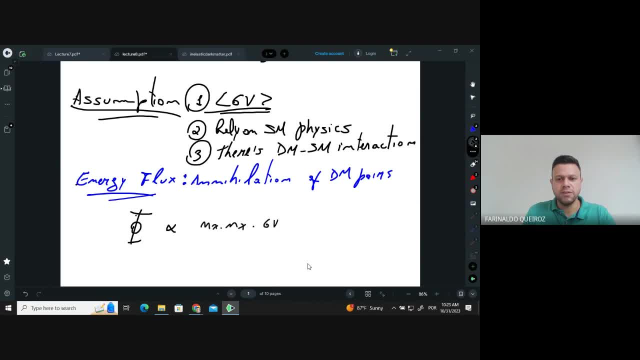 it should depend on how strongly they are interacting. sigma v, not thermal. and should depend on on what else from this formula only look at this for non-relativistic particles, non-relativistic particles, non-relativistic particles- Again, I'm assuming to be non-relativistic. 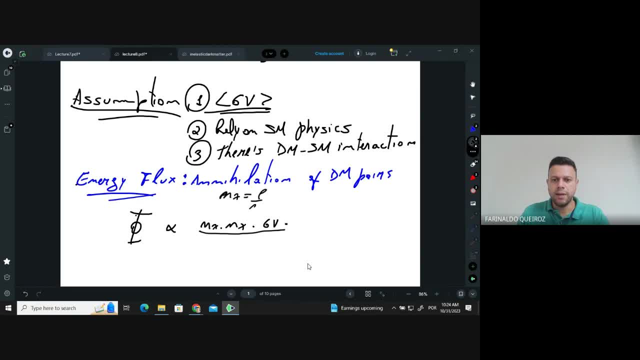 Then n is equal to rho over n. Then I'm going to erase these two m's. I'm going to put m squared here and rho squared there. Okay Fine, But now what I'm going to do is I have kai kai producing from the first. 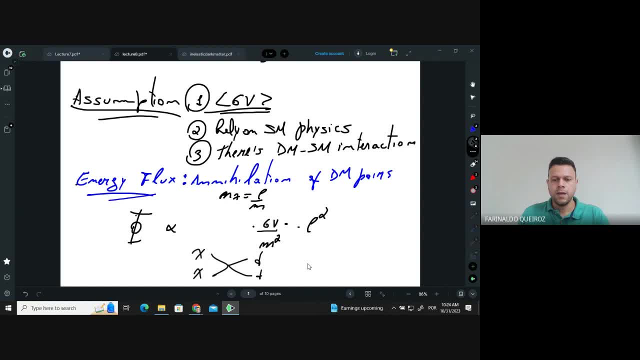 I'm going to put kai kai producing from the first. I'm going to put kai kai producing from the first, kai kai producing from the first, If I'm interested in the number of gamma rays produced. so five gamma. 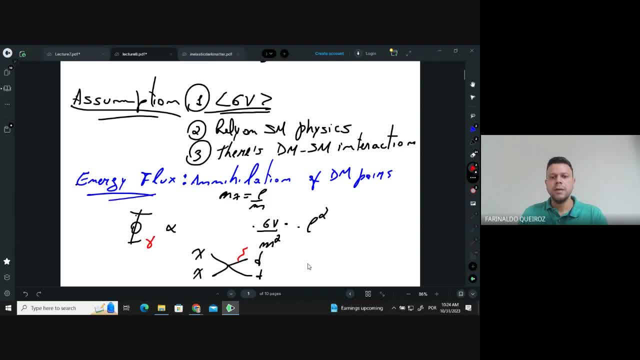 I want to know how many gammas are produced per annihilation. So if I produce one gamma, I have one number of gamma rays. If I produce two gammas, so even if I had one annihilation, so even if I had one annihilation, 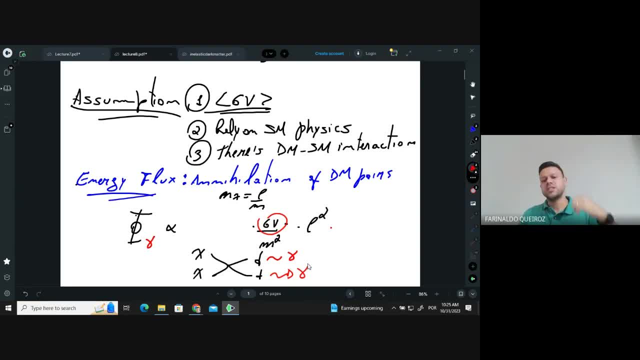 I produce two gammas, I produce one annihilation and I produce three gammas. I produce one annihilation and I produce three gammas. so I should account for the number of gammas produced. Okay, But the number of photons produced does depend on the energy of the incoming particle. 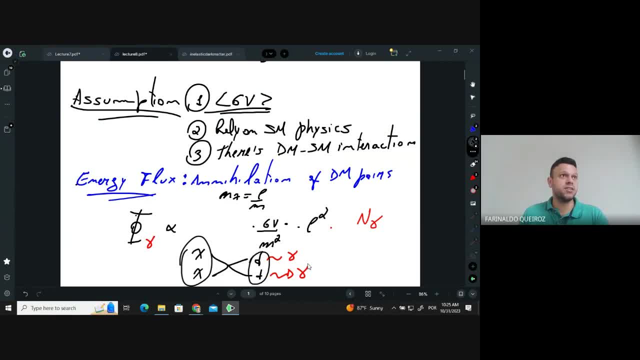 or in other words, the energy of those particles in the final state, which is controlled by the initial energy. So this number of photons and this number of gamma rays, and these photons have a continuous distribution Because if you have one TeV energy, 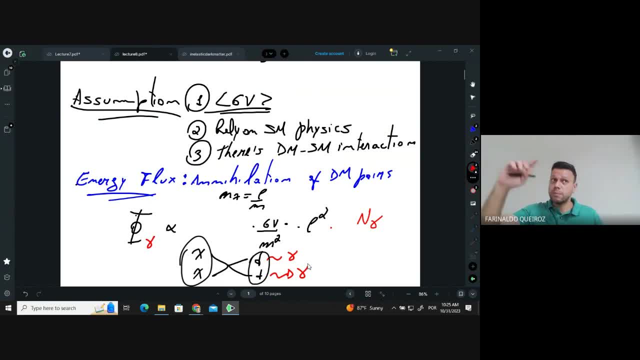 and you produce E plus and minus one TeV, you're going to produce one amount of photons. If you have a 10 TeV energy put into E plus and minus, you're going to produce a different amount of photons because the accelerated, larger energy will produce more photons. 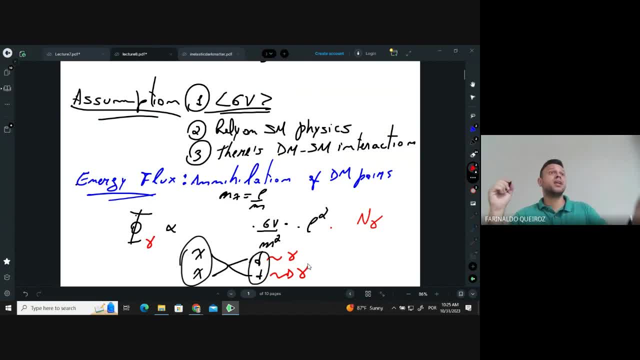 The amount of radiation you get depends on the acceleration you have. In other words, in the initial part you have 10 TeV, In other words, in the initial energy you have. So this number, the flux, is a function of energy. 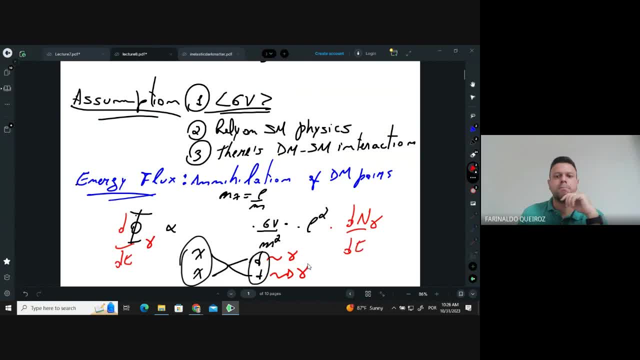 as well as the number of photons produced per annihilation. Okay, Moreover, as my telescope, I'm probing a region of the sky and I want to make sure that the flux I'm observing from this region of the sky is consistent. 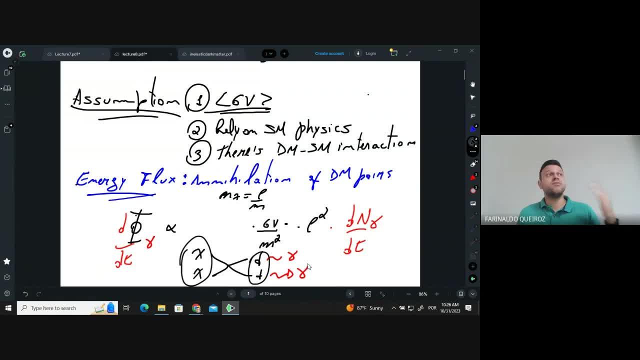 with the number of photons that Leticia observed with a different telescope observing the same region, but in a larger volume. So I normalized by the solid angle of the region I'm observing. Okay, So this means that you have a D gamma here? 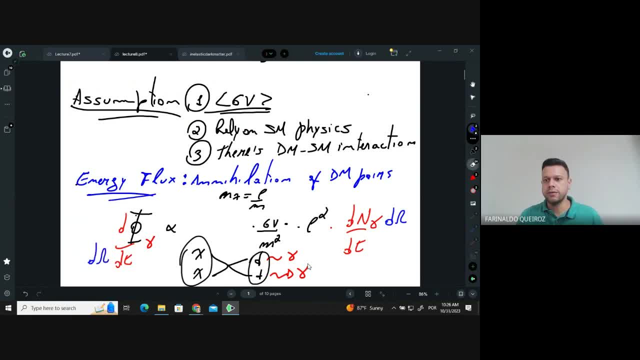 or you put a D solid angle there and then you put the solid angle there and the angle here, normalization, which is four pi squared. Okay, Four pi. So that's the formula for the energy flux, That's just the flux for dark matter, annihilation. 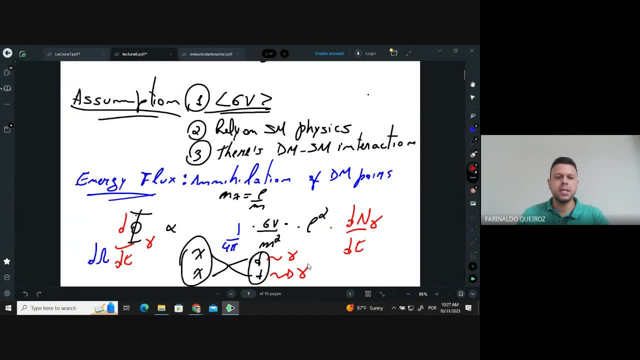 And the energy flux is simply: you take this formula and now rewrite more beautifully: d-flux, d-omega, DE. equal sigma V over m, chi, squared one over four pi, integral, rho, ds, dn, DE. And now what I did? I just did this. 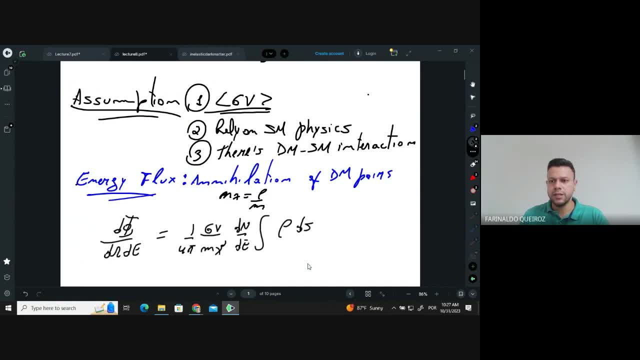 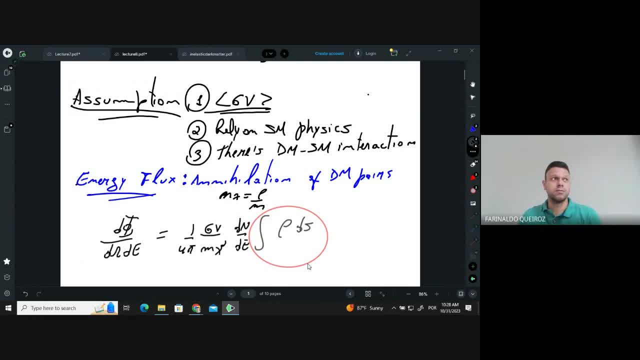 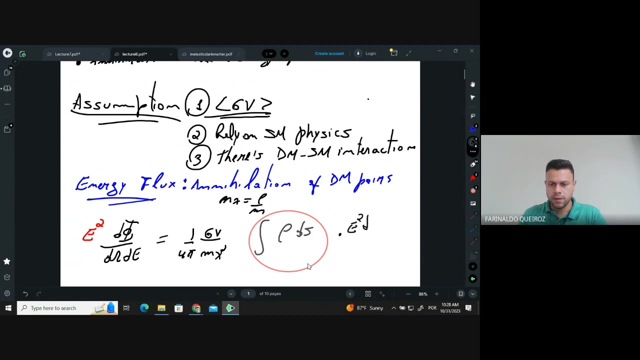 across between the distance between me and the source. and this thing here, when I multiply by e or e squared, is called energy flux. so I then multiply by e squared here, or I rewrite this thing here, let me erase, okay. so what I'm trying to concentrate the next lectures is to: 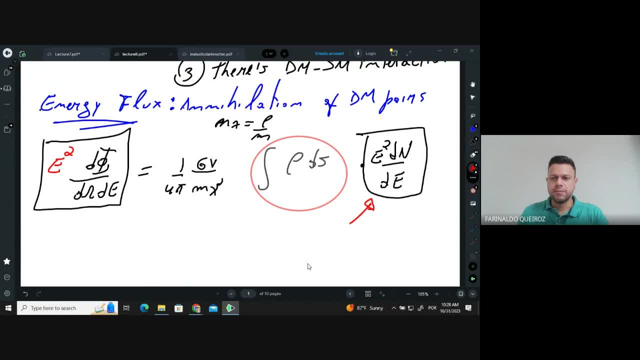 you derive this thing called energy spectrum. so this is from. I mean, I'm gonna write this: the energy spectrum comes from collider physics, this comes from astro, astronomy or astrophysics. okay, so this is from astrophysics, from, if you, for examplewhether, it was where. 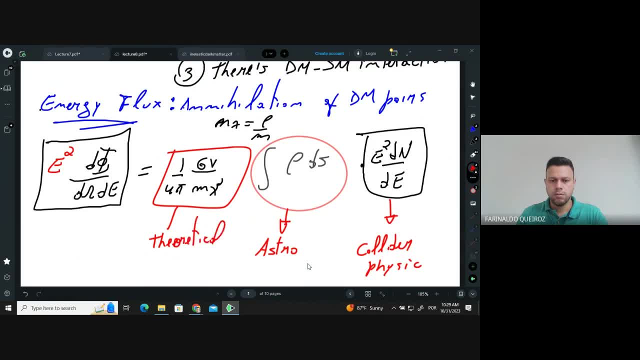 Speed is held or temperature is held, you can see radiation ascendance, calves 问. or this comes from from, let's say, your theoretical model in particle physics you I observed in terms of some dark matter model. I need to input from astronomy, astrophysics, collider physics in order to program all for a direct detection. I need an input from nuclear. 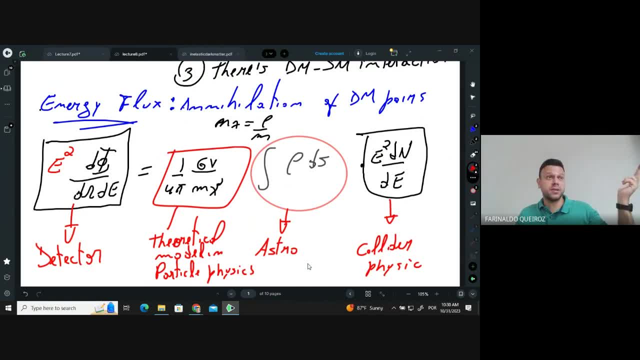 physics, astronomy and the detector measurement- so it is just these two detection methods- is showing to you that this search for dark matter requires most disciplinary science. just the right commodity building does not suffice, you, Dean. you do need input from different sources. okay, so as a dark matter physicist, you should not follow some weird trends and try to undermine different areas of. 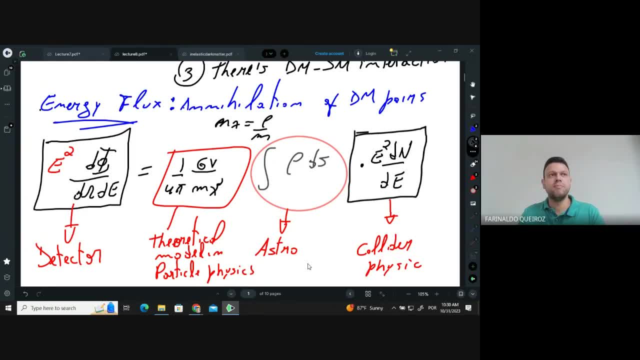 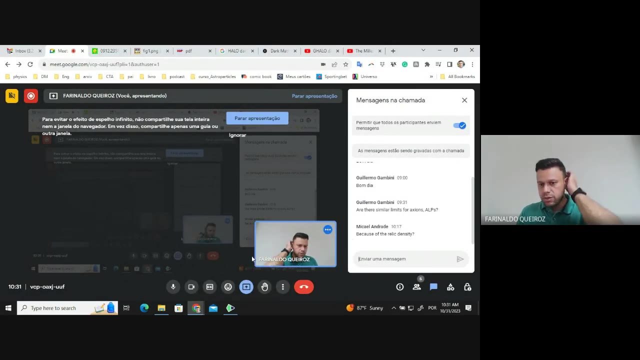 research, because sometimes, in order to solve big problems, you need independent input from other areas which are not necessarily yours. okay, they are also important. okay, and I think we finished for today. we don't have any more questions. Mikal asked for the relic. Mikal, could you repeat the? 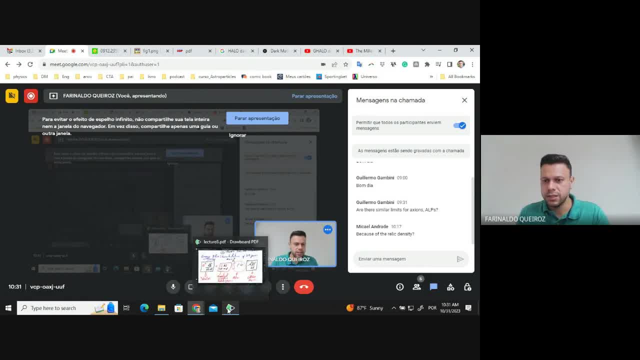 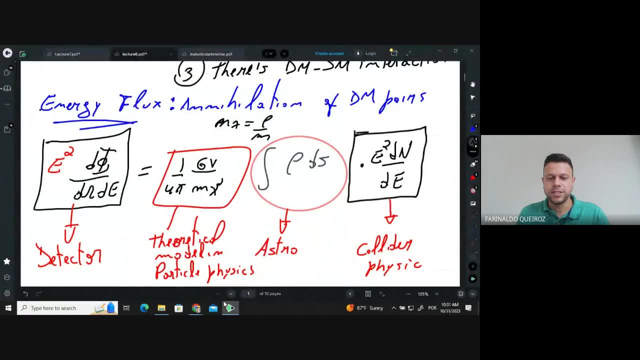 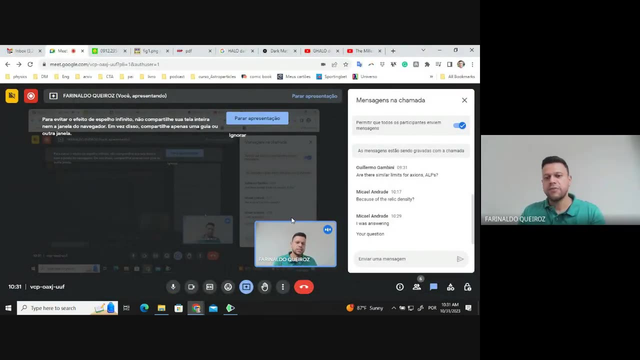 question, so I don't know in which point that happened. for the relic density: yeah, maybe he was. yeah, I was answering okay, yes, because of the relic density, perfect, okay. so if this has to do, for instance, with Gijemo, asked let's say, for actions, actions, uh, the relic density you can put. 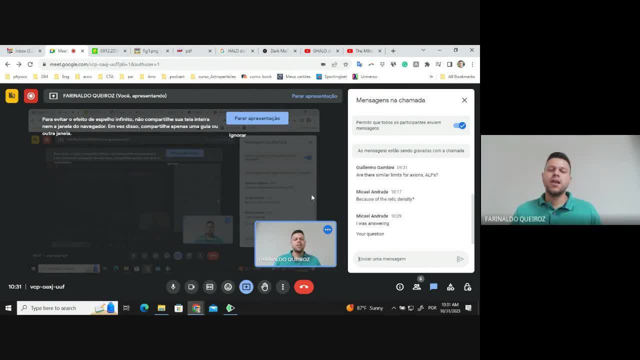 for actions has nothing to do with annihilation. therefore, it's not natural to expect any signal from gamma rays. annihilation of actions, annihilating, producing gamma rays- that's. that's. that's weird, actually the action. they do have a lifetime. they're not stable particles fully stable. they decay for. 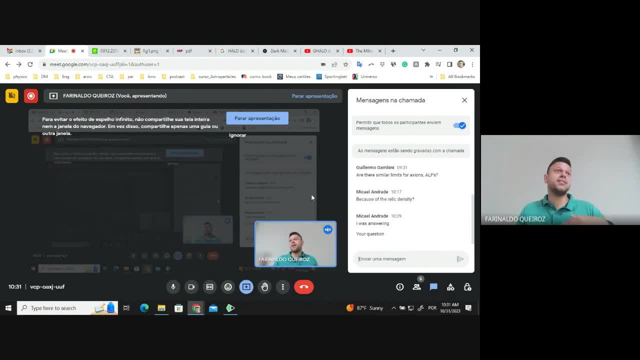 lifetime, much longer than the age of the universe. that's why we haven't seen them decaying. okay, so access could be dark matter. to me they're not so um, that's my personal taste, and they're not so compelling because you assume them to be unstable. so it's like to say you're putting. 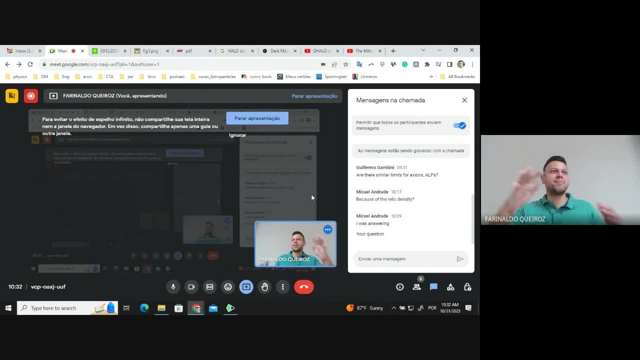 an end to the universe because you say they're unstable dark matter that stopped to exist. we are a. there is no Galaxy and we, we are gonna be killed. so it's just this, okay. Dark Made has to be stable, not cosmologically stable. it's just not natural to me, you know. so you, okay, you have a part which is long. 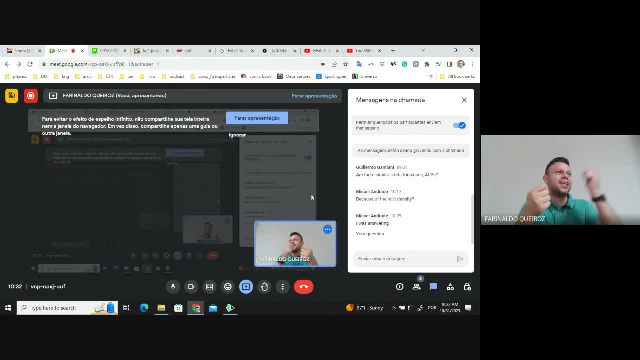 lived and it's dark matter and it's just tune it the Lifetime to be large enough. enough, because we didn't see any decay. so I just increased the lifetime. I said nobody's stable for us, but in you know, 100 million years from now it won't be stable. 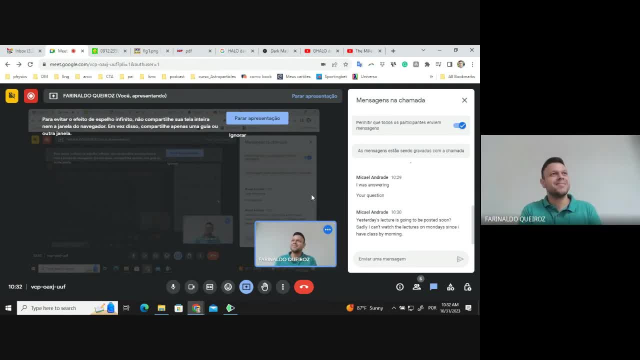 Everything will be doomed. OK, it's fine. It's consistent with data, It's OK. It's just not so natural to me. Axios is a different story. Axios are very, very well motivated, But Axios and Dark Matter to me is just my taste anyways. 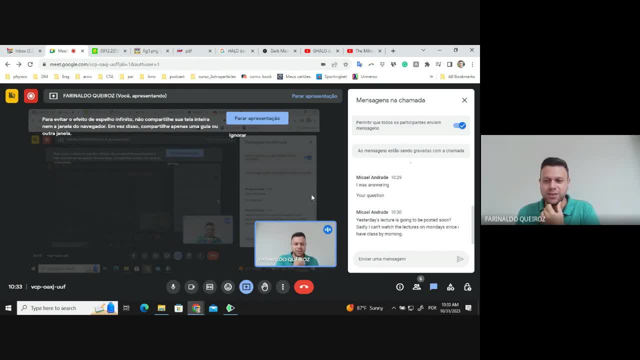 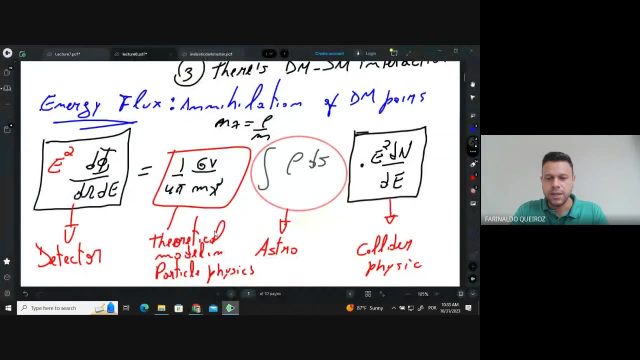 So yes, I'm going to post last lecture on YouTube. I just didn't post it yesterday because I had some other things to attend to, Sorry. So just to finish, as I was saying that we need input from other things And the Axios would not annihilate into something, 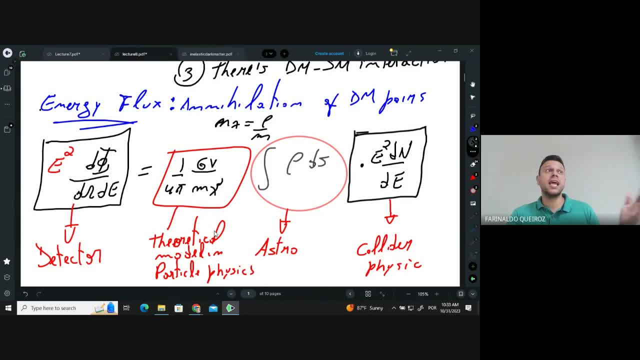 that I could see, But I could also observe the decay of Axios into something else. Then, instead of being this form of annihilation, what you do is you replace this sigma v over mass. You replace the sigma v over mass here and put the rate. 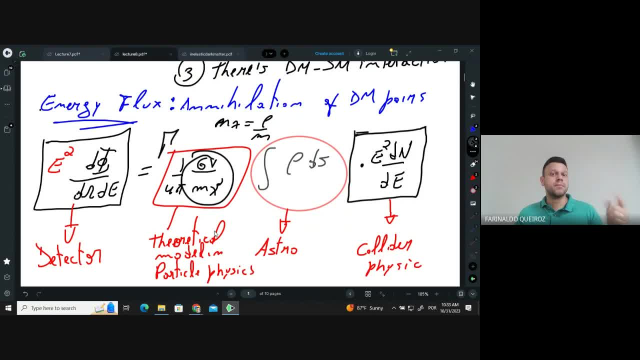 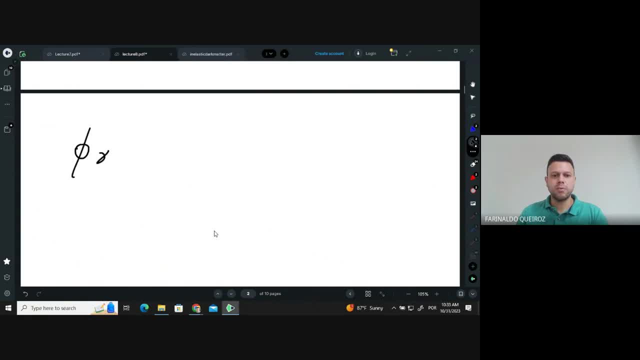 Instead of being m squared, it's just m, Because the flux- I started this formula discussing flux- should be proportional to number. densely squared right, I have two Dark Matter particles. I had two right by each other, But now I had just one, which was the decay. 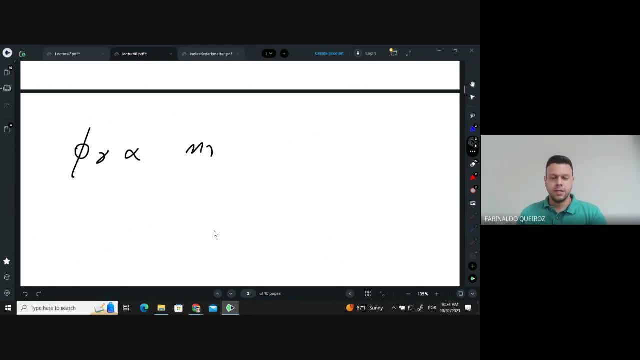 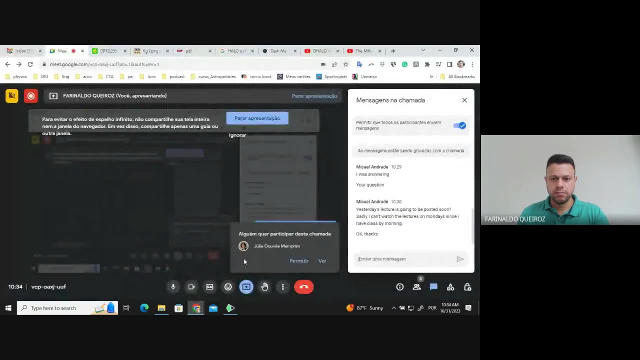 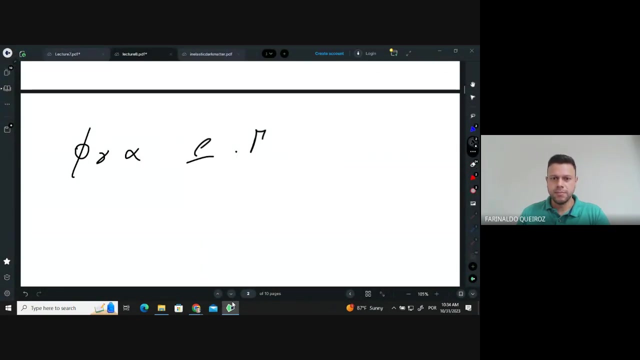 I just want decays, I just have n chi. So then, while someone is entering, now, n chi And I had the interaction rate, So n chi is rho over m, So I'm going to replace this with rho over m, OK, 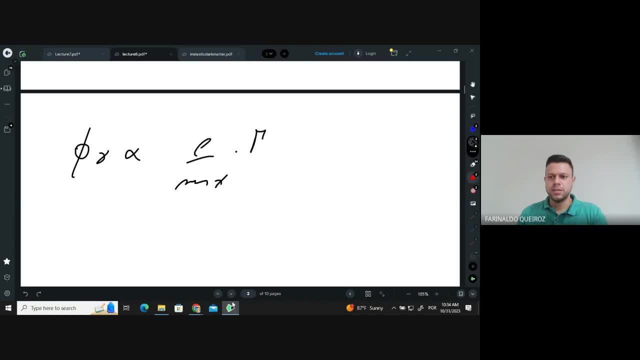 And what is the rate Rate is 1 over the lifetime. So then I replace this with 1 over the lifetime. OK, And my DNDE is still here And that's a flux, So the flux for decay would be equal 1. 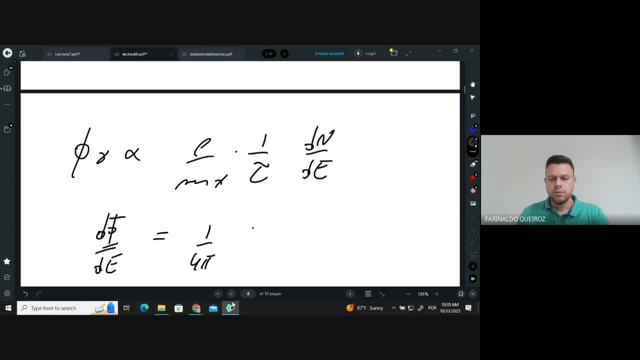 over 4 pi solid angle, The integration, rho, DNDE and 1 over the lifetime. So the longer it remains for the Excellent Slides, OK, then I replace this with 1 over the lifetime. look, the largest the lifetime the dark metal particle, the smaller is the flux. 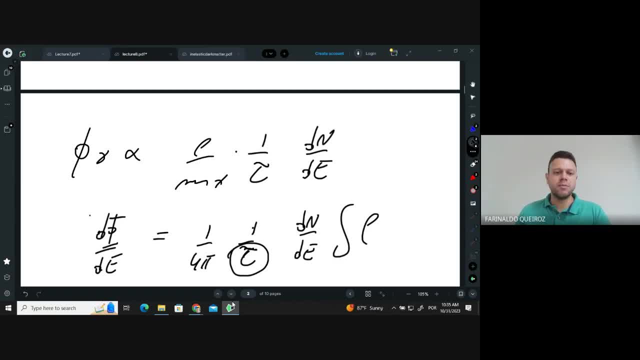 so if i do observe a flux of gamma rays, let's say 10, then i have to place a limit on how large tau should be to produce a flux which is smaller than 10, because you see, as i increase tau the number is smaller than 10. right? so i can do have a document particle that produces eight. 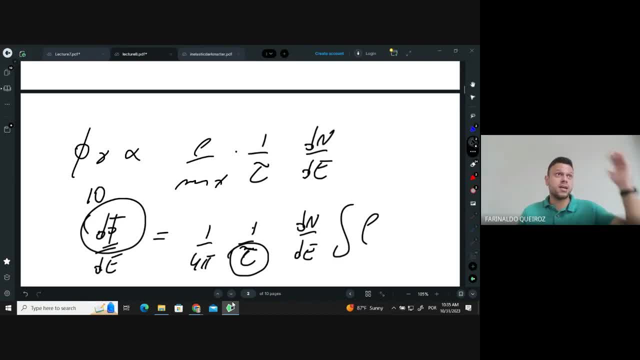 events, but not larger than 10, because i observed 10 and most maybe i can say no. seven events came from dark matter and all the other three events came from whole stars. whatever it's a master physical source, okay, so i have to just impose a lot the place, a constraint on the dark metal lifetime.